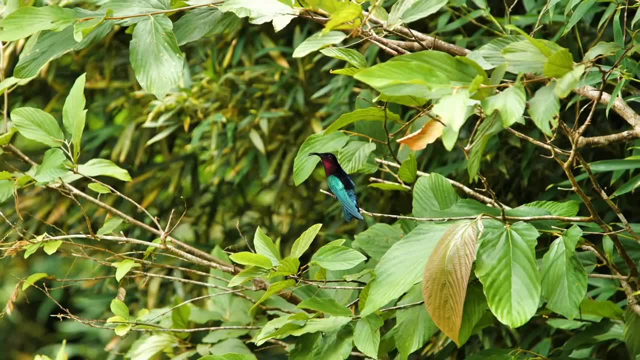 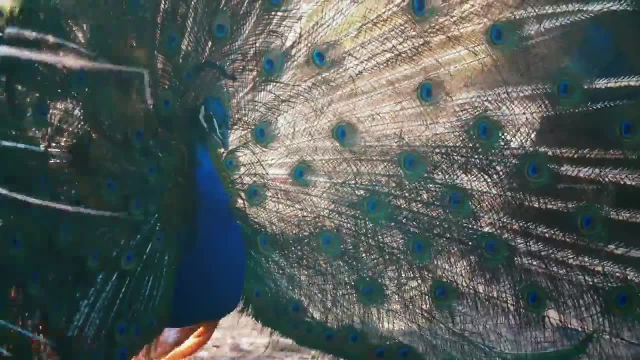 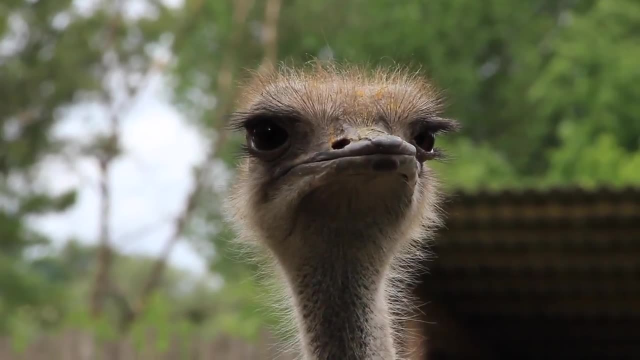 Slater had made a name for himself in the realms of ornithology, proposing a new way to divide the globe Based on the distributions of birds. But, as with many of his fellow scholars of the Victorian age, his curiosity about the natural world could not be contained. 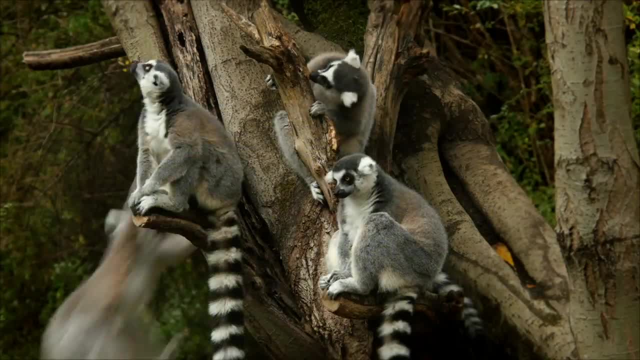 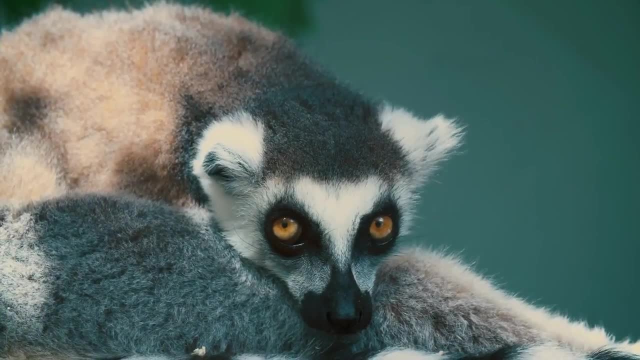 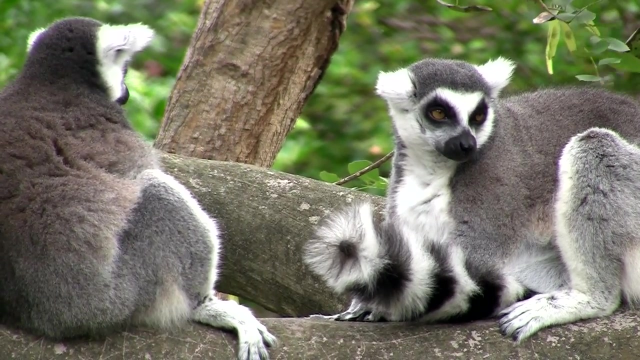 And now he turned his attentions to the mammals of Madagascar. He pored over the specimens, returned to him probing and classifying with intense fervour And, slowly and surely, a seed of an idea grew inside his mind. A seed of an idea grew inside his mind. 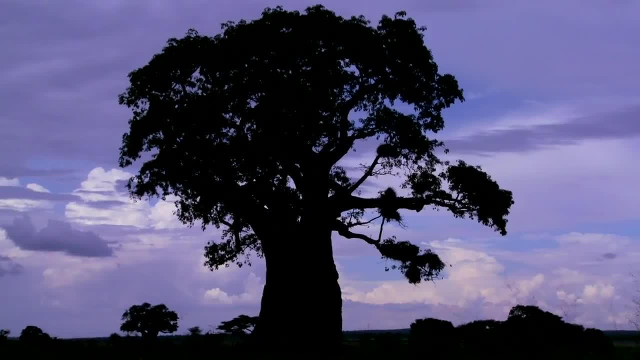 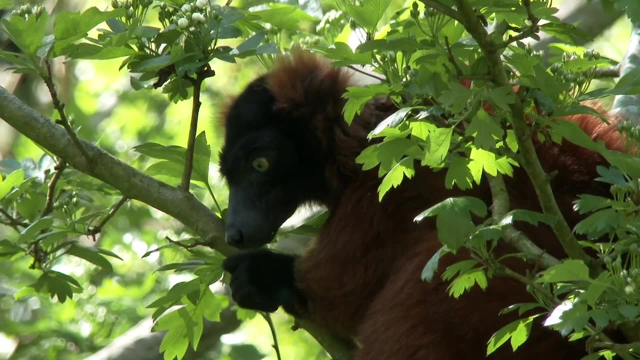 And slowly and surely, a seed of an idea grew inside his mind. And slowly and surely, a seed of an idea grew inside his mind. And slowly and surely a seed of an idea grew inside his mind. There was indeed a staggering bounty of lemur species in Madagascar. 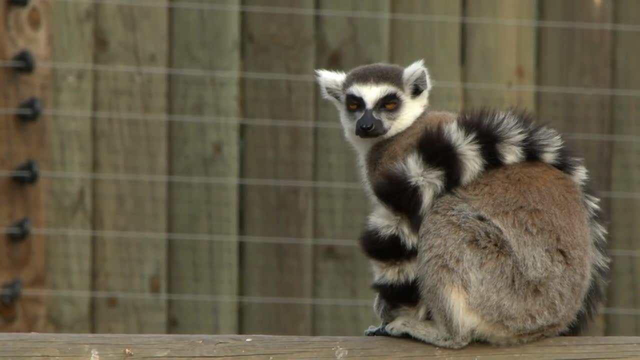 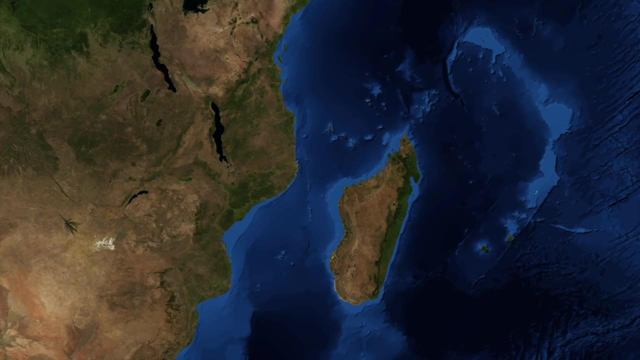 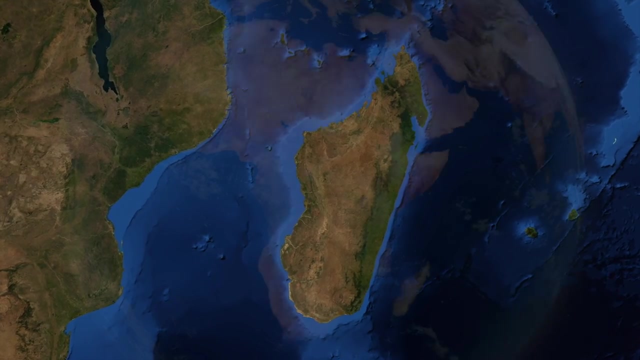 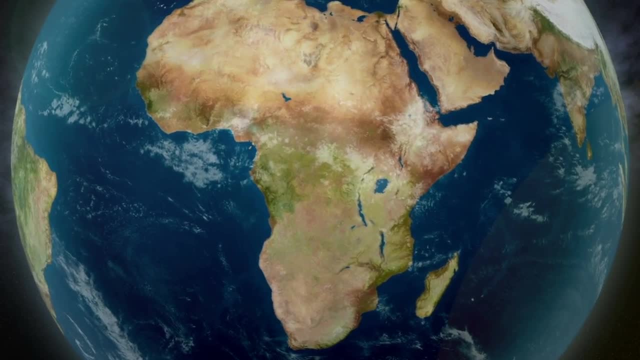 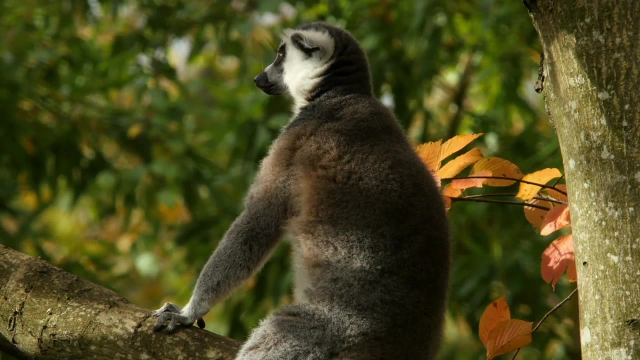 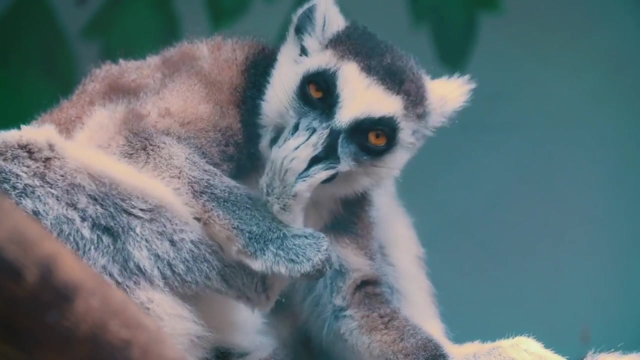 In comparison, Africa boasted a mere 12 species and the Indian subcontinent only three. The implication could not have been clearer in Slater's mind: Madagascar had to be the primordial homeland of these tree-dwelling mammals, from which the Asian and African varieties were derived. 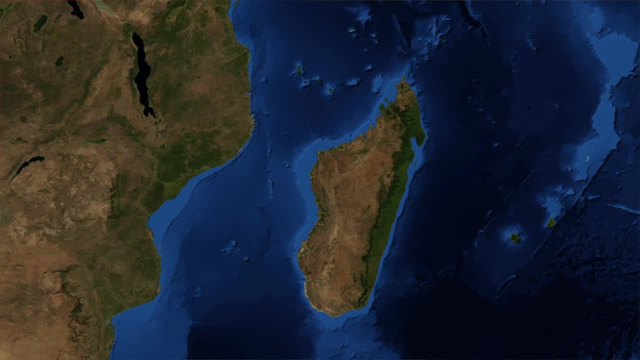 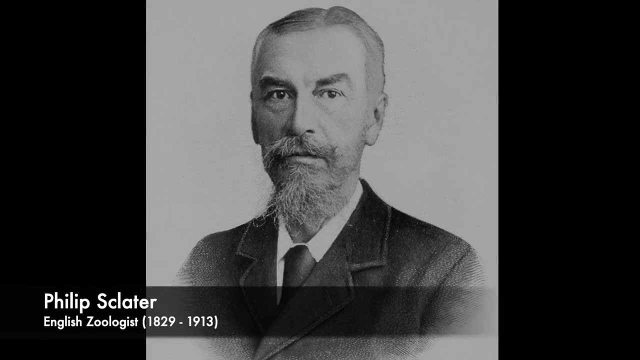 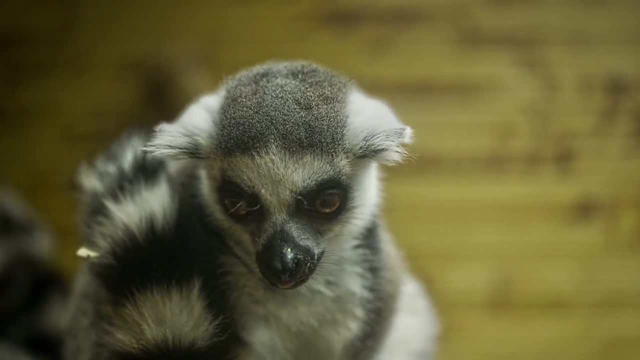 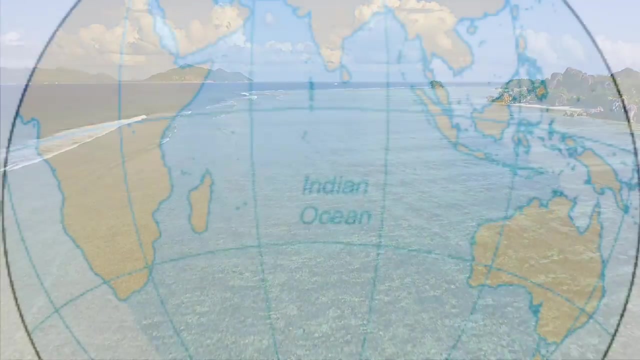 But how had they crossed the great oceans between? Slater was once again confident in his conclusion. They must have travelled overland Across a land bridge that had once connected Asia, Madagascar and Africa. Such a bridge must have been gigantic. It must have been gigantic. 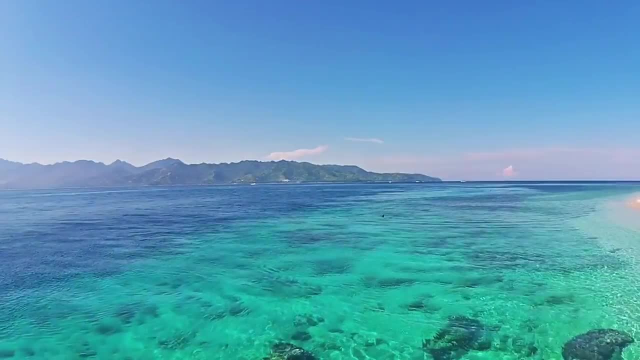 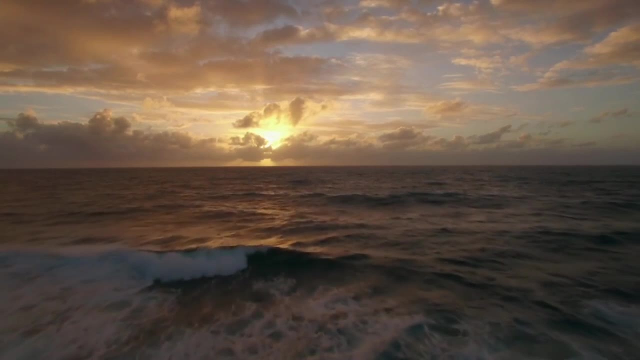 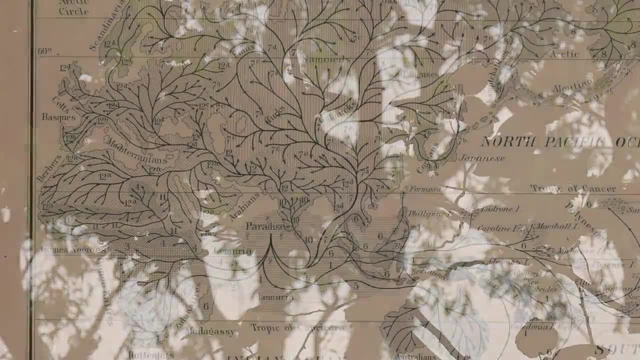 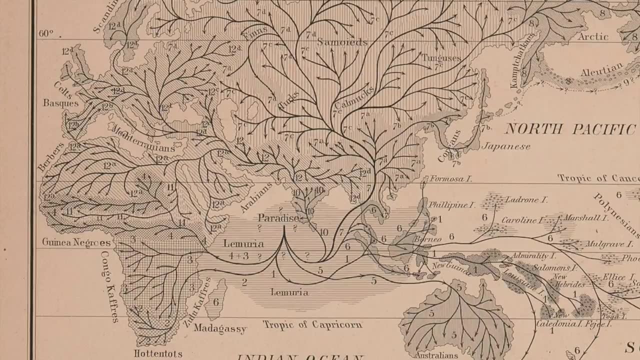 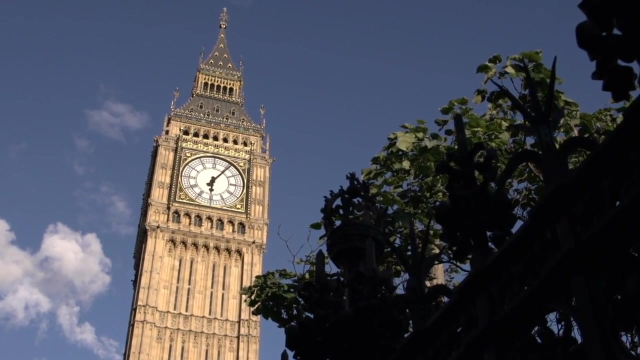 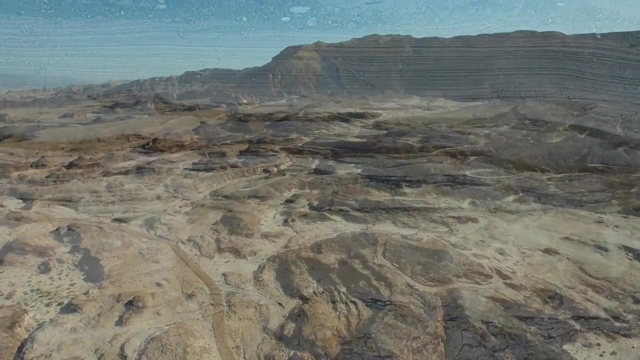 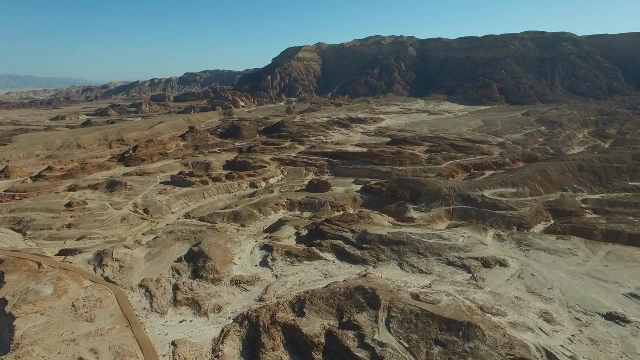 to flow out of their homeland Lemuria. At this point of the 19th century, the land of the Lehmans was now under the control of という. 2013, it the sort of ab 1975. I'd heard of the. 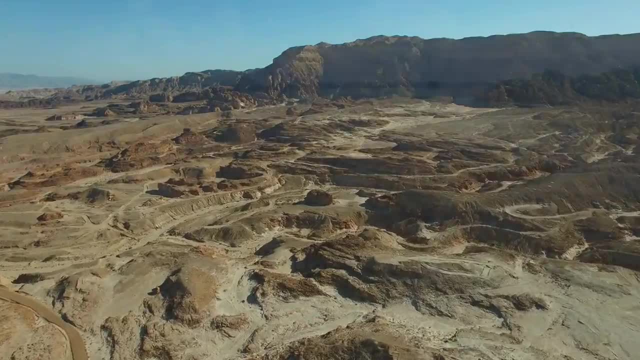 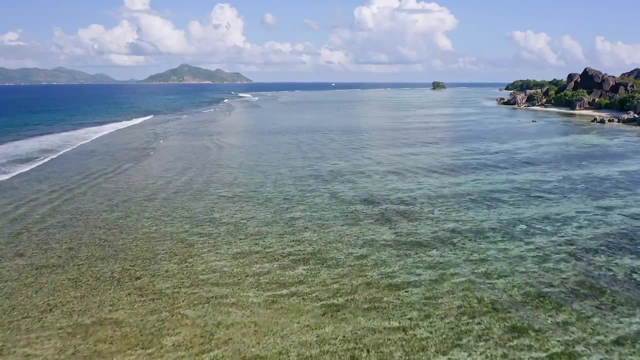 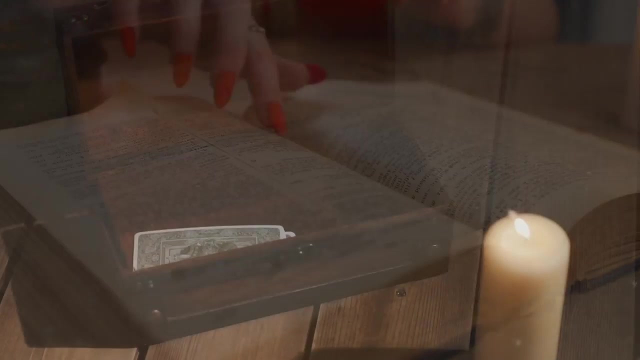 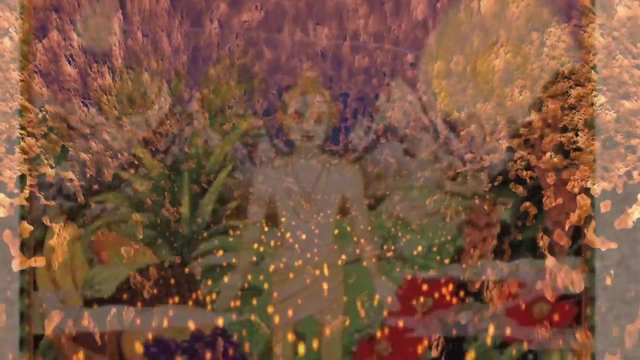 nativist Texas entity called Udall. He was like more of a liberalologist. He thought about what would happen in 2006.. But the following decades would see his ideas seized and transported outside the realms of science and ultimately into the occult. 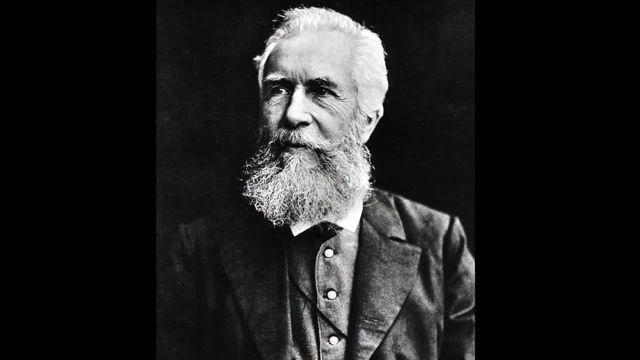 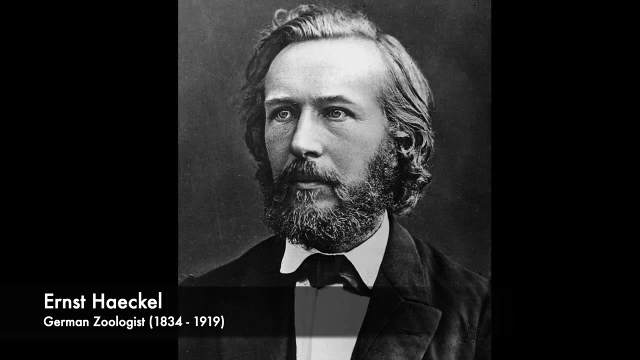 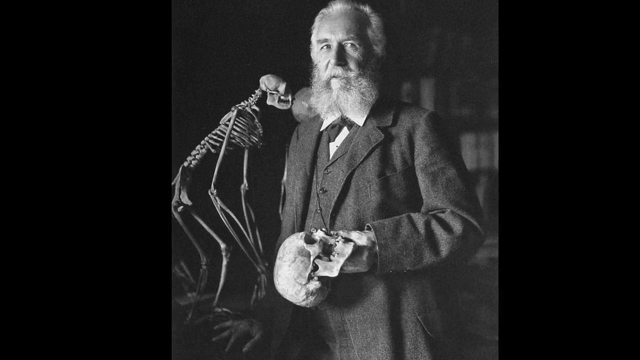 In 1876, a new rejection of the theory of evolution was published by German zoologist Ernst Haeckel. His History of Creation not only rejected Darwin's suggestion that humans had evolved and radiated from Africa, preferring an Asian origin instead, but suggested it was Lemuria. 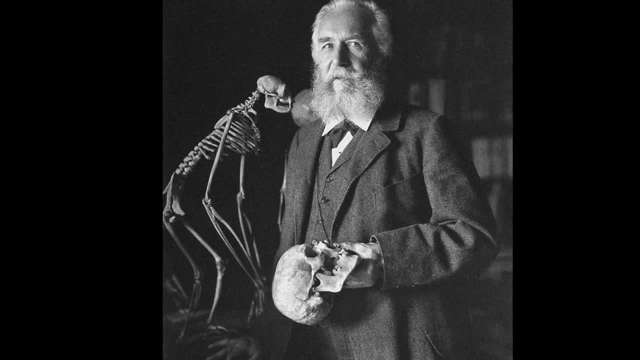 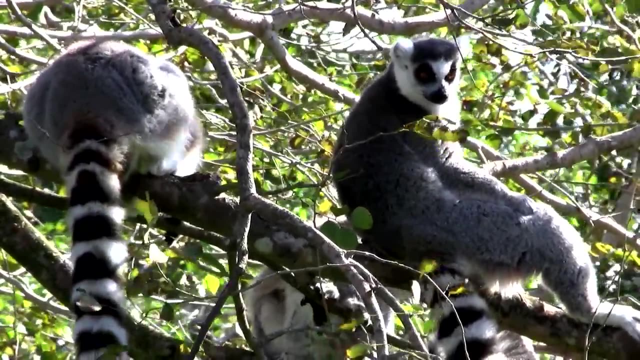 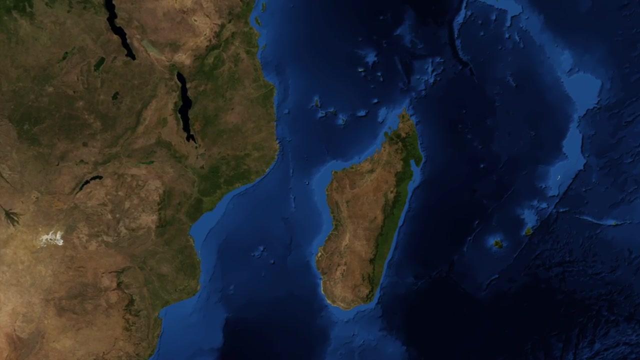 that the lost cradle of humanity could be found. For Haeckel, it was here, among the lemurs and the other lower primates, that mankind first emerged, spreading to Asia and Africa before the continent sank. In later translations of Haeckel's work, maps depicting Lemuria in the Indian Ocean. 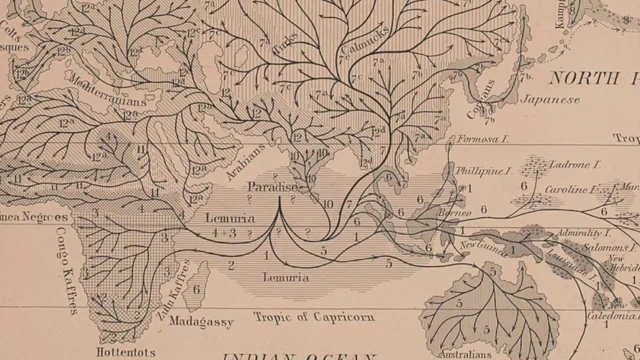 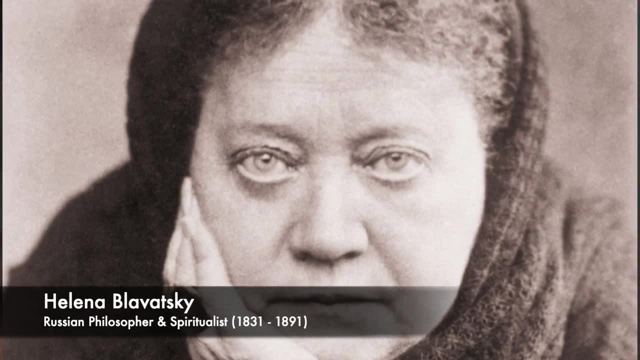 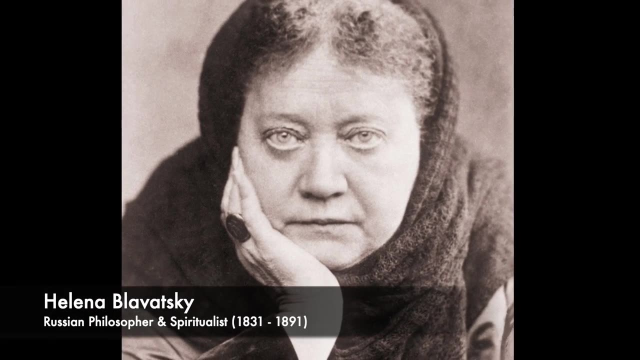 were labelled Paradise. In the decades that followed, the idea was transformed yet further For the Russian medium Helena Blavatsky, whose esoteric religious doctrine, Theosophy, was followed by 45,000 at its peak, including members of high society. Lemuria was the mythical. 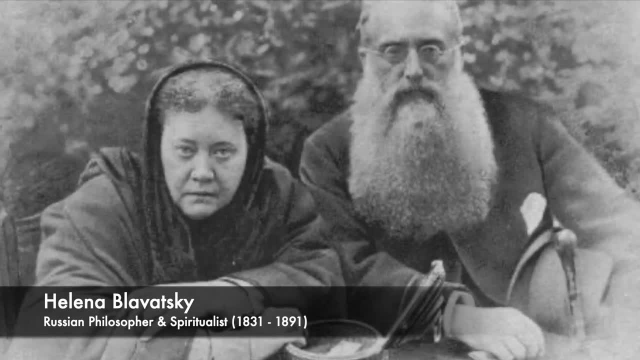 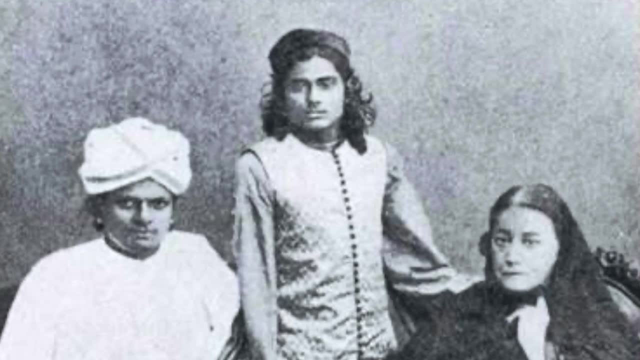 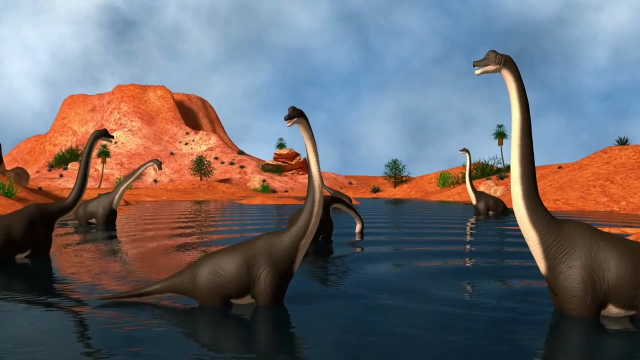 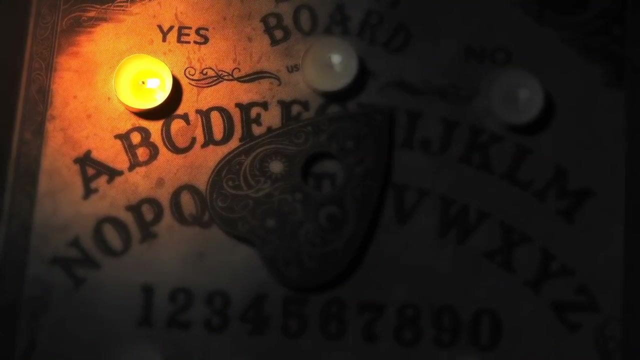 homeland of one of the seven races of humanity, A group of egg-laying hermaphrodites endowed with four arms and four eyes, who had lived alongside dinosaurs on the lost continent until its fiery, destructive end. The concept of Lemuria, from its well-intentioned scientific beginnings to its strange transcendence. 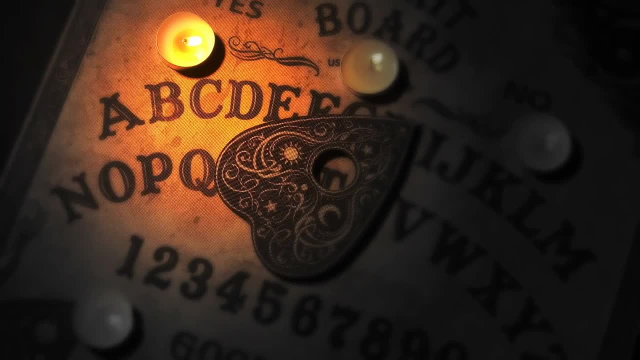 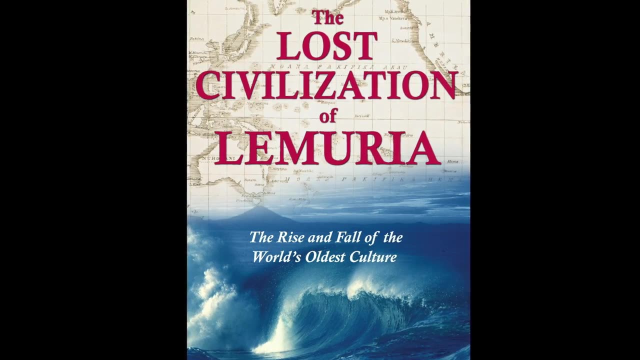 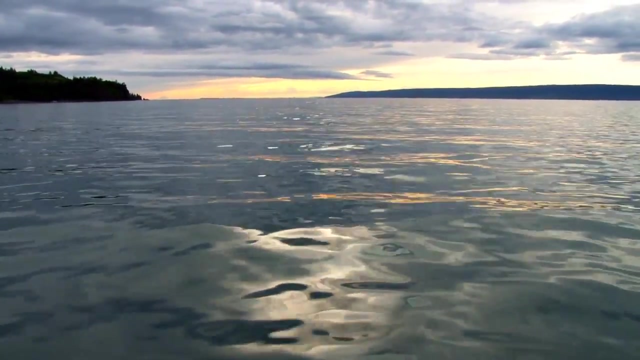 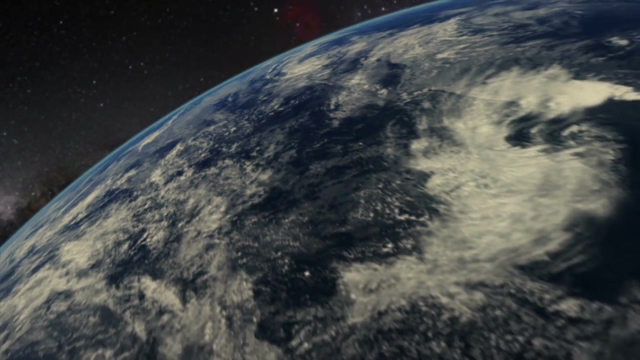 into the occult was one that nevertheless persisted well into the 20th century. It wasn't until modern theories of plate tectonics came to the fore that the lost continent was finally sunk, And so the last 60 years of geological and geophysical study have revealed an altogether 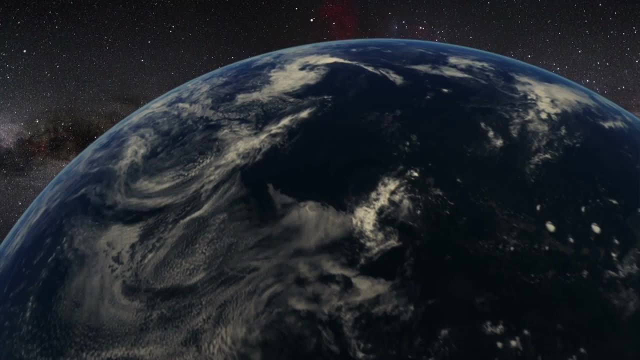 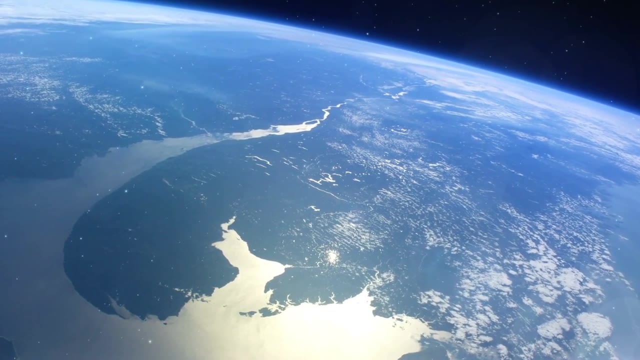 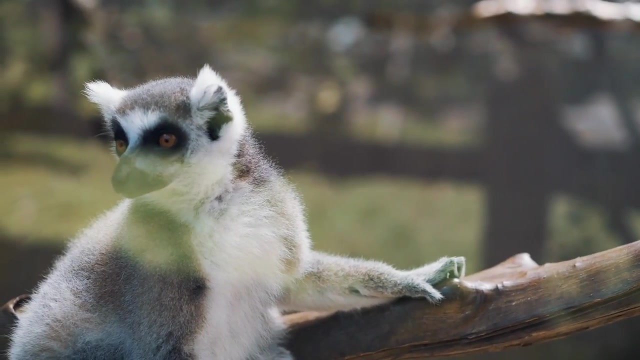 more provable history of continental movements through time. Rather than merely rising or sinking, they traverse the globe, joining and splitting, building and shattering. Lemuria may never have existed, but we now glimpse an even more evocative past. The world has been divided into two parts. 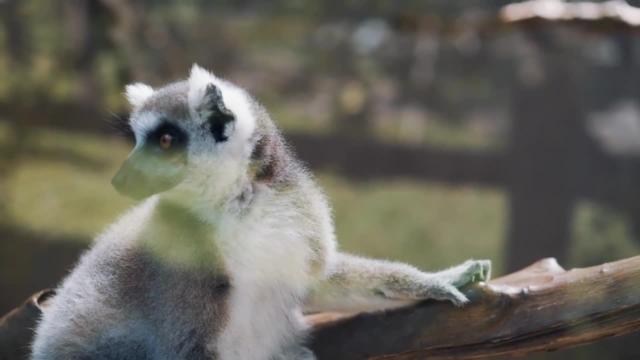 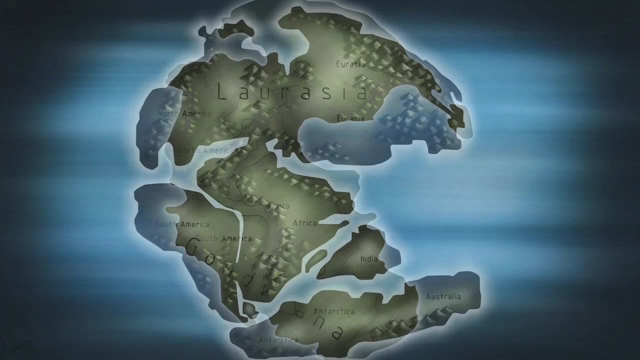 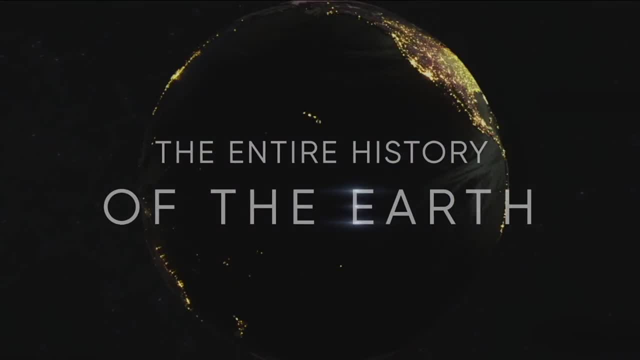 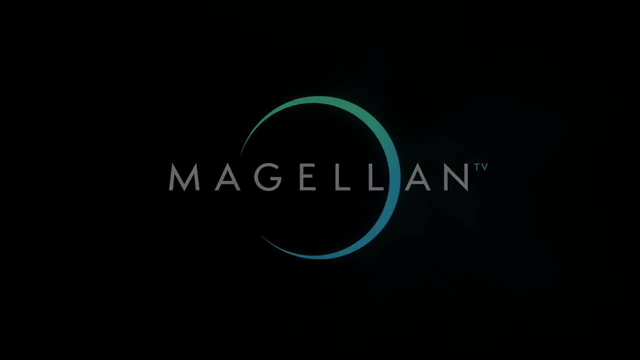 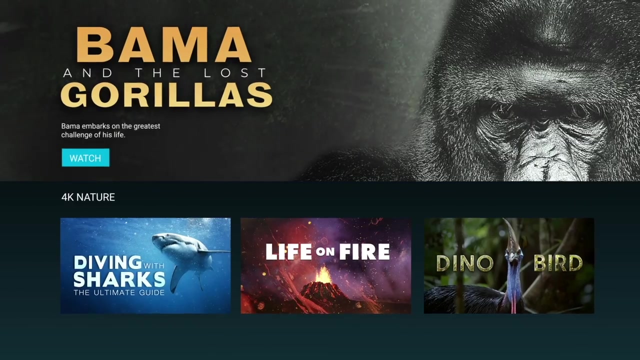 This video is sponsored by Magellan TV, the documentary streaming service. Magellan have been great supporters of the channel for a while now. They offer a vast range of programs on a truly comprehensive range of topics, more than 3,000 in total. 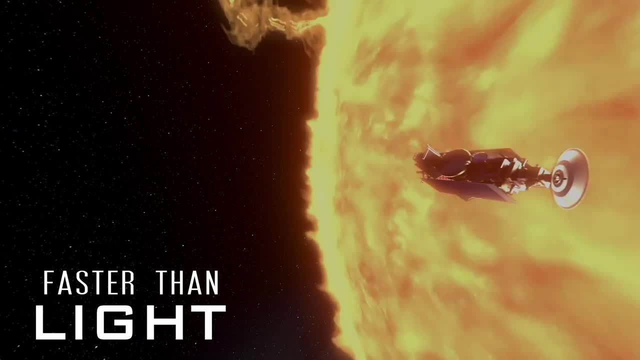 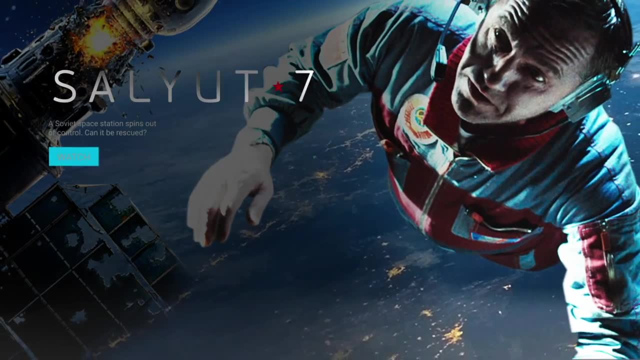 From the depths of space to the dinosaurs. there's something here for everyone. Head over to History of the Universe to find out how they've inspired our work, And one Magellan doc that we enjoyed recently that pairs nicely with this video on supercontinents. 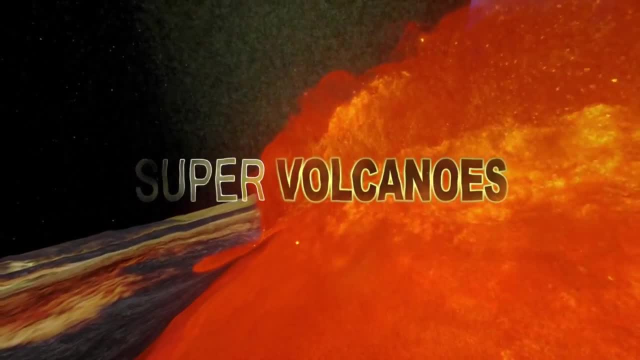 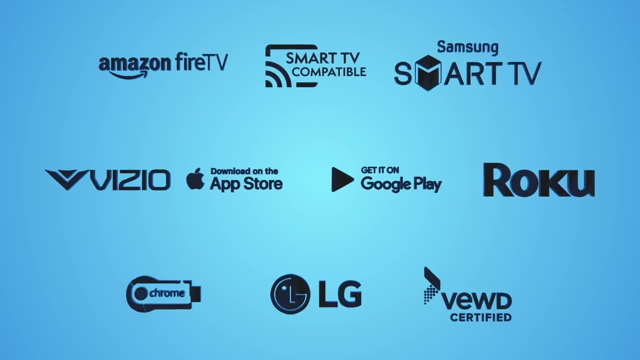 is Super Volcanoes, a fascinating exploration of what makes these earth-shaping titans tick. And you can now take advantage of an exclusive offer: 30% off an annual membership. This gives you an entire year for less than $3.50 a month, even if you've joined Magellan. 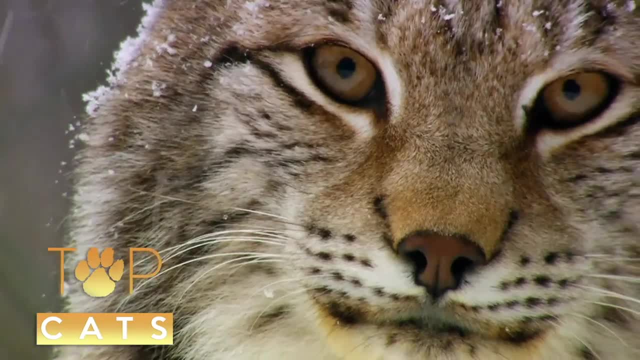 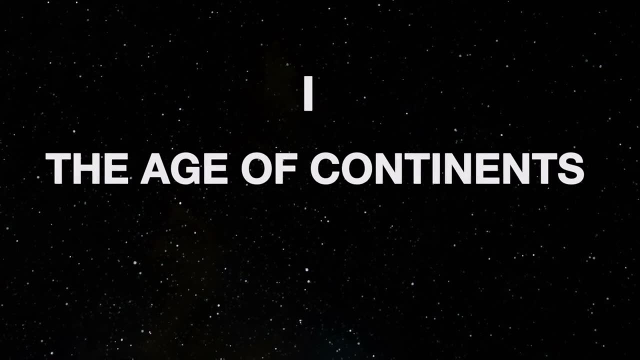 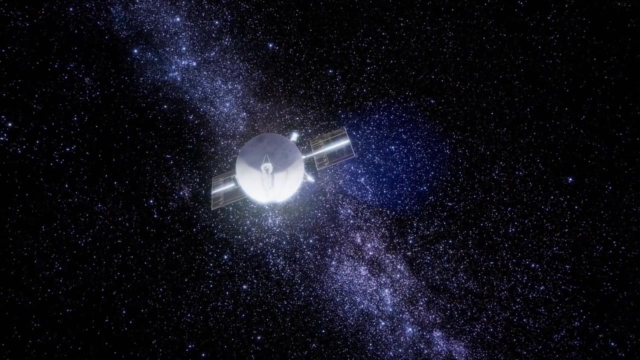 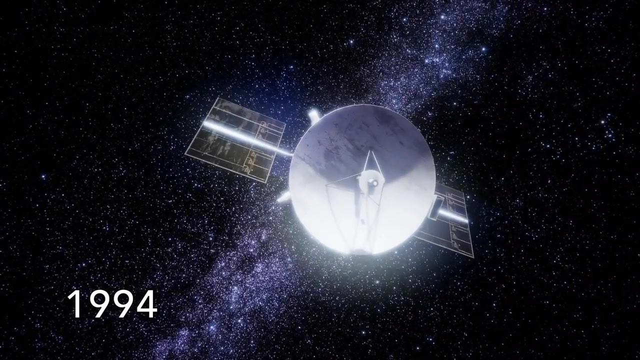 before and lapsed. You can simply click on the link in the description to claim your discounted membership today. I'll leave the link in the description below. Towards the end of 1994, a small spacecraft plunged, whirling into the scorching clouds. 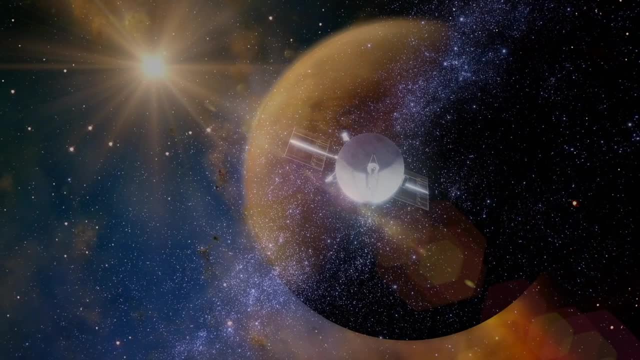 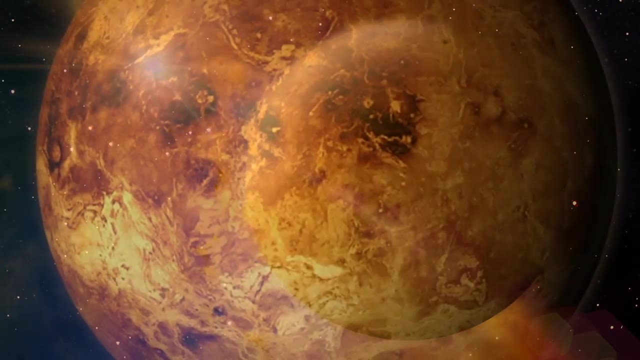 of Venus. It was a small spacecraft plunged, whirling into the scorching clouds of Venus. It was a small spacecraft plunged whirling into the scorching clouds of Venus. It was a graceful death well deserved by a probe that had accomplished so much in its 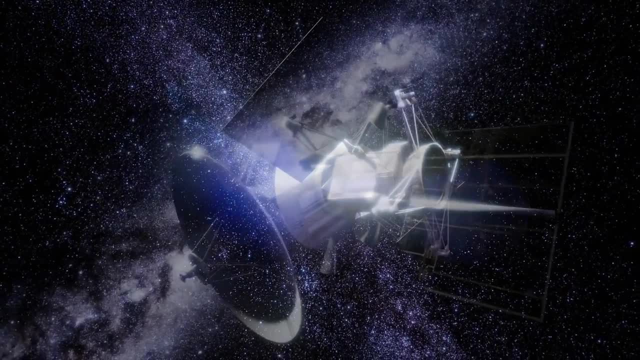 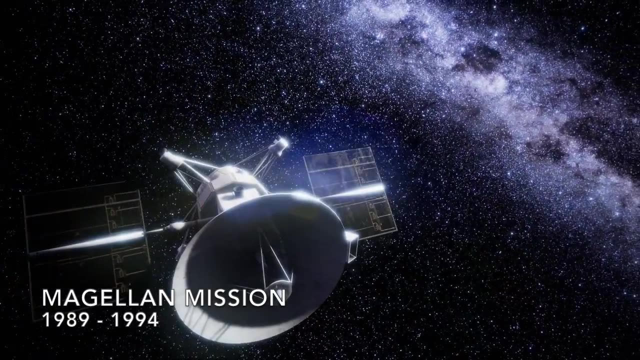 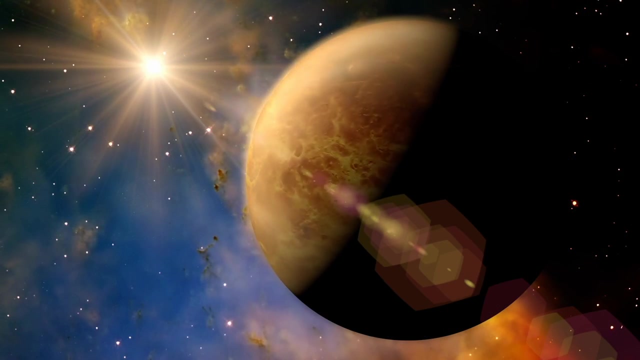 short life. For the last four years, the Magellan probe had been swooping past the shrouded planet in great polar loops, passing from north to south just 300km above the surface, before swinging far out back into space to prepare for another pass. 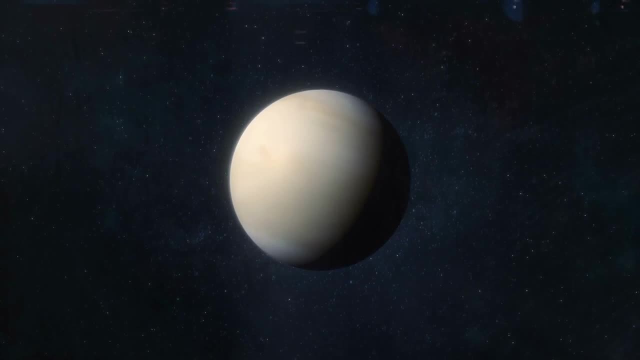 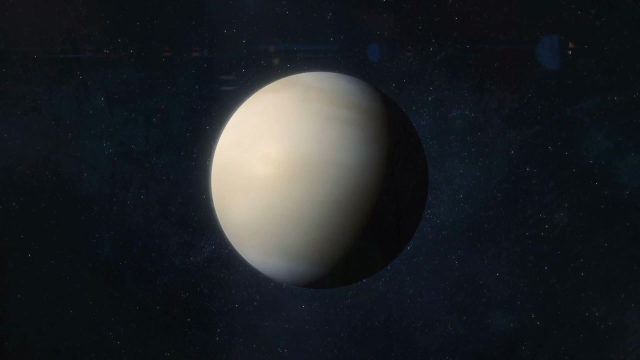 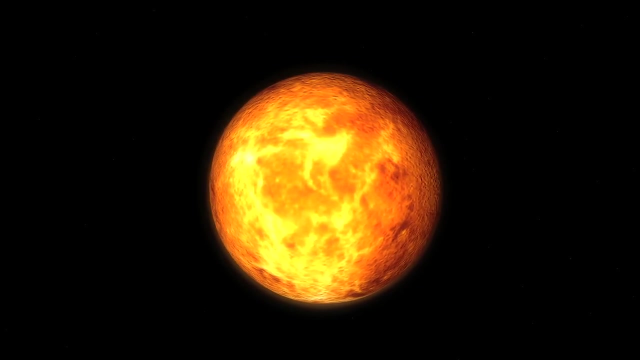 With each transit as the planet rotated serenely beneath its clouds. Magellan imaged a new swathe of the Venetian surface, But normal cameras would not suffice here. Earth's twisted neighbour is so thoroughly wrapped in cloud and haze that visible light 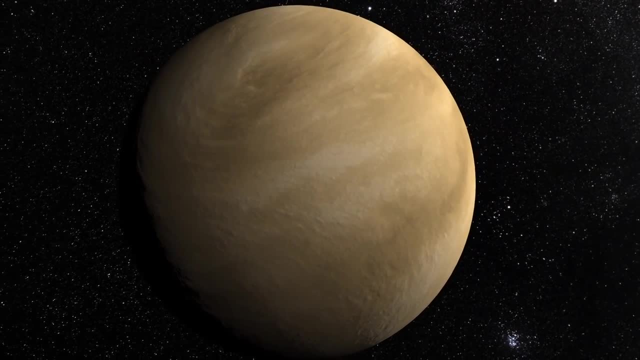 could not hope to penetrate. Instead, Magellan scanned the alien surface with radar and in less than two years had mapped 98% of the planet's surface. This was the first time Magellan had scanned the alien surface with radar and in less than two years had mapped 98% of the planet's surface. 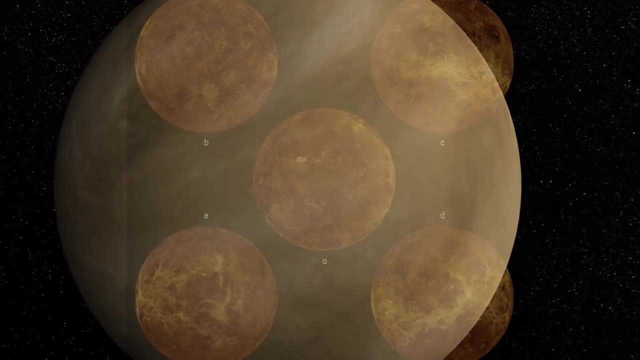 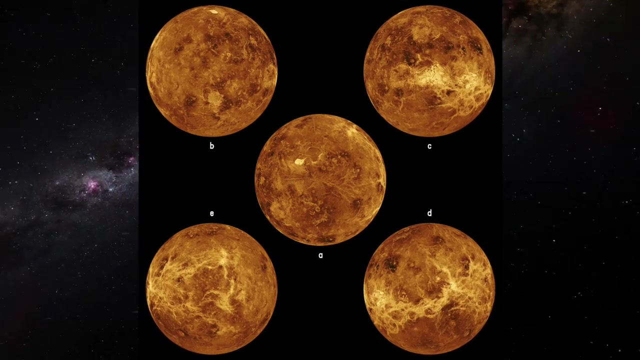 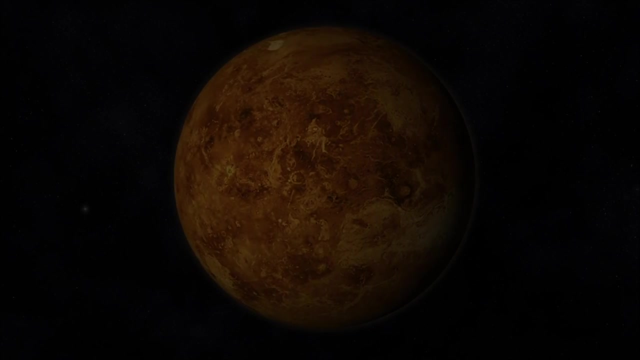 This was the first time Magellan had scanned the alien surface with radar and in less than two years had mapped 98% of the planet's surface. But the radar images revealed something strange. Venus seemed to have no continents at all, Despite being so similar to Earth in size and rocky composition. the swaddled planet. 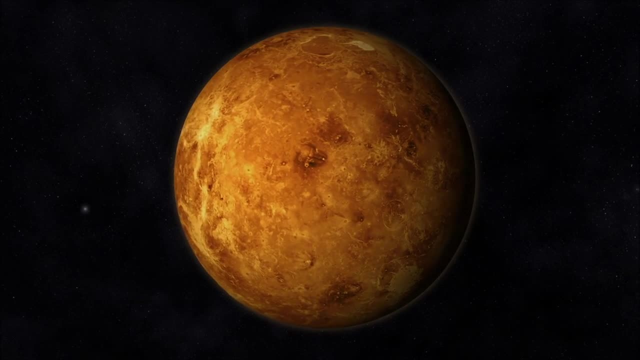 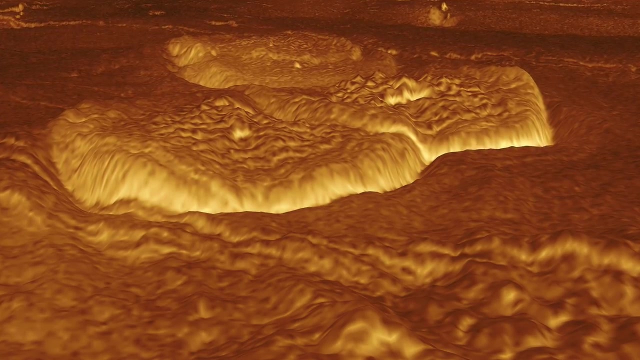 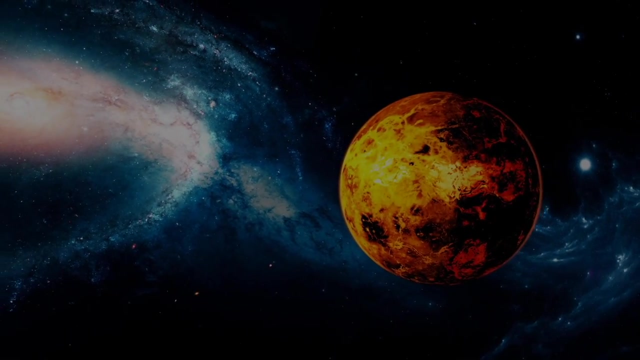 seemed to have none of our surface diversity. Magellan saw plenty of volcanic features, from shield volcanoes to vast lava fountains fields, but they were all hallmarks of a single basaltic rock: No sedimentary deltas, no metamorphic mountains, no explosive stratovolcanoes. 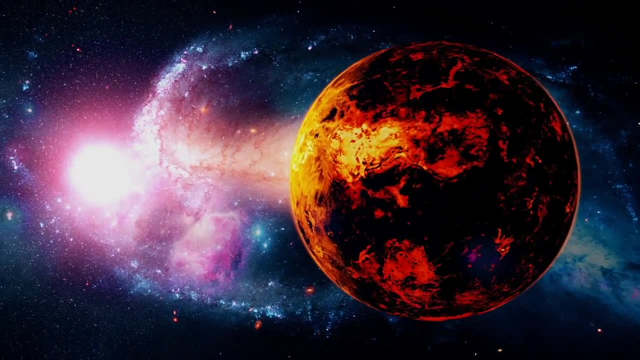 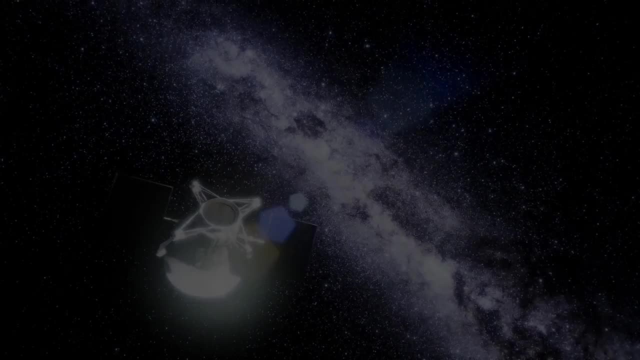 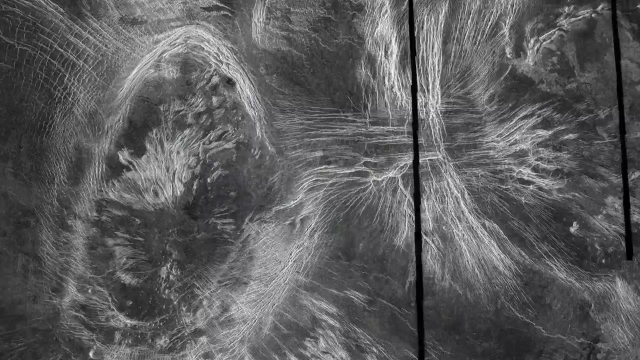 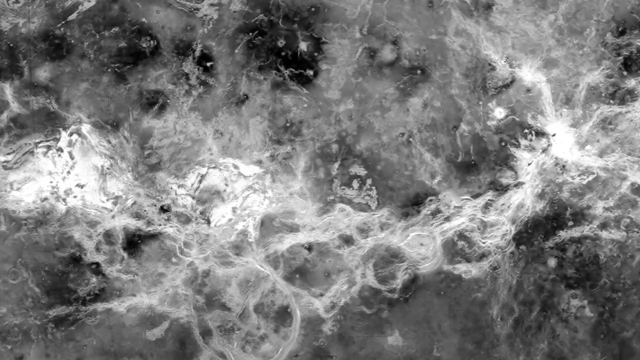 Only dark fluid lava over the planet's entire surface. Magellan's data was invaluable to scientists trying to understand how Venus became Earth's evil twin. The radar images revealed that the plate tectonics that defined our surface never really played a role on Venus. Without the lateral movement and recycling of the crust, there was nothing driving the creation of new types of rock. Without a tectonically driven rock cycle and being positioned that much closer to the Sun than Earth, Venus's conditions spiralled out of control. 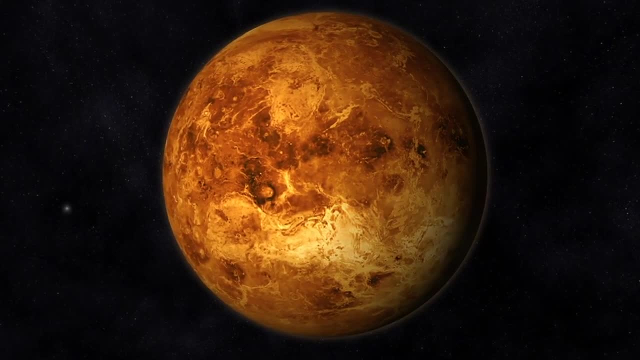 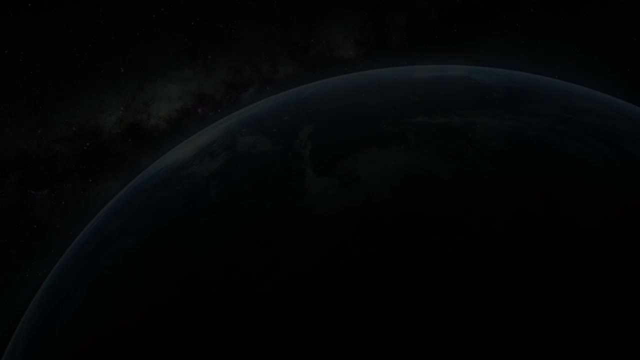 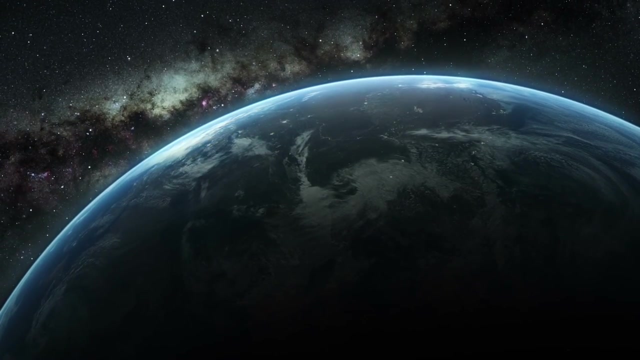 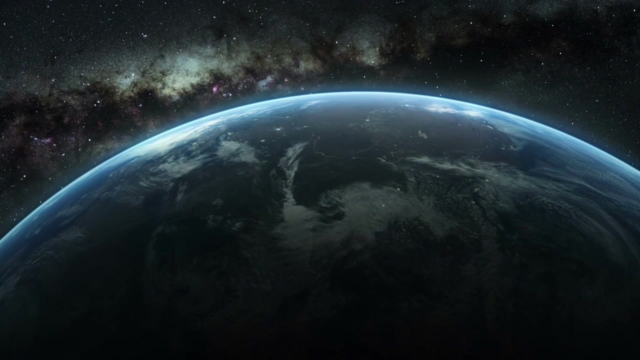 Without plate tectonics, the planet was baked alive. Earth was dealt a luckier hand. The beginning of plate tectonics established a feedback cycle that has protected us from Venus's fate for the last three and a half billion years. 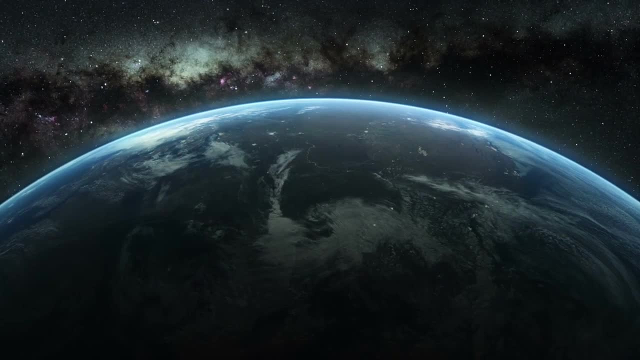 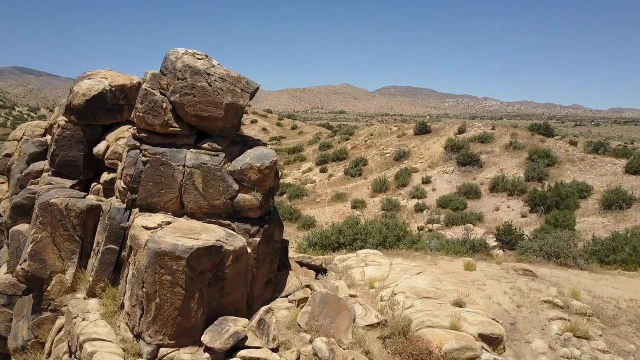 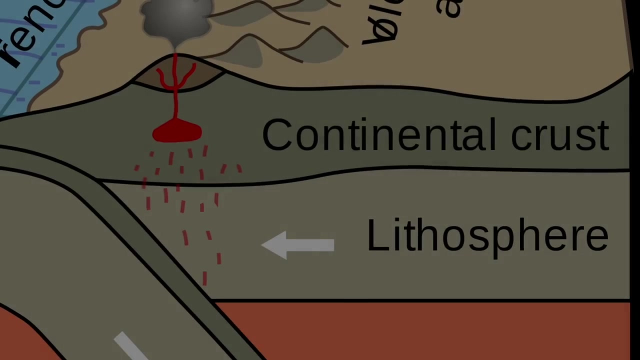 Those plate tectonics have also endowed our planet with a startling variety of rock types and we can trace the first continents of the planet, The first continents of the planet, The first continents of all, To those earliest creeping moments. Continental crust is special. 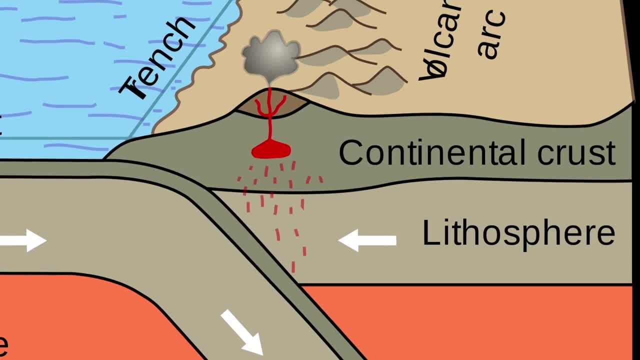 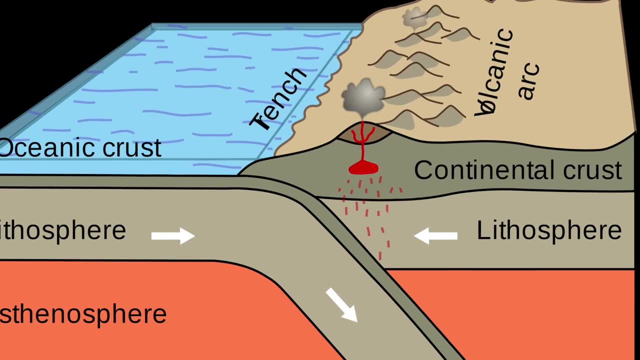 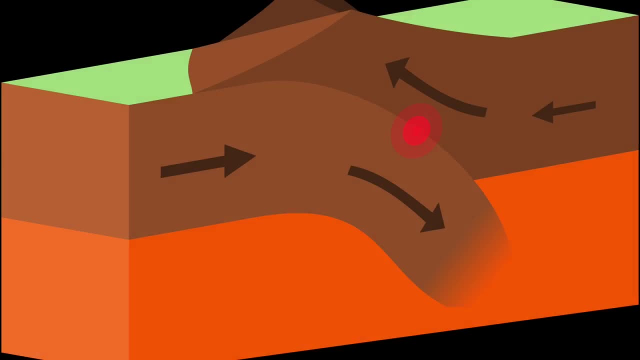 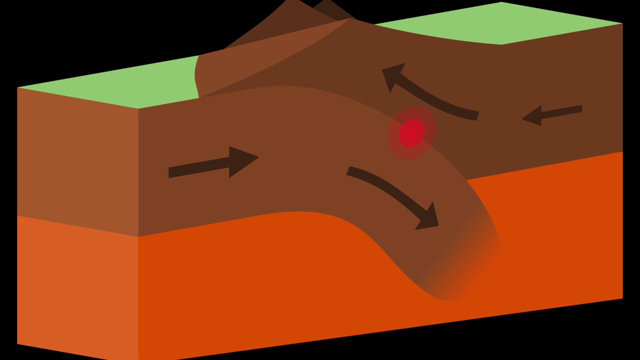 It has a distinct and refined composition, like a fine whiskey to the raw grain mash of the oceanic crust. As plates collide, they crumple and thicken, allowing molten rocks to sit for longer in the heart of the crust. Here they partially crystallise, losing their heavier minerals and becoming progressively. 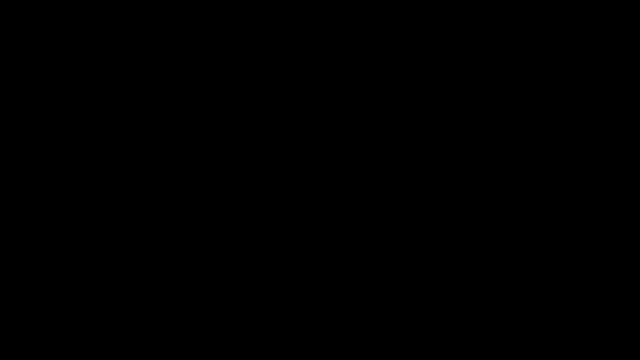 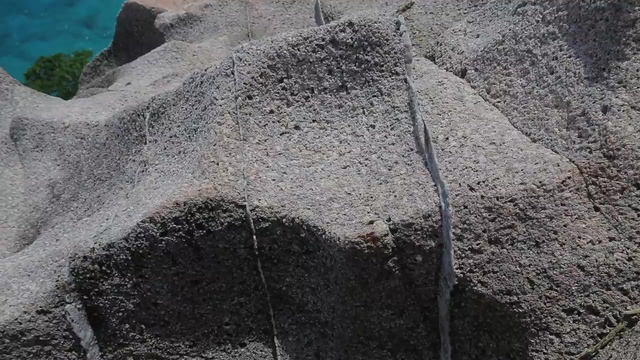 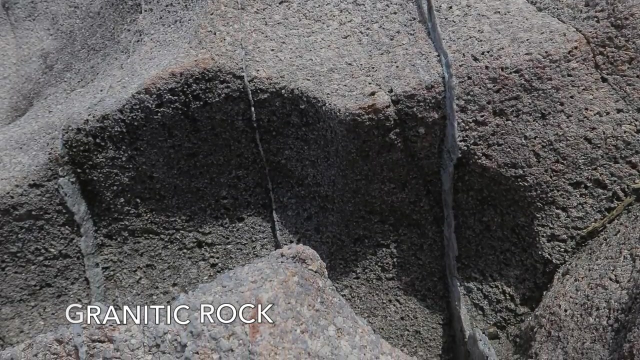 lighter and less dense. It is these relatively lightweight granitic rocks that are the foundation of our continents, And they have been gradually accumulating ever since plate tectonics began. The first continents of the planet. The first continents of the planet. The first continents of the planet. 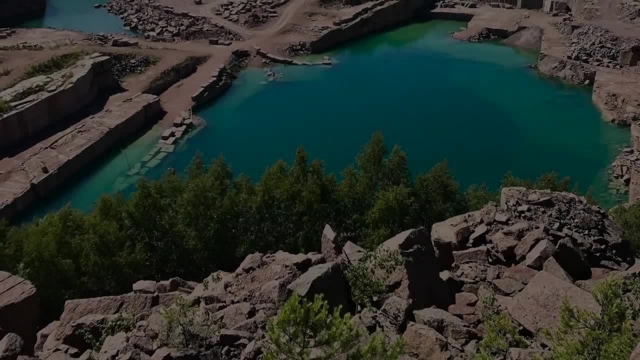 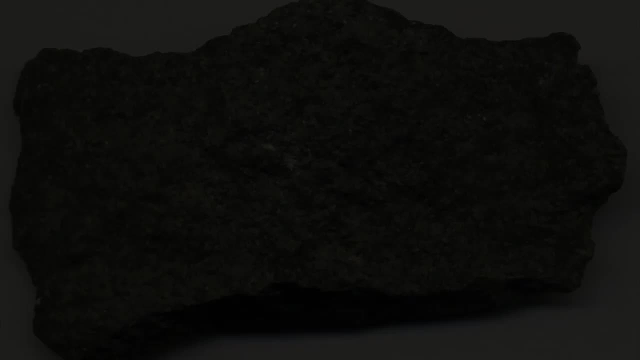 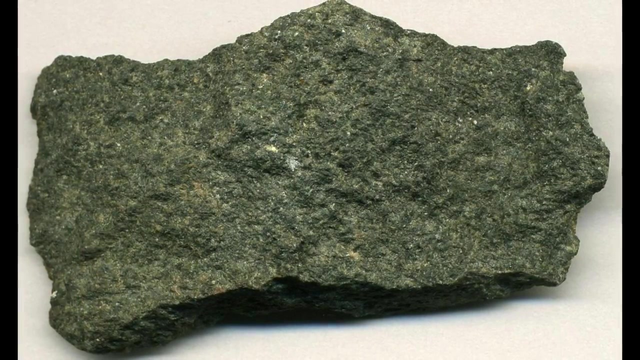 Because of their lower density, they float buoyantly on the top of the mantle and are not easily subducted at collisional plate boundaries. Instead, it is the denser basaltic oceanic crust that floats lower and is sacrificed at subduction zones. 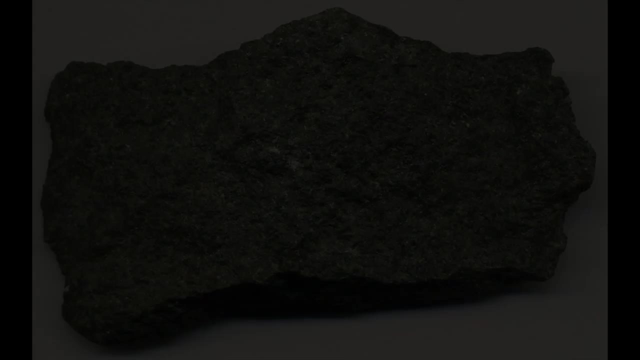 In this way, continents once formed stand proud, bubbling like a cork that won't be sunk. They can be destroyed, of course, by the forces of wind, water and sand. In this way, continents once formed stand proud, bubbling like a cork that won't be. 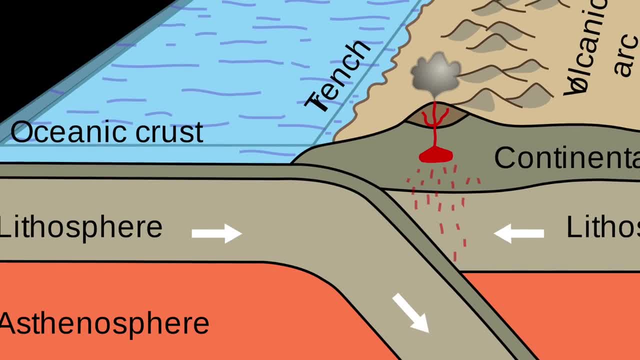 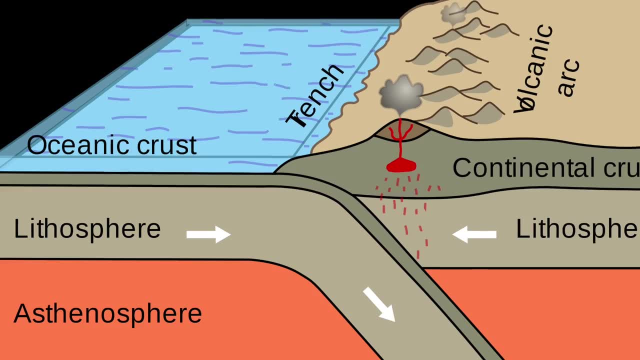 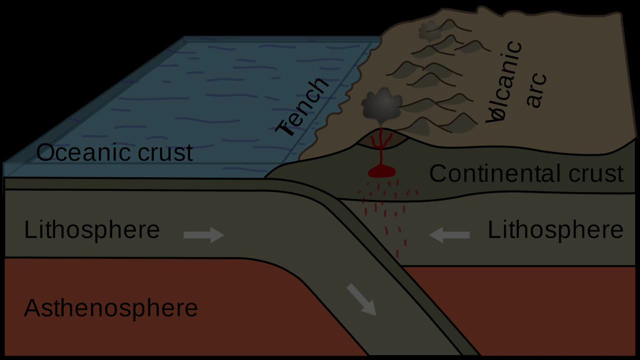 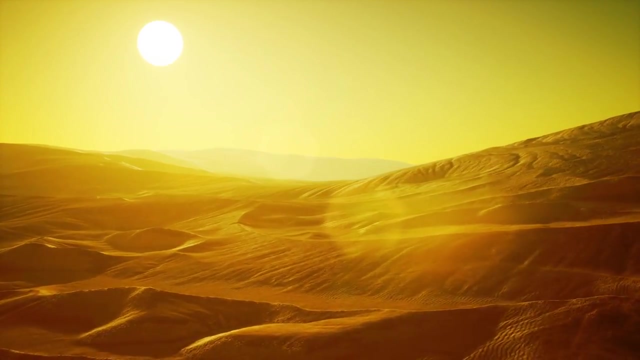 sunk and ice, but in any clash of tectonic sumo, these bulky behemoths will always emerge victorious. The oldest remaining fragments of continental crust today are some three and a half billion years old. They have persisted in the face of erosion, collision and rifting. We know. 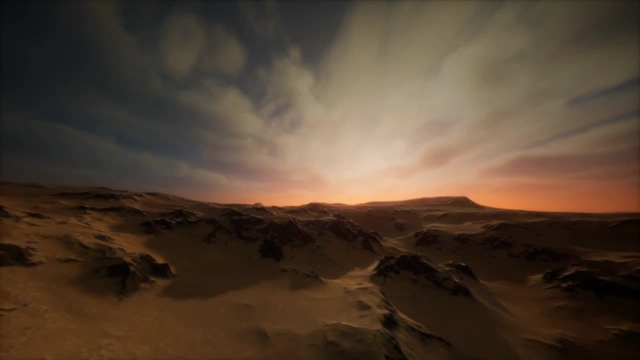 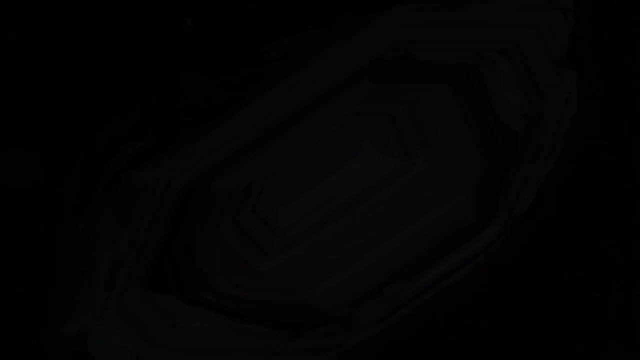 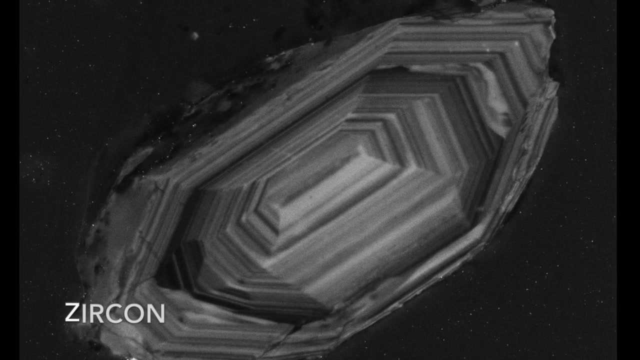 their great age, from mineral crystals called zircons that are some of the most resilient constituents of continental rocks and which contain a precise elemental clock in the form of decaying uranium atoms, By precisely measuring the proportions of original uranium and its decay, 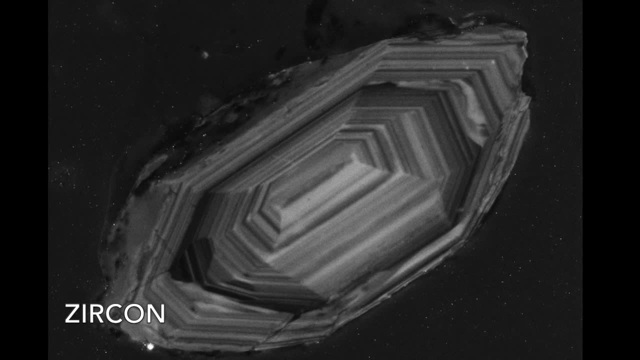 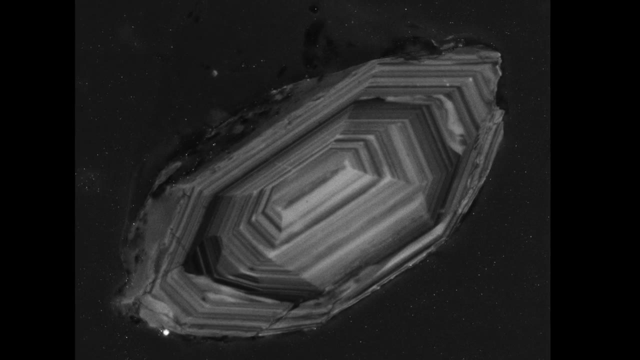 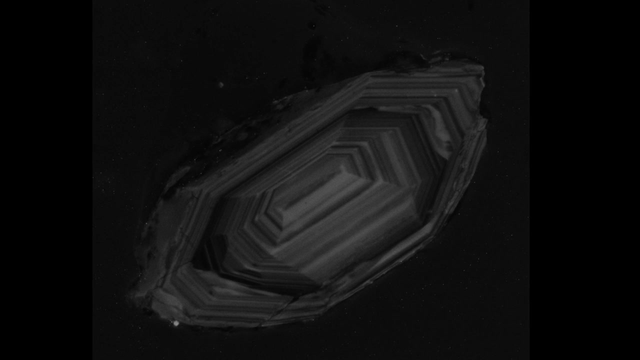 product. lead. geologists can reconstruct the age of the crystal and therefore the rock that contains it. Even after the original rock is eroded away, the zircons will survive to be reincorporated into sedimentary rocks and preserve an echo of the mountain that gave them birth. 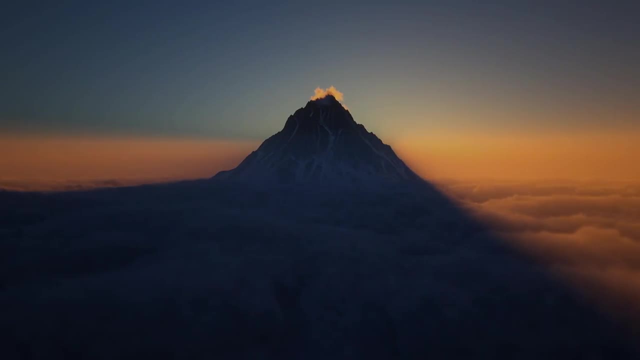 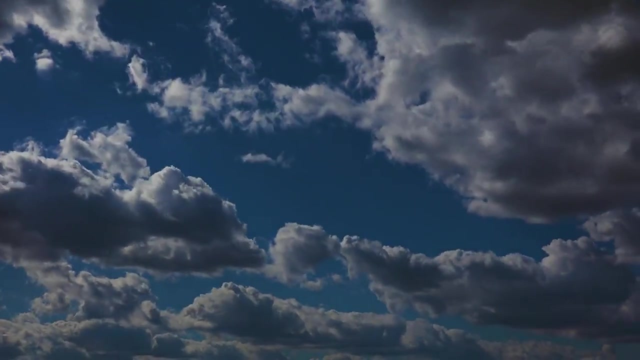 In this way, tens of thousands of zircons have been dated to build a picture of continental crust creation through geological time. More zircons imply more rock formation, but the actual record seems to show that the zircons are not the only ones that have survived. The zircons. 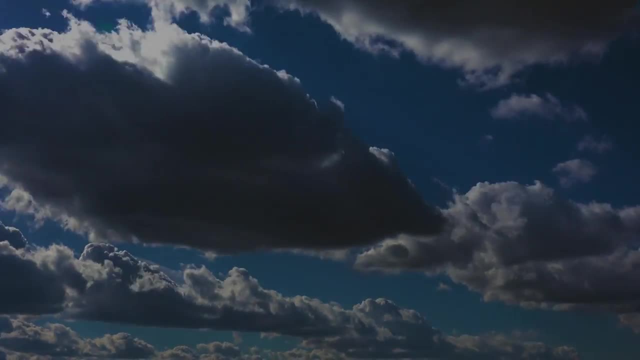 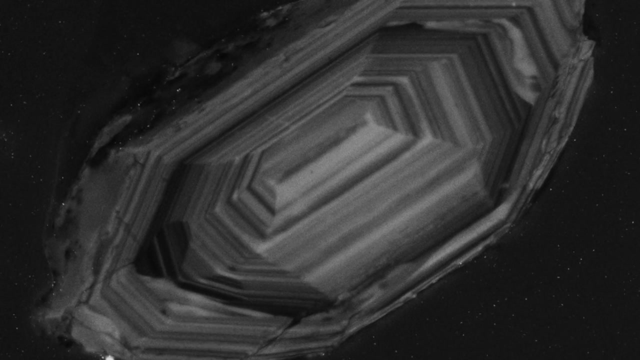 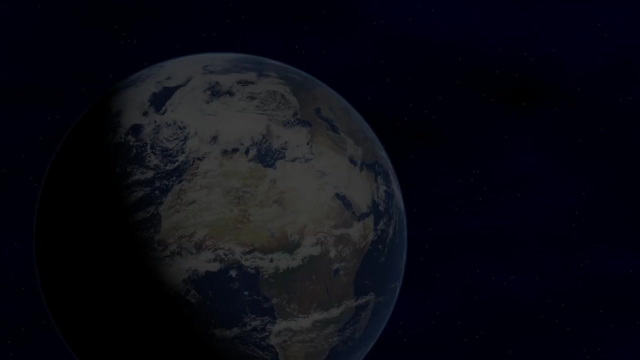 seem to show a surprising pattern. There are times when zircon production is inexplicably low, when continents merely exist and are barely being added to at all. How does this fit with a global picture of plate tectonics? To understand that, we must take a step. 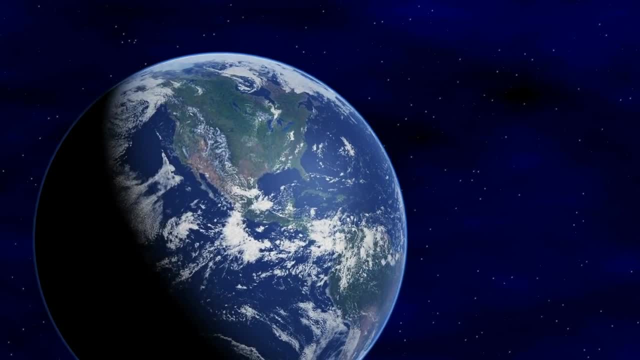 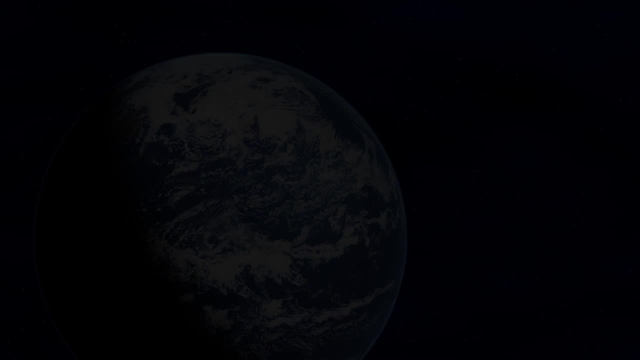 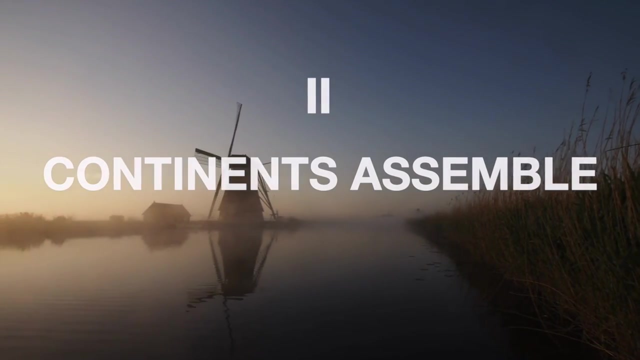 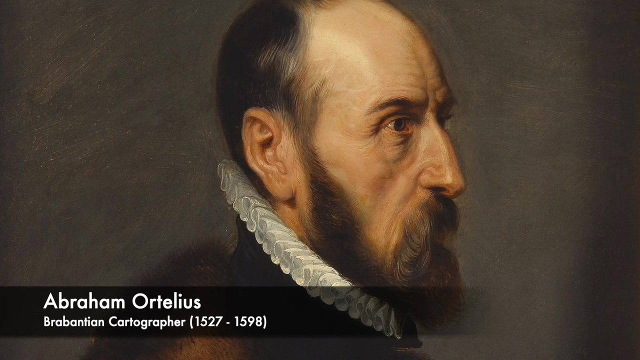 back from individual crystals and search for other clues in the continental fragments preserved. In the 16th century, perhaps no one in the world had looked at Earth's continents quite as closely as Abraham Ortelius, Fascinated by the intricate process and artistry of committing vast swathes. 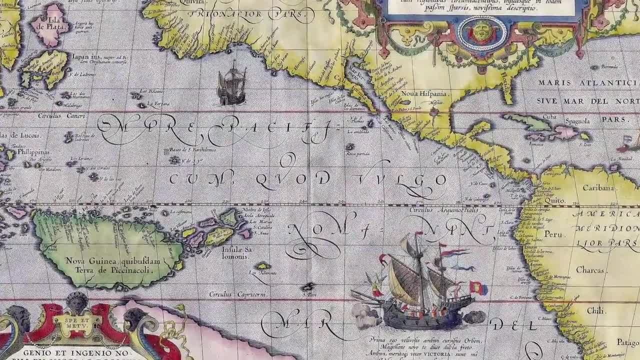 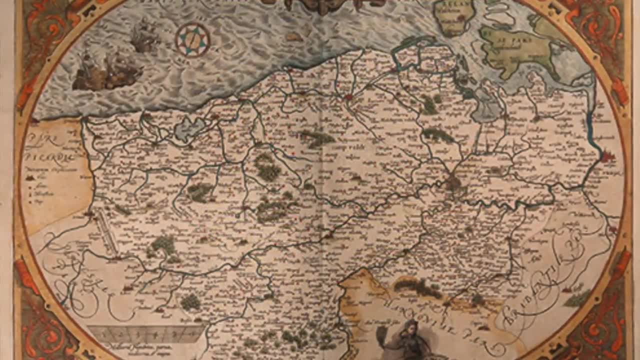 of land to a single sheet of paper. he pursued cartography with almost every waking moment. It is little wonder, then, that this influential geographer saw something in the shape of the world that none had given voice to before. The coasts of Europe, Africa and the Americas seemed to. 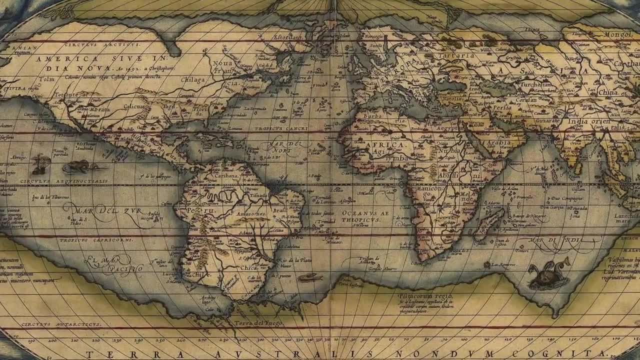 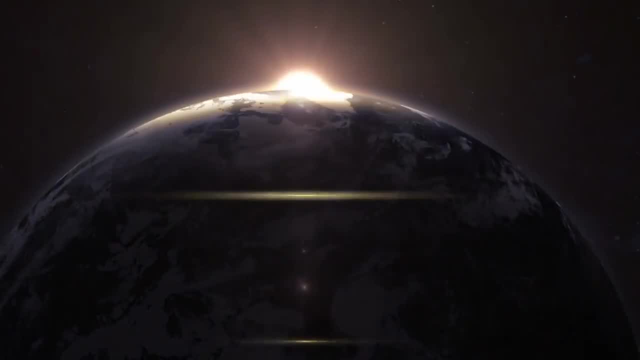 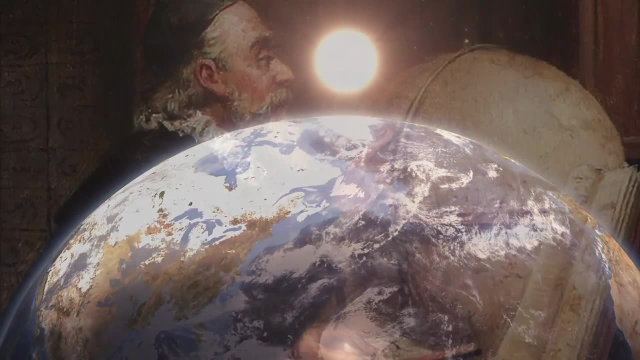 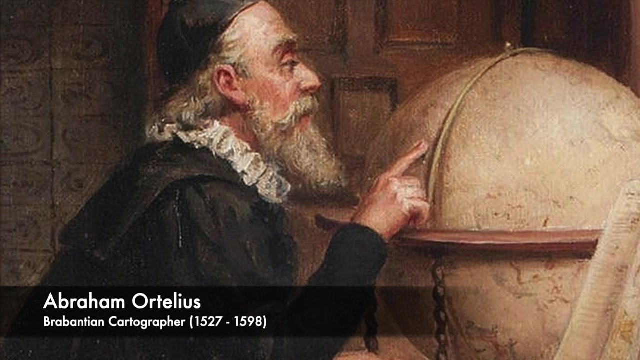 match one another. Ortelius imagined these continents ripped apart, as he described it, by devastating earthquakes and floods. Arguably, he was the first to imagine the Europe of crusts and crusts, imagine the concept of continental drift, an idea which wouldn't truly be popularised. 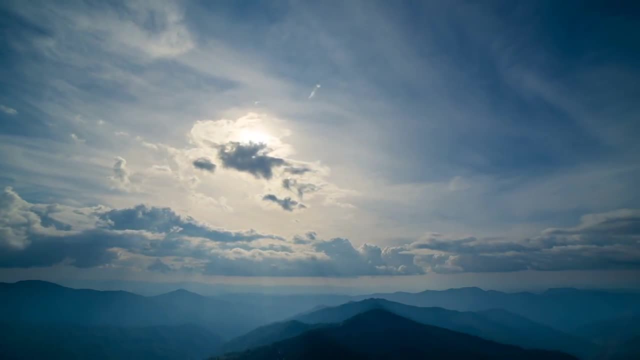 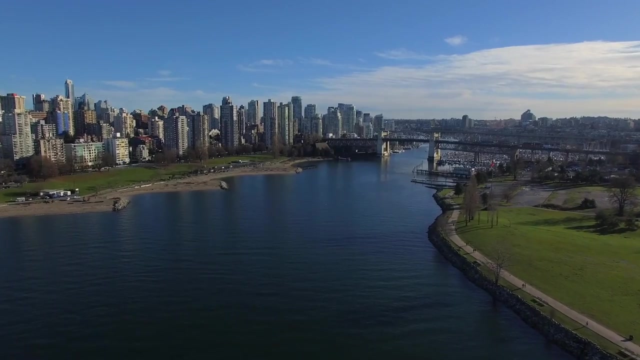 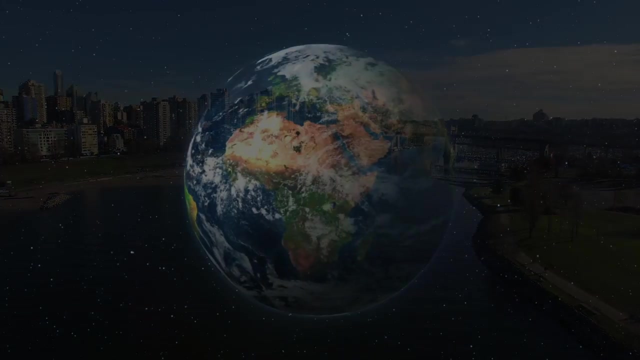 until the early 20th century by the meteorologist Alfred Wegener, For it would be nearly 400 years before modern scientists could verify that the Dutchman's suppositions were in fact correct. Africa, Europe and the Americas had indeed once been. 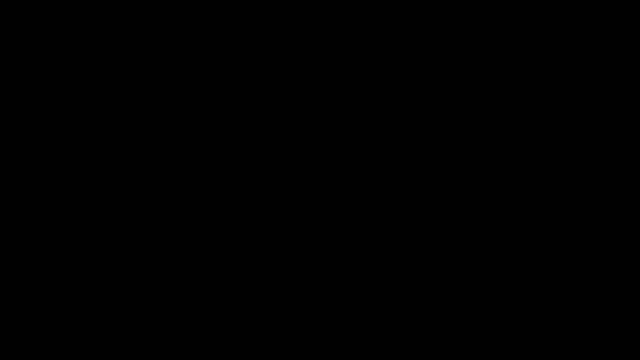 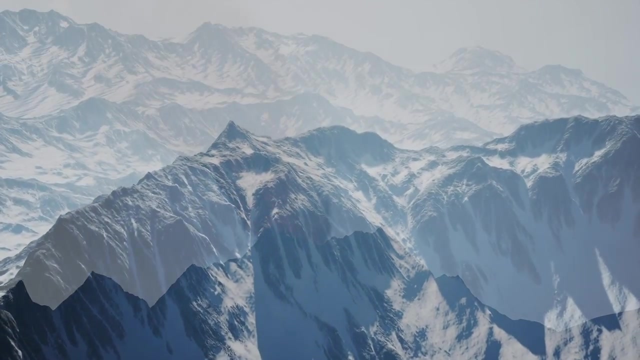 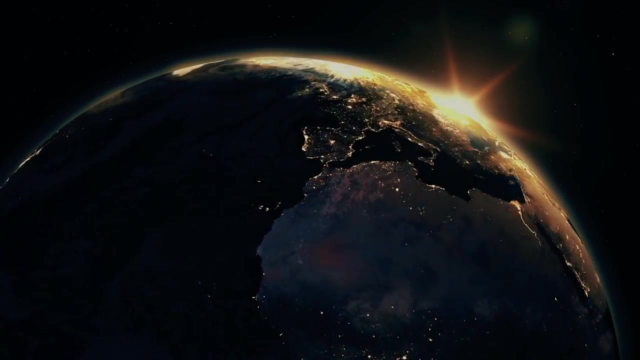 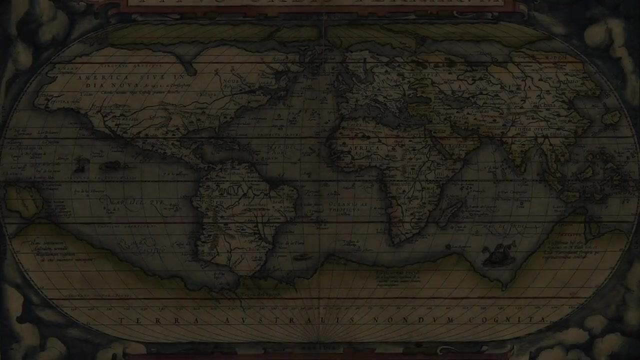 joined and had been torn apart by the inexorable forces of plate tectonics. Earthquake and flood was just the beginning of the catastrophe that befell these once united continents. As Ortelius contemplated the shapes of shorelines on his 53-page atlas of 1565, he was unknowingly 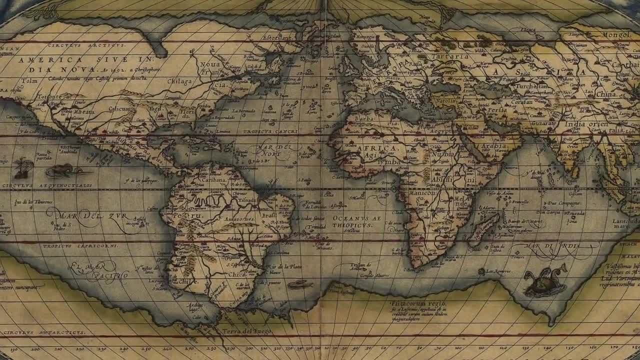 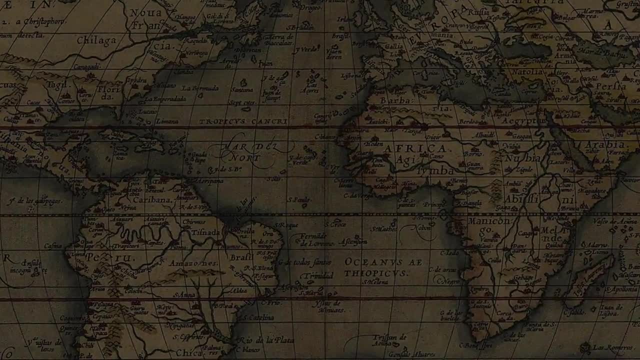 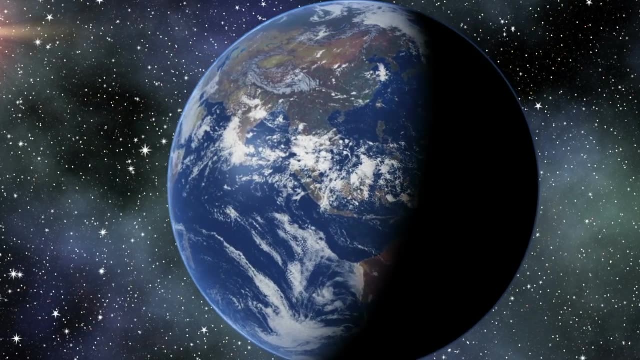 tracing the open wound of a supercontinent Ripped asunder. There are no supercontinents on Earth today. The largest discrete landmass is Eurasia, with an area of around 55 million square kilometres, But even this gigantic continent makes up. 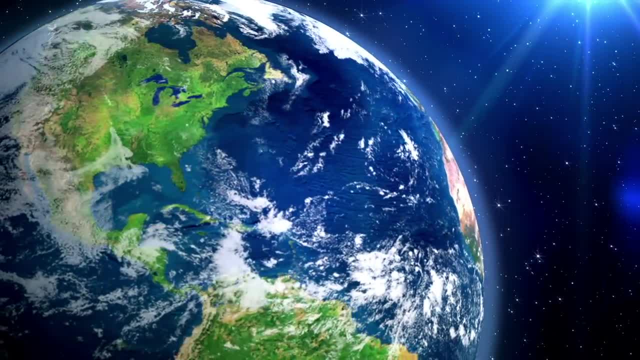 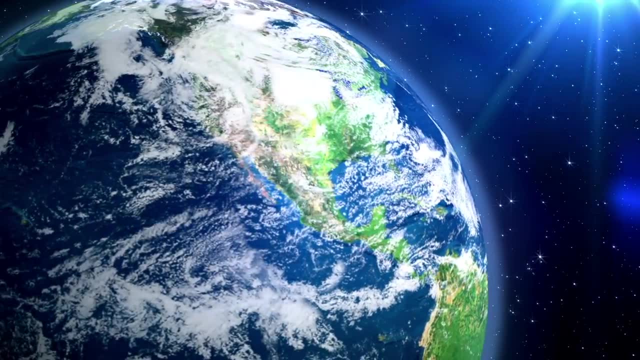 little more than a third of all the land area on Earth. Various definitions of supercontinents require that all or nearly all of the Earth's continental crust be gathered in one single area, A single immense and unbroken landmass. 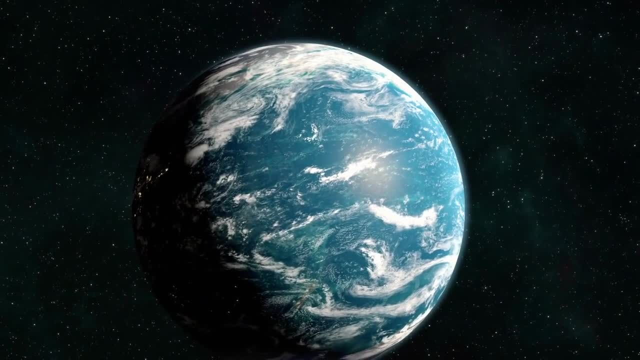 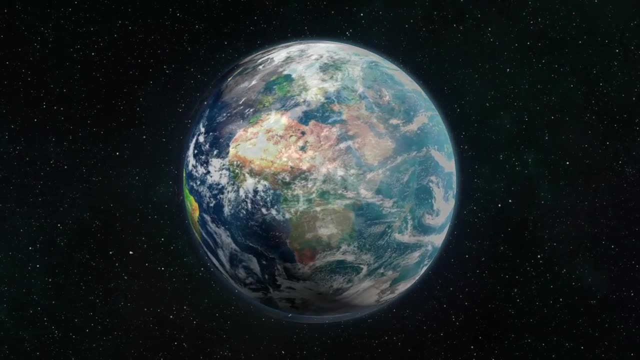 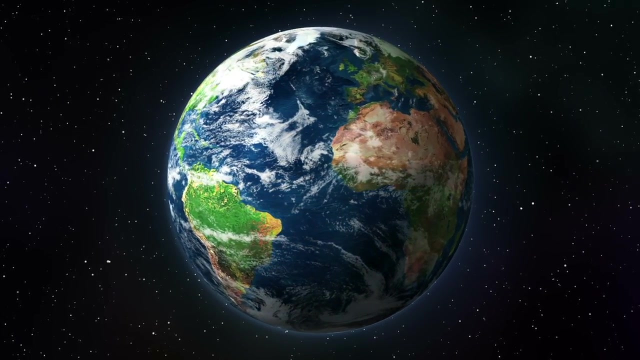 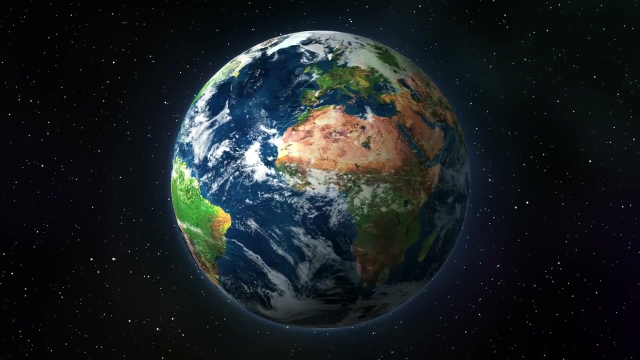 Alternatively, some scientists accept a more loose definition, that a supercontinent is merely the joining of continents that had previously been separated. Yet still, whichever way we look at it, there are no supercontinents on Earth today. But there are clues buried within the crust that show that this hasn't always been the 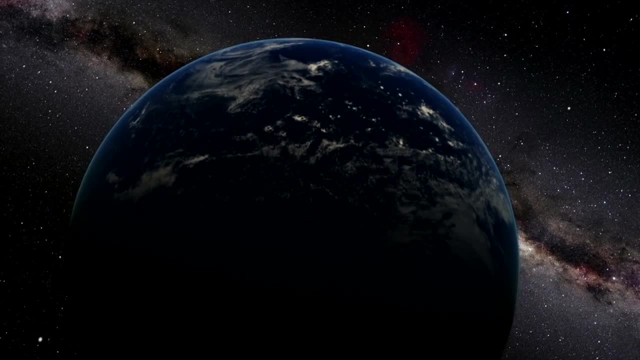 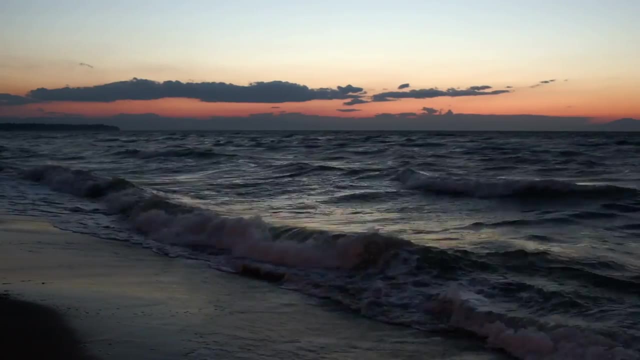 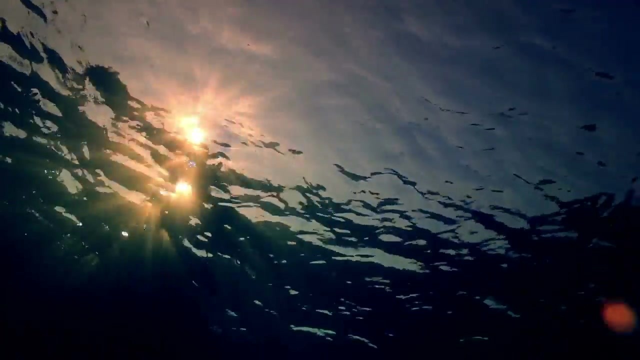 case. The young crust of ocean basins preserves one of the clearest histories of continental movement through time. Oceanic crust is produced at mid-ocean ridges like the one in the centre of the Atlantic, adding incrementally to the gigantic slabs either side at a pace of 2.5. 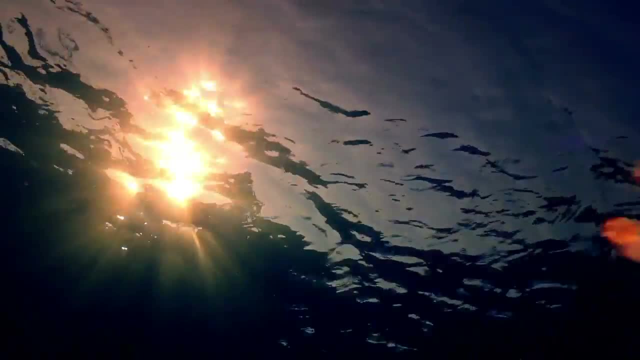 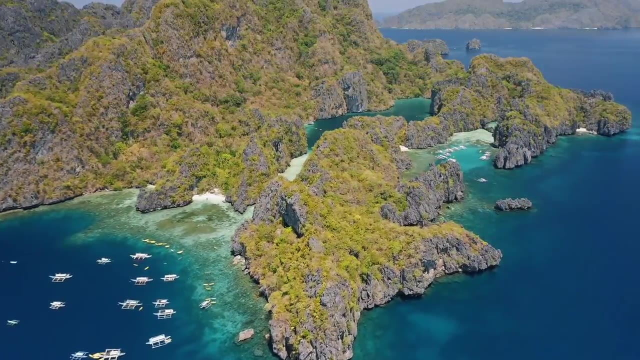 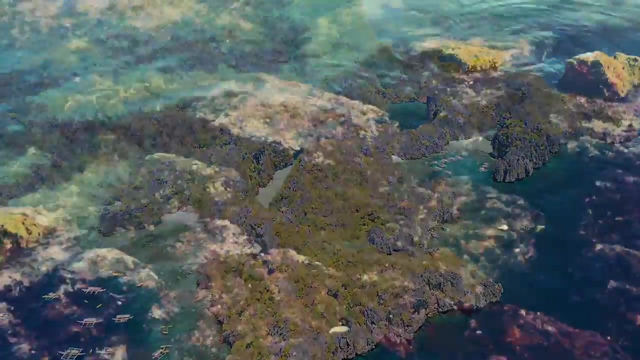 centimetres per year. That's roughly the same speed as our fingernails grow. The great continents attached to these slabs are shifted by the same amount. So by reversing this oceanic conveyor, we can travel back through time. 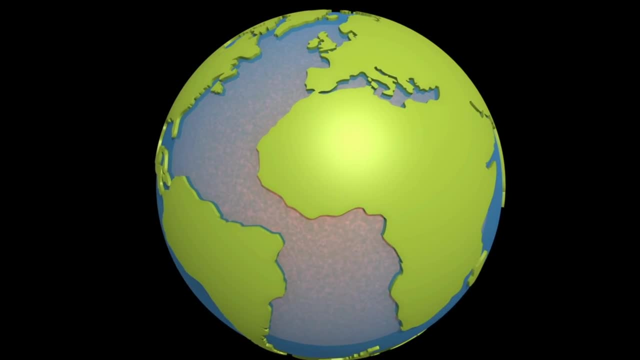 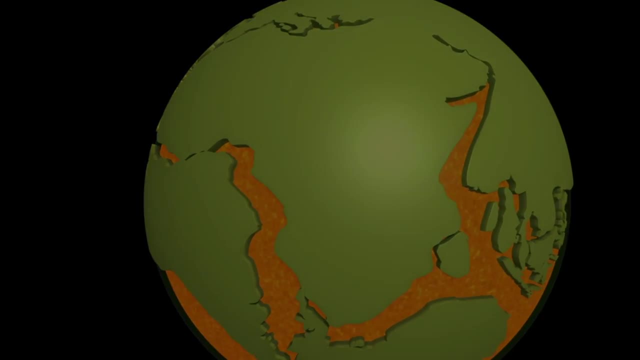 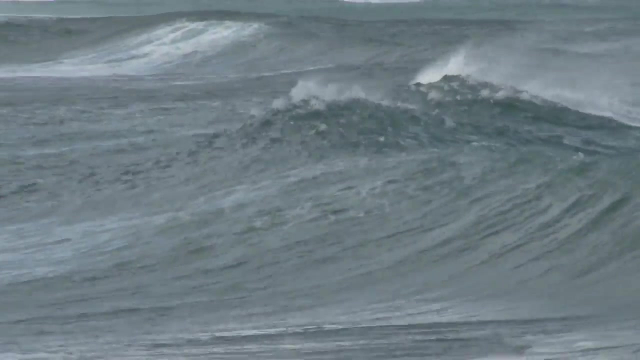 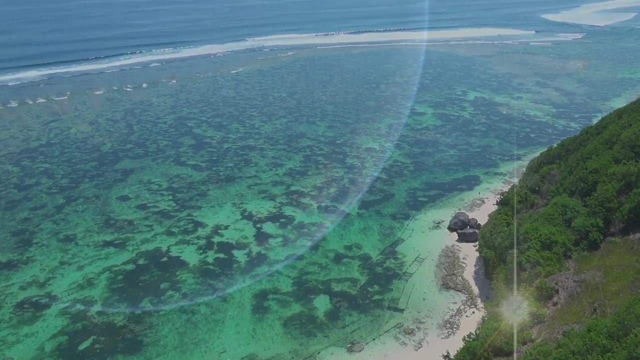 And close the Atlantic, reuniting Europe and Africa with the Americas. Other ocean basins aren't always so easy to interpret. Geologists turn to the fossil compasses frozen in these rocks to reconstruct the time and direction of movement As our magnetic field has periodically flip-flopped, swapping north and south magnetic poles every. 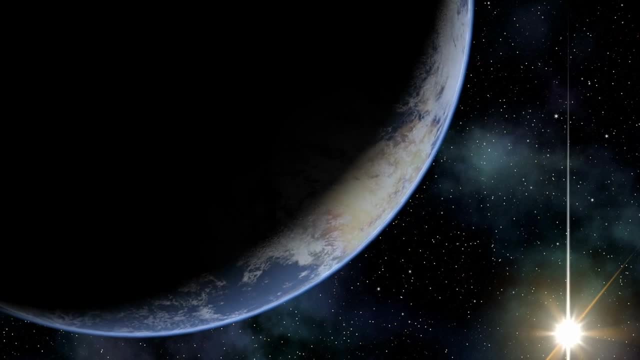 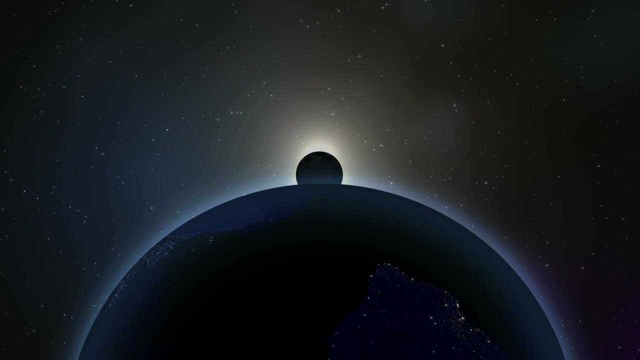 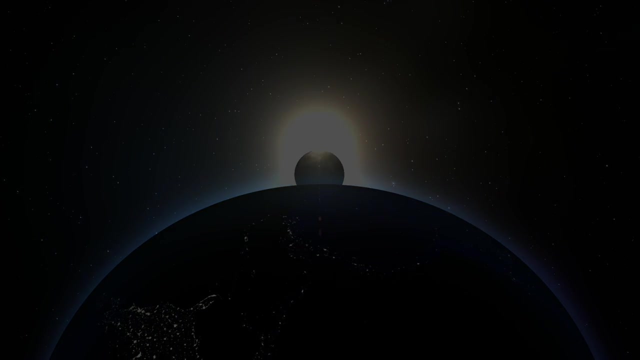 few million years. the reversals are recorded in the new crust that forms. Stripes of magnetic anomalies are etched invisibly into the crust like data on an old videotape. Once again, we can play that tale And watch the continents dance. 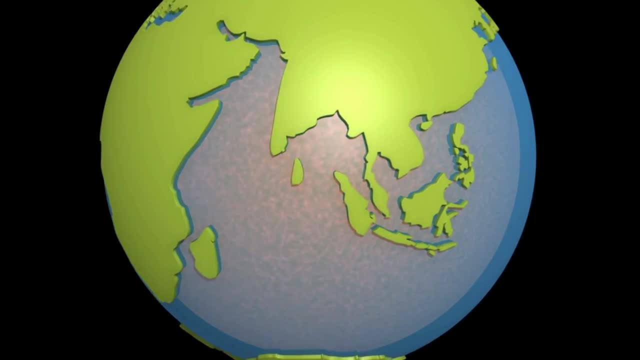 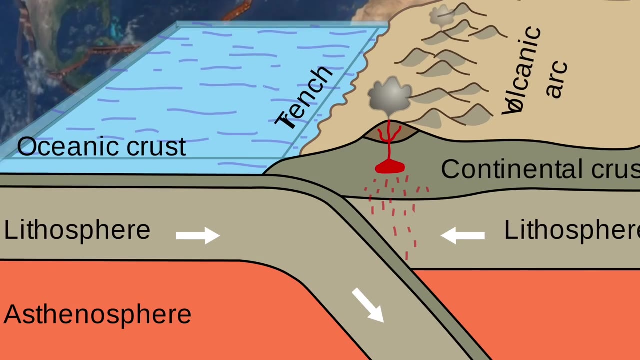 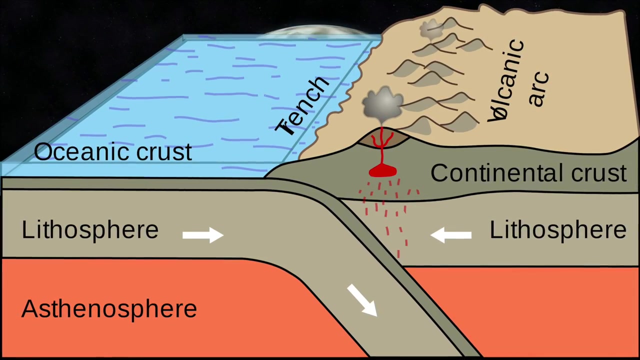 But ocean basins can only help us so far. Unlike continental crusts, oceanic slabs are easily sacrificed to the mantle when two plates clash, and the constant production in one place on the globe inevitably means constant destruction elsewhere. The oldest ocean crust, 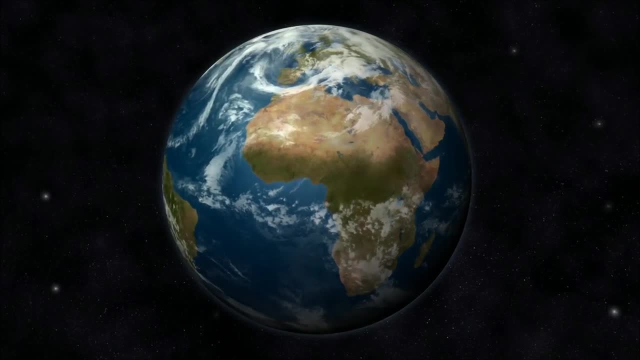 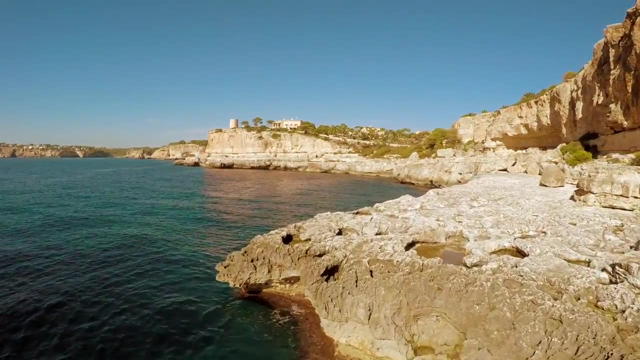 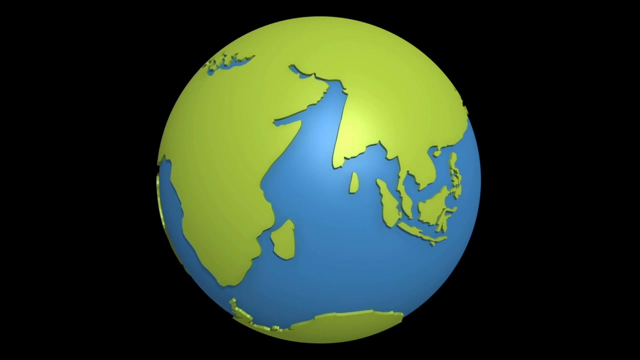 that survives today is just 300 years old. The current ocean has 340 million years old. in the Mediterranean Sea That means there is still some three billion years of continental movement that we cannot hope to know from basins alone. For that geologists must turn to the continents themselves. The land masses preserve a history. 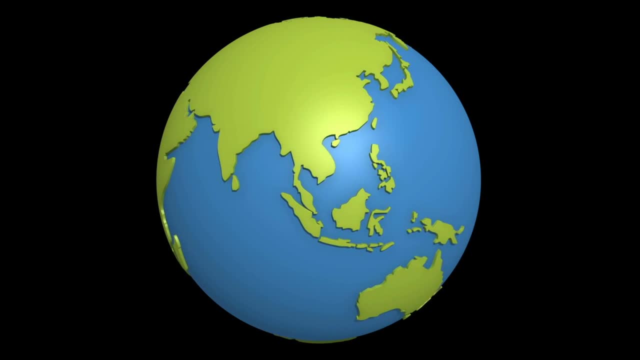 of where the rocks have travelled, as well as the trials they have faced through the years. The volcanic rock is one of the most important rock formations in the world. It's the oldest out of all the other rock species. The volcanic rock is the largest rock in the world, The 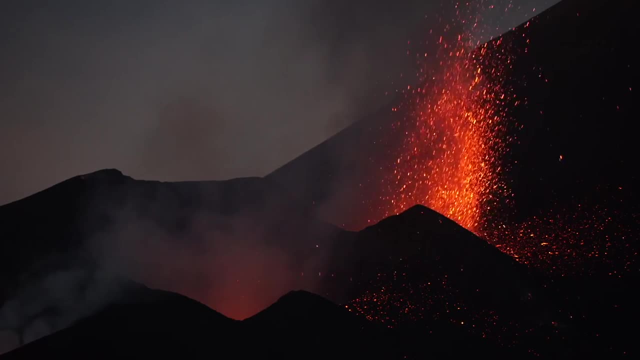 largest rock in the world. The only rock in the world is the most important rock in the. The rocks that preserve fossil compasses are rare on the continents and not regular enough to preserve the periodic reversals, but they can still be used to pinpoint the magnetic. 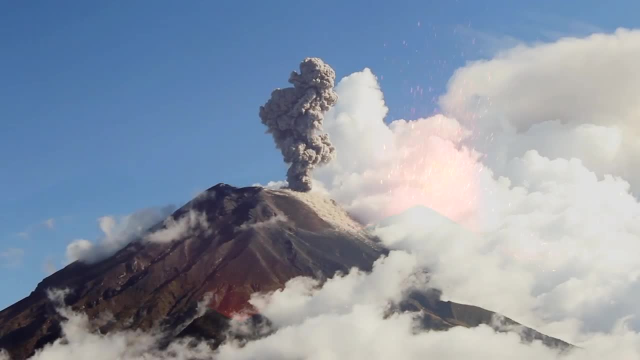 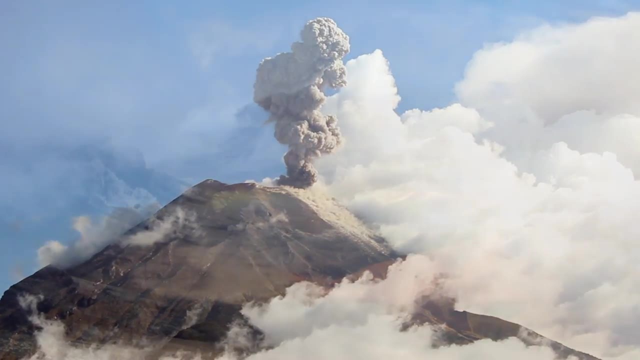 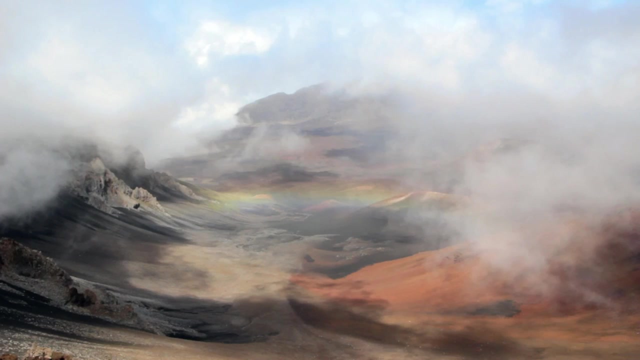 pole at the time of rock formation. If that rock has since rotated or moved east or west, then its fossil compass will be misaligned, Moving the rock and its associated landmass back. we can plot that continent's position at the moment. the rock formed. 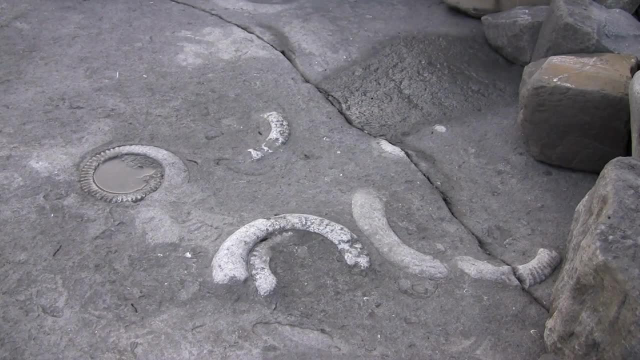 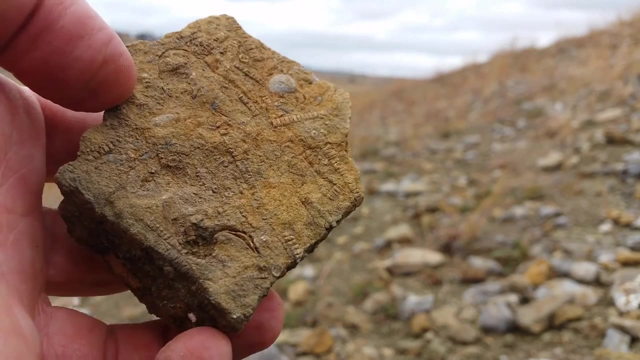 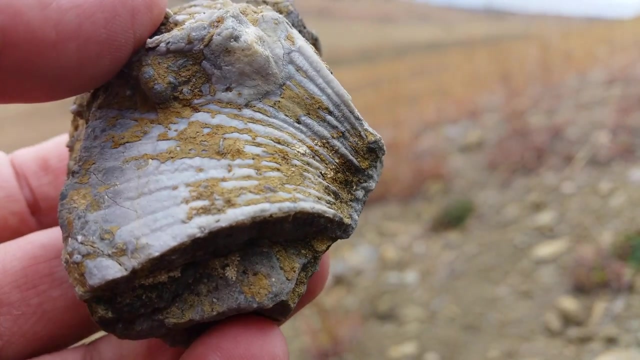 And more traditional fossils offer a straightforward reconstruction of continental juxtaposition. If fossils of the same organism are found on now-separated continents, we can assume that these landmasses were once connected somehow. By plotting the paleogeography of entire fossil communities, paleontologists can reconstruct. 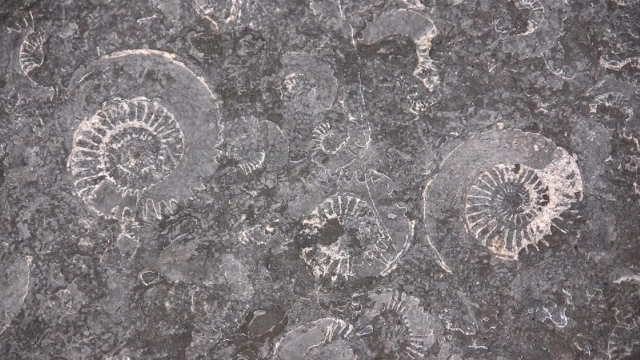 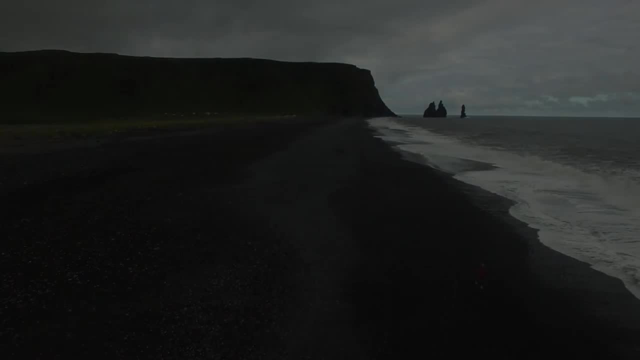 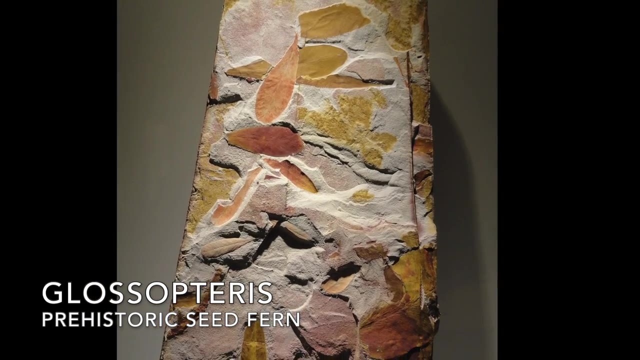 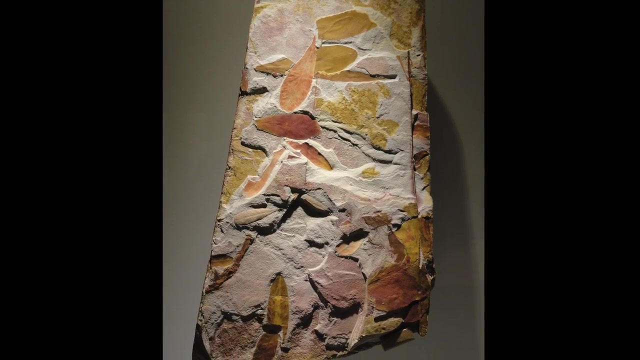 not only the ancient continental configurations, but also the locations of these landmasses on the Earth. 300 million year old fossils of Gosopteris, a tall woody shrub with tongue-shaped leaves, are found in Antarctica, India, Australia, South Africa and South America. 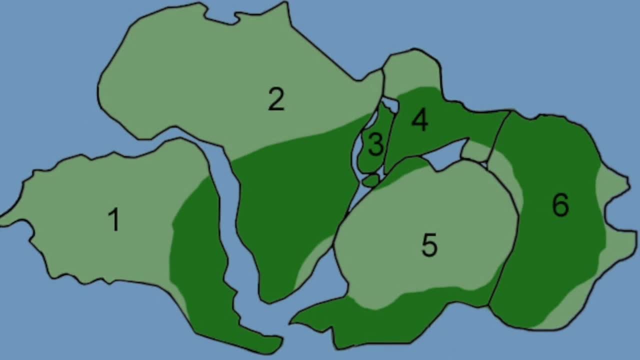 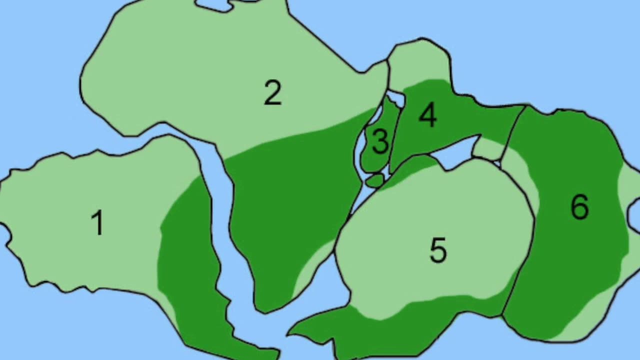 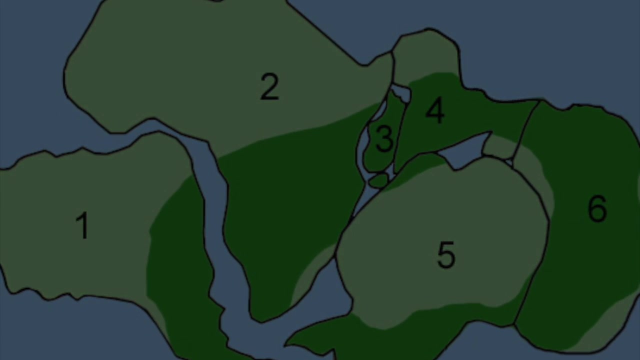 Their distribution suggests that not only were these now-disparate landmasses once united, but that the resulting supercontinent must have sat at temperate or tropical latitudes where the wet, swampy conditions the plant preferred could dominate The distribution of lemur-like animals across Africa, Madagascar and India. today is not. 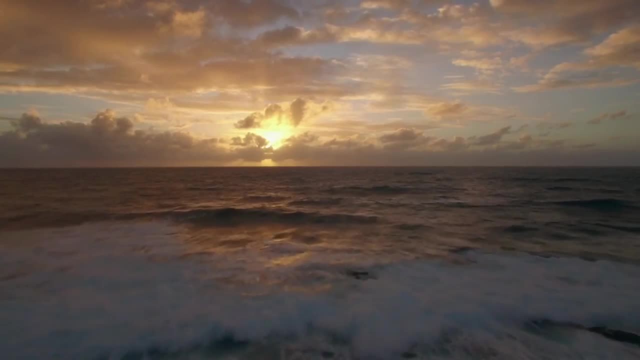 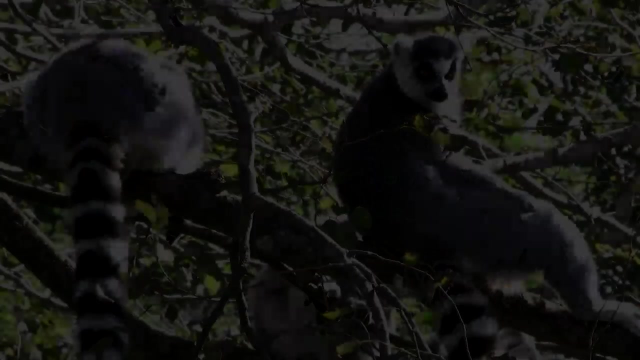 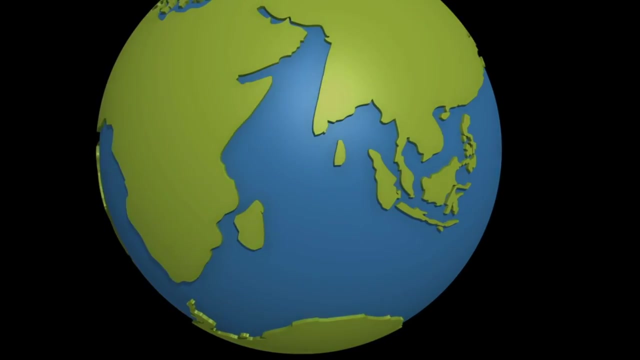 due to the sunken land bridge of Lemuria, but rather a sign that the three were once joined and have since been rent apart by lateral plate-technology. Other clues in the surviving continents are harder to decode, but offer a window into the moments of continental collision and separation. 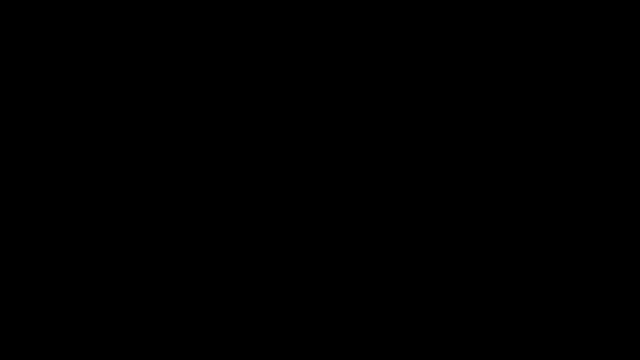 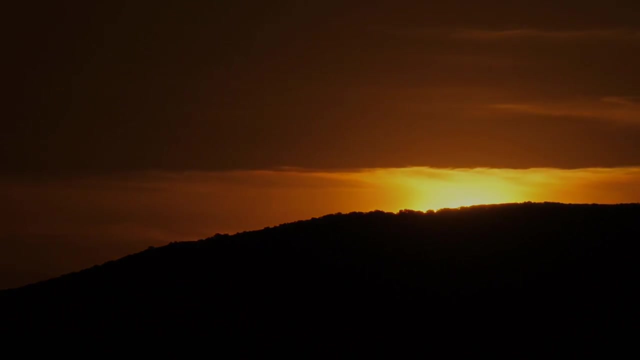 Kingsley, Cosgrove, Hardy troopers. When two buoyant landmasses collide and neither is willing to succumb to subduction, the rocks crack, crumple, compress and eventually come to rest shade of hundreds deep in the ocean. sudden警ar. 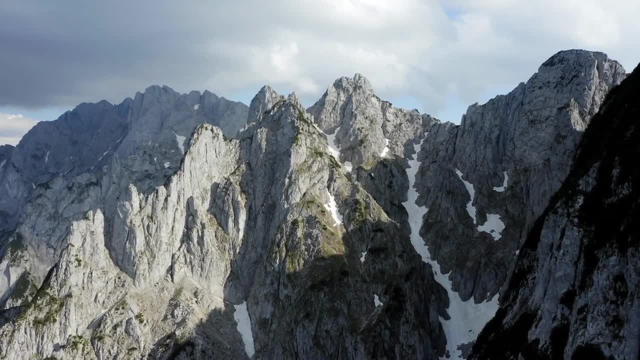 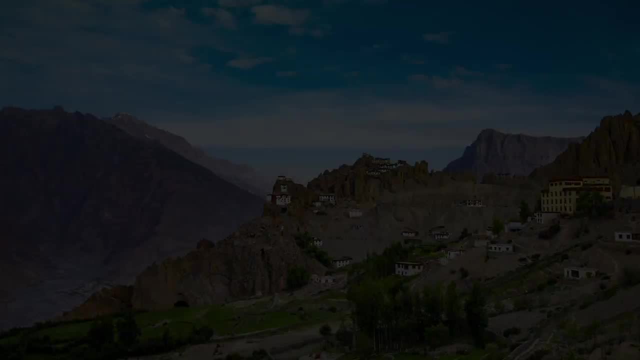 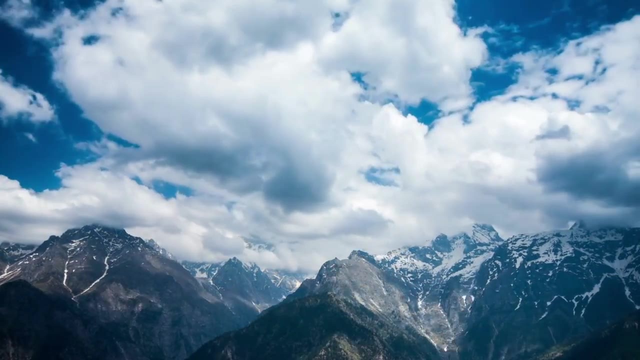 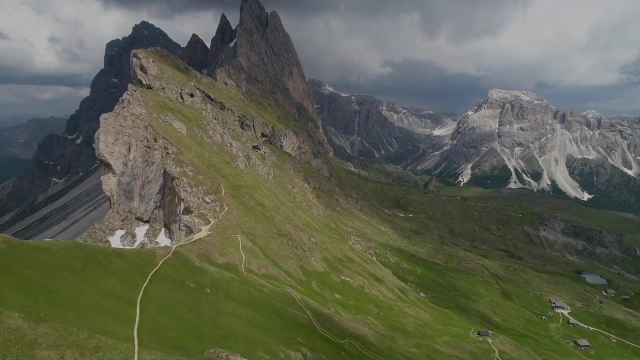 Shake-ünder can reach many miles higher than surrounding landscape, like the Himalayan Range and Tibetan Plateau today, and the rocks formed at their hearts preserve the tortured scars of the collision that formed them And over millions of years, even the tallest mountain eventually succumbs to erosion, and the hearts of 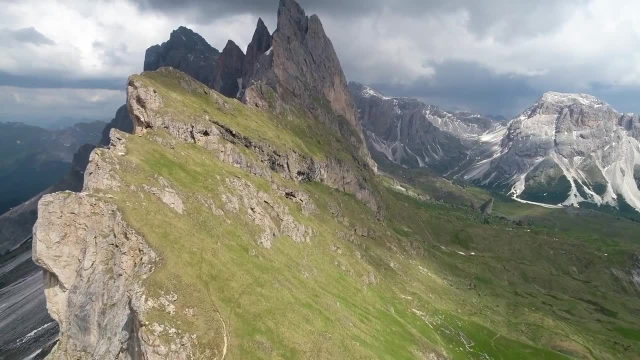 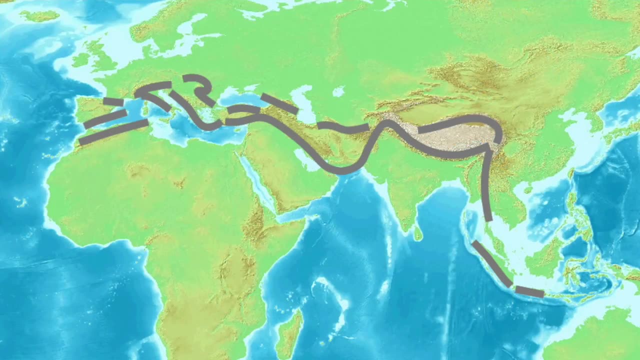 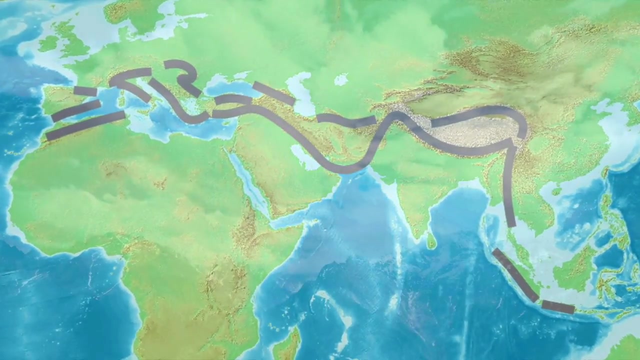 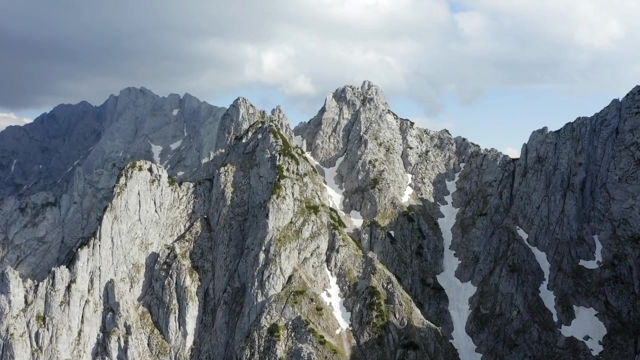 these ancient ranges are exposed at the surface. They are known as orogenic belts. Using these warped rocks to reconstruct mountain-building events many hundreds of millions of years in the past is not straightforward, But doing so reveals precisely which continental slabs collided, and when. Yet 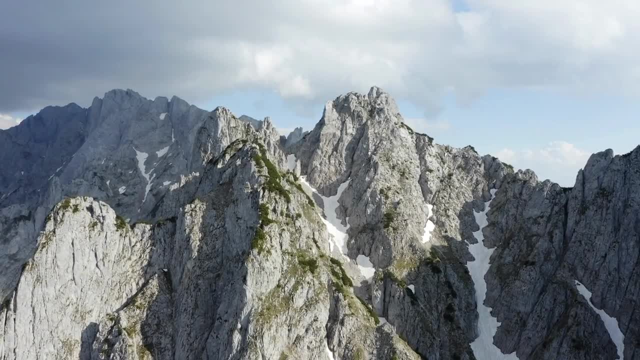 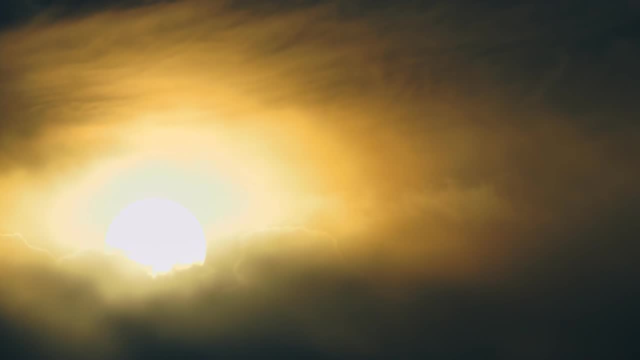 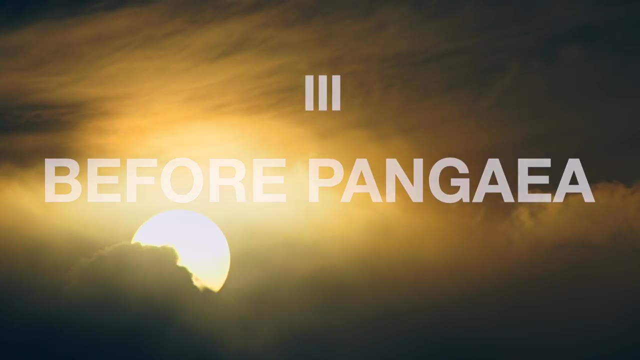 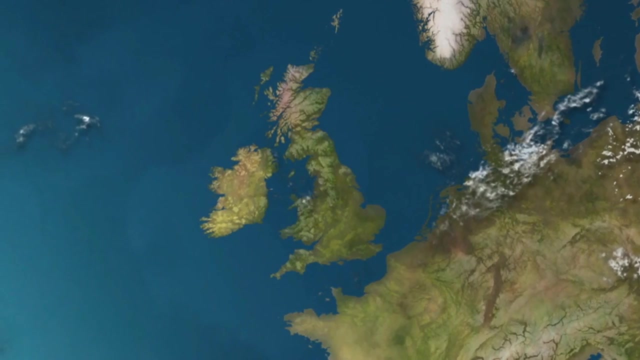 even if we don't fully know the origin of these rocks, we know that they are still there. We know why. We now have a clearer picture than ever of our planet's checkered supercontinental past. Scotland and England are now as one, fused together at the northern edge of 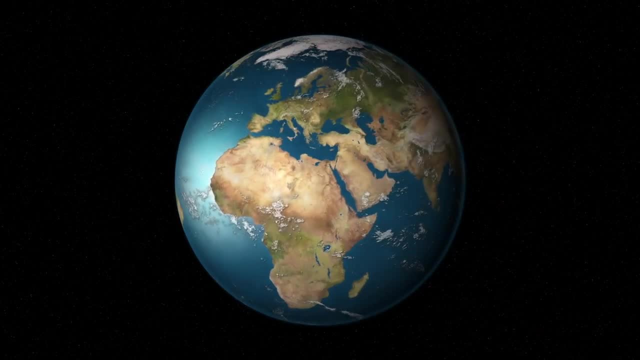 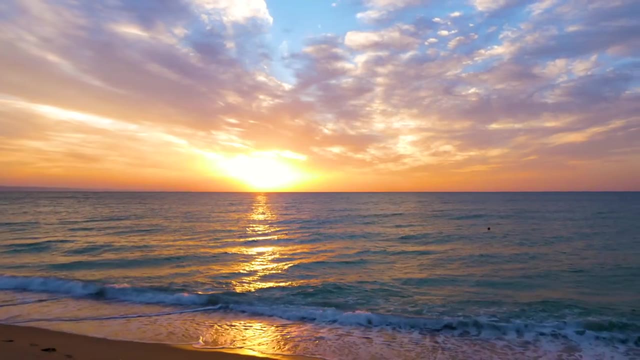 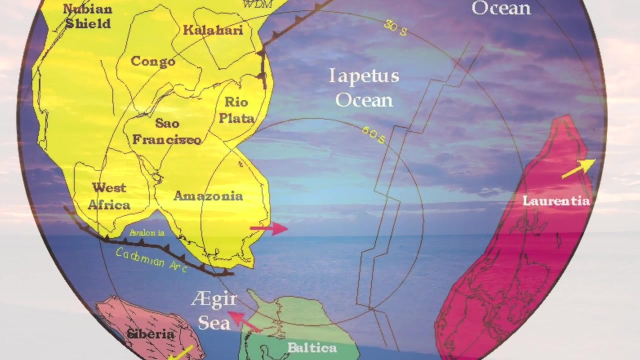 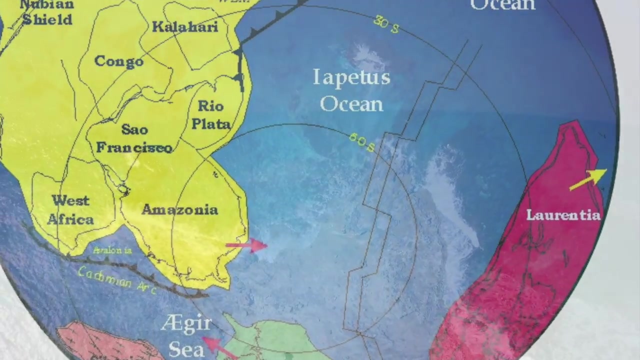 the Eurasian continent, But this was not always the case. 500 million years ago they were separated by a great ocean, the Iapetus. But plate tectonics is ever fickle and driven by the unpredictable flows of the upper. 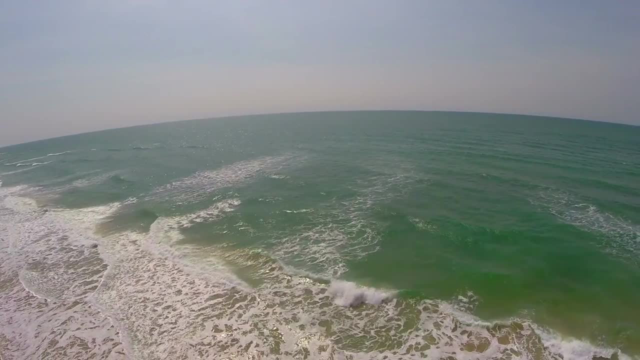 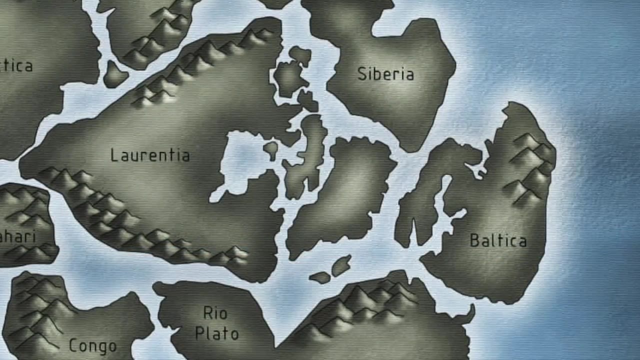 mantle. gradually, the Iapetus Ocean Basin began to close. The continent of Laurentia, along with the Scottish homeland, bore down and the ocean was torn apart. The Iapetus Ocean Basin was torn down upon Baltica and what was to become England. 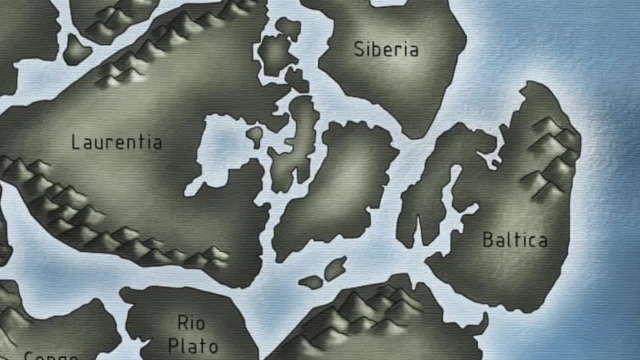 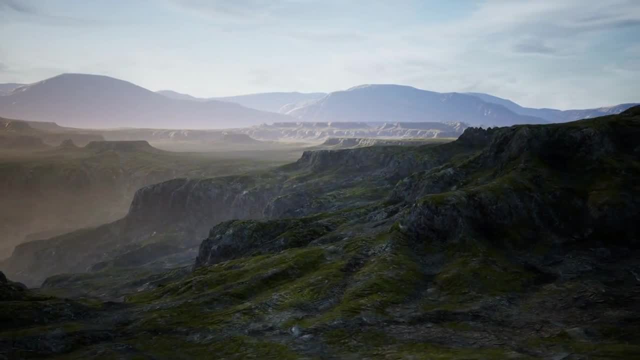 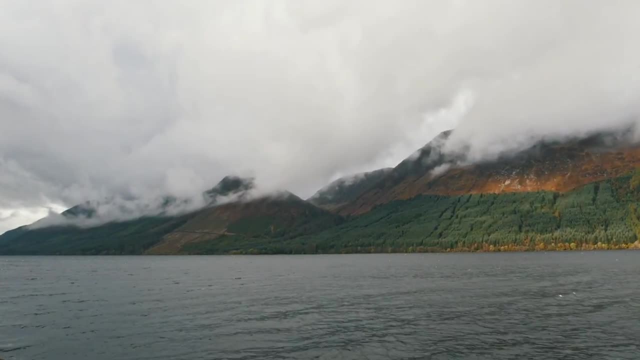 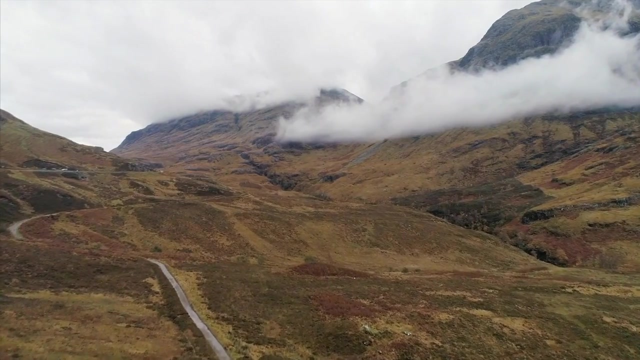 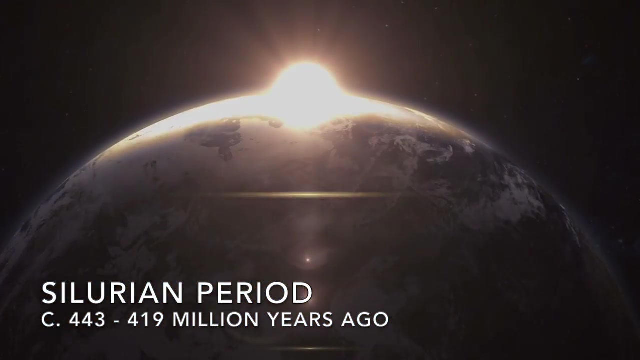 When all of the ocean basin was gone, the two Leviathan continents crashed into one another, building mountains in an event known as the Caledonian Orogeny and fusing the Laurentian and Baltican continents together forever By. 420 million years ago, in the Silurian period, when life had barely made it onto the land, the Iapetus Ocean was no more. 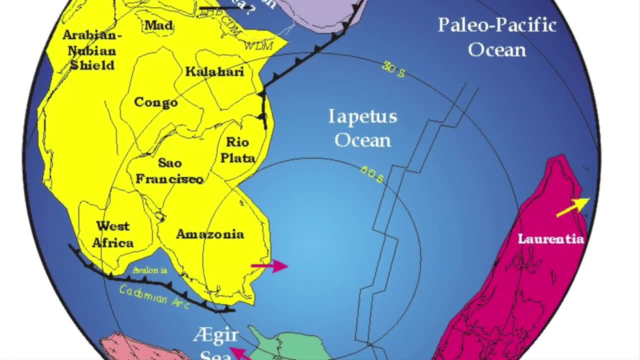 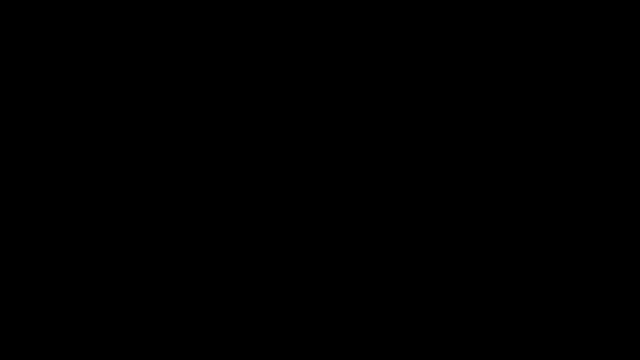 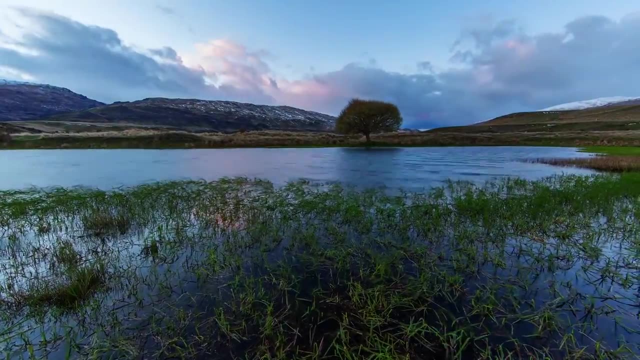 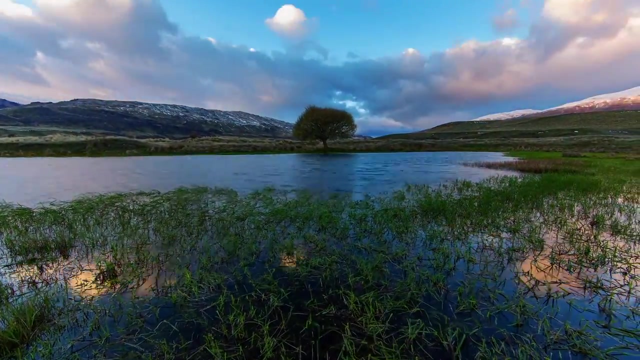 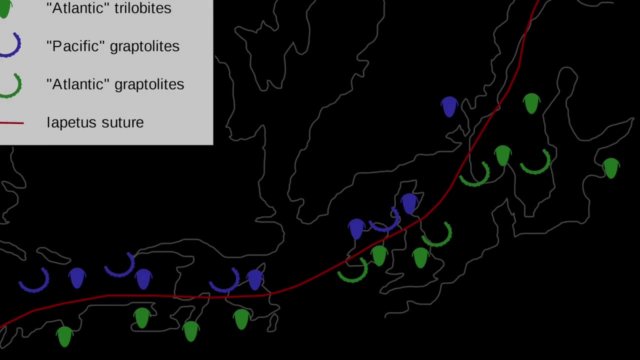 And all that remained was the twisted crash site of two continents forced unforgivingly together. That crumpled mountain range has since eroded, But geologists can still trace the tortured scars across the British landscape. The Iapetus Suture Zone runs from the Solway Firth to Lindisfarne, uncannily close to the modern Scottish border. 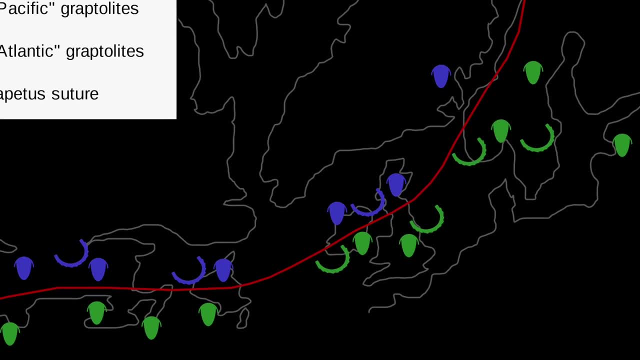 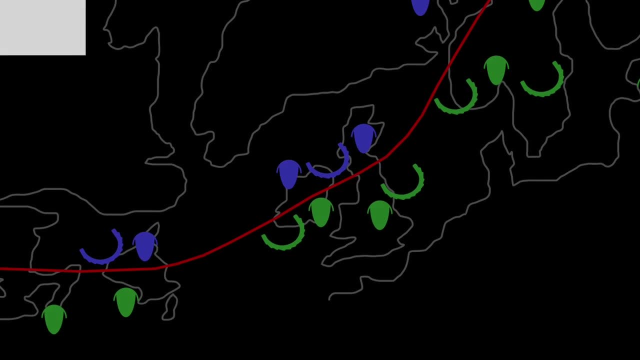 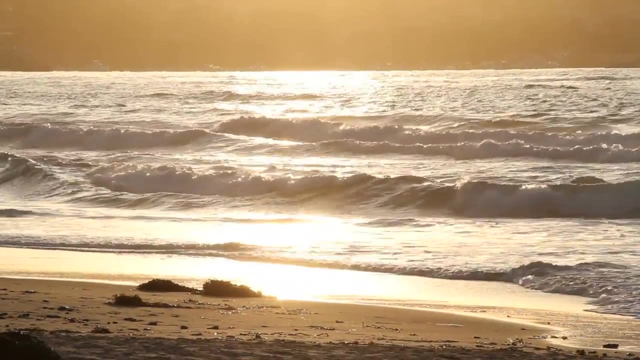 The Iapetus Suture is just one of the scars left behind in ancient continental crust. There are collision zones like it all over the world, but as we probe further back in time, crustal clues that have escaped erosion become increasingly hard to find. 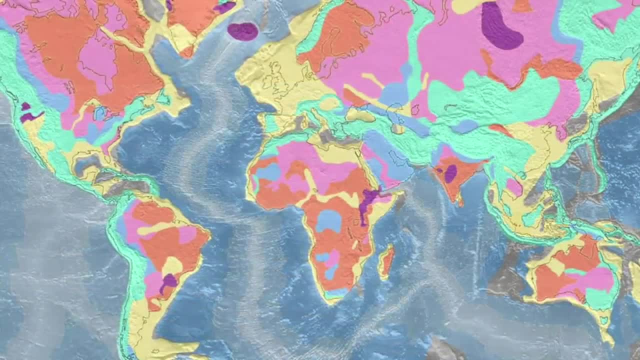 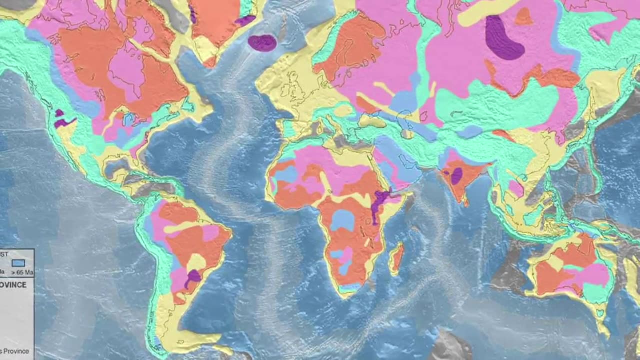 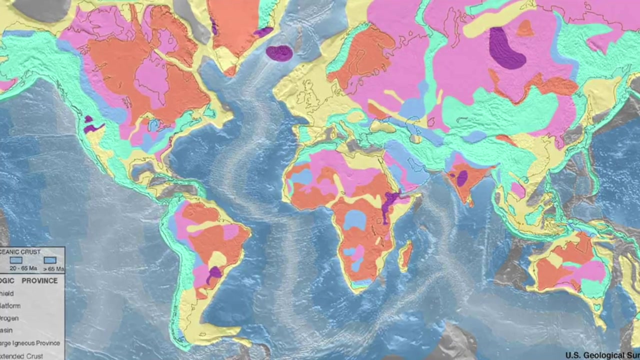 Certain of the oldest remnants of continents called Cratons can be found in Canada, Australia, South Africa and elsewhere today, But there are tantalising hints that in their earliest days they were united into one or a series of Archaean supercontinents. 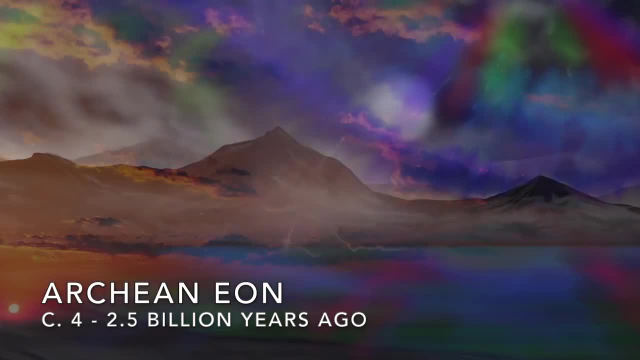 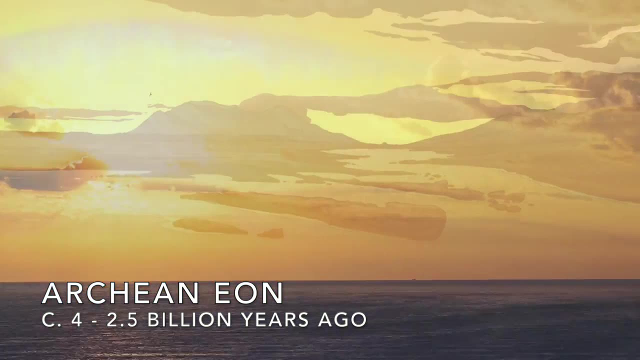 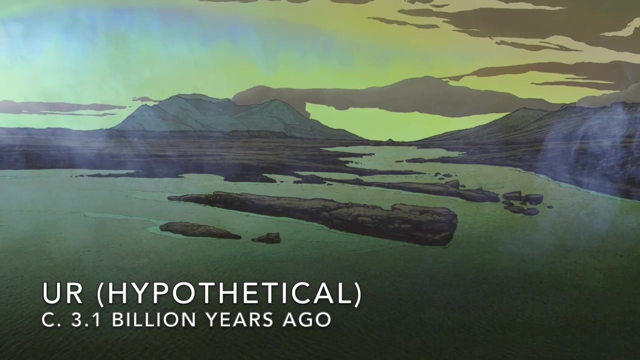 Archaean Supercontinent 했는데. The Perilla Reconstruction Construction extends the record of supercontinents almost back to the first continental masses of all. A single early supercontinent, Ur, has been proposed based on the observation that all of the cratons dating to 3 billion years ago were clustered together at a later time. so 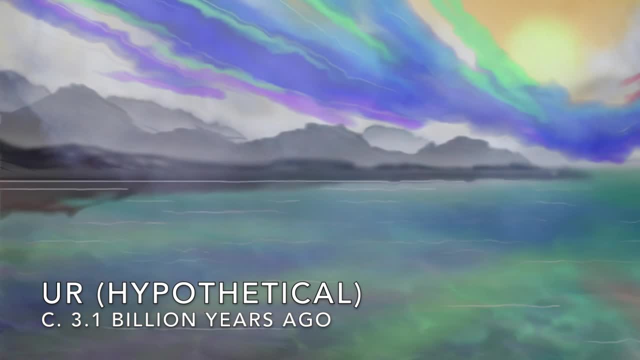 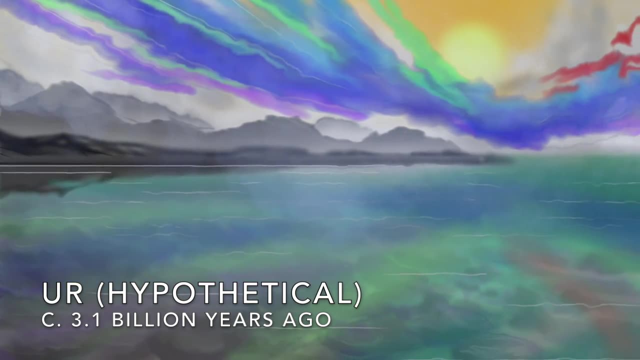 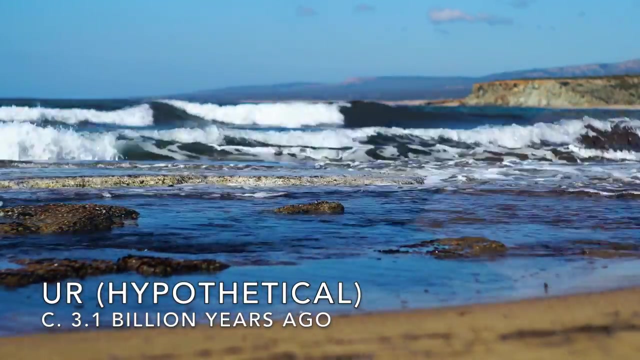 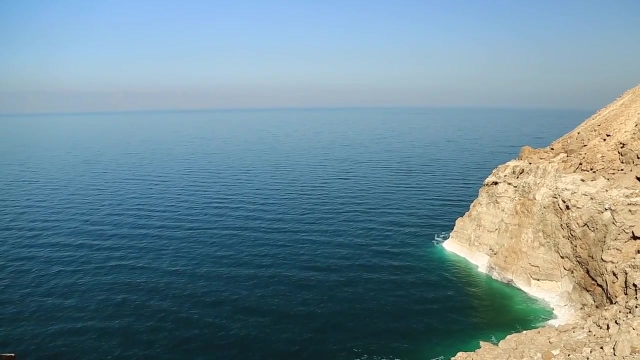 are likely to have formed and stayed together since their earliest moments. But with such ancient rocks, few other clues remain that could hint at the configuration or position of Ur, and its very existence relies on a great number of assumptions. Instead, a more conservative reassembly suggests that the ancient cratons were incorporated. 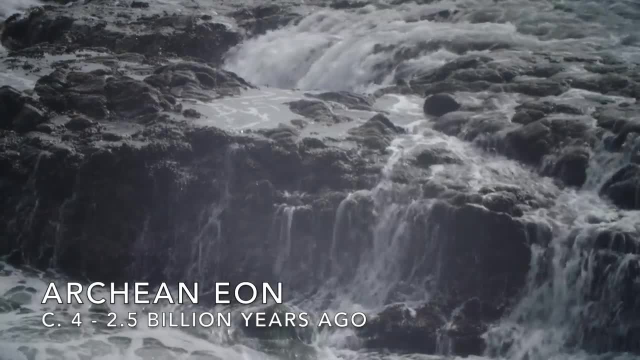 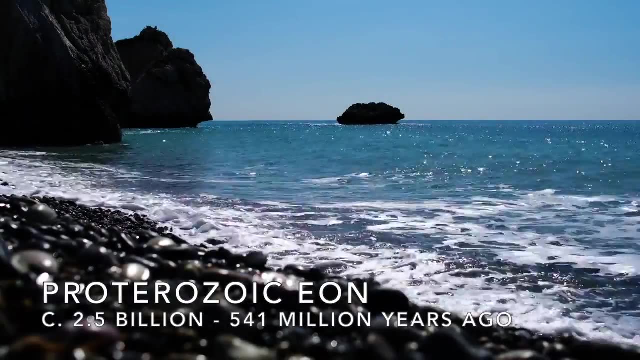 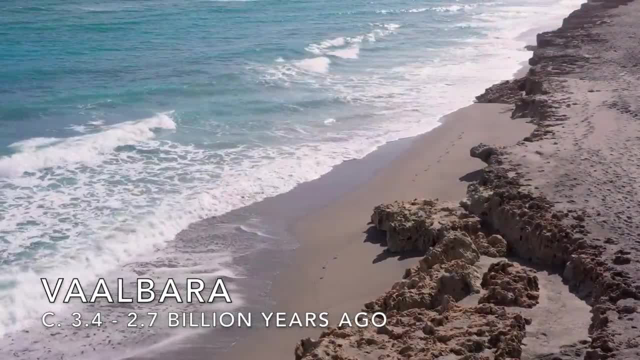 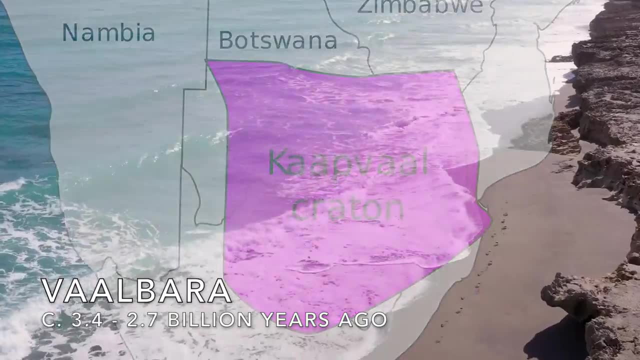 The first was Valboa, The second was Pilbara, which reigned from around 3.4 to 2.7 billion years ago and combined the Kapval Craton now found in South Africa and the Pilbara Craton of Australia. 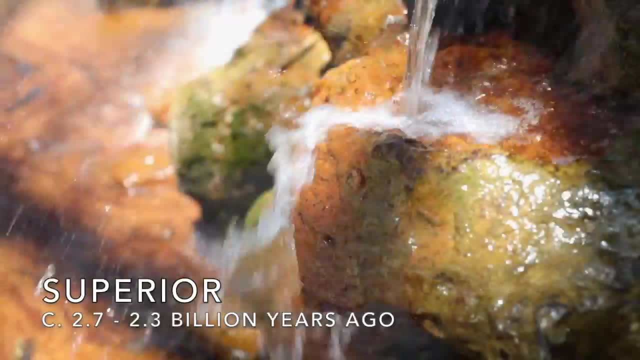 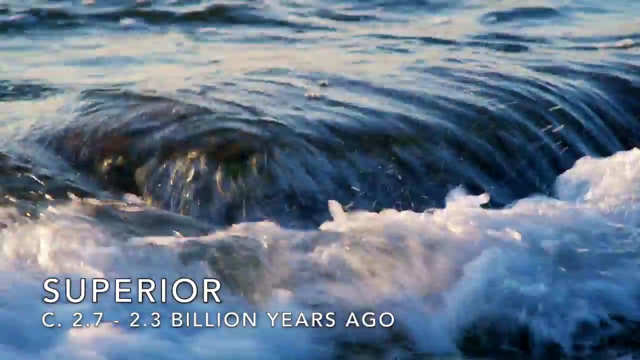 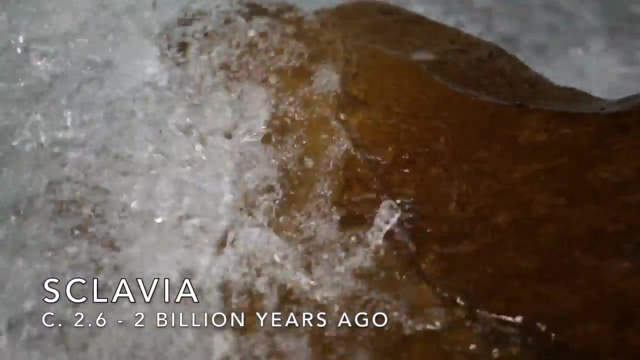 Next came the continent known as Superior, which existed from 2.7 to 2.3 billion years ago and of which only the Canadian Superior Craton survives today. At the same time, the Slavia continent, including the modern Canadian Slave Craton, reigned from. 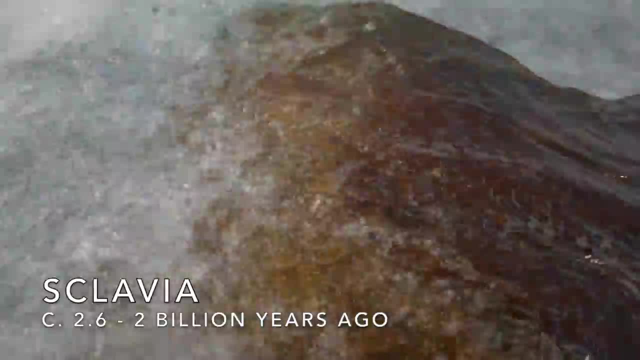 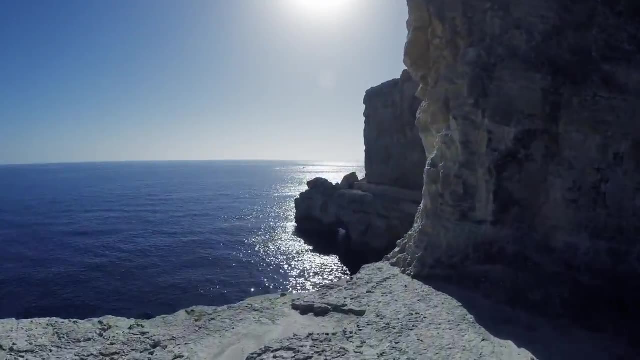 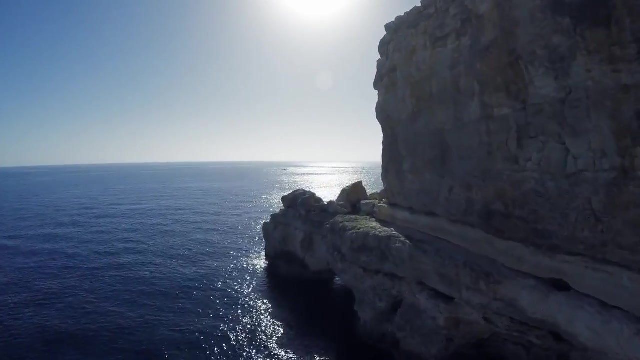 2.6 to roughly 2 billion years ago. These reconstructions are based on the scant ancient evidence available from these and other crustal blocks, including the pulses in zircon creation that are consistent with their assembly, But we have no real evidence. 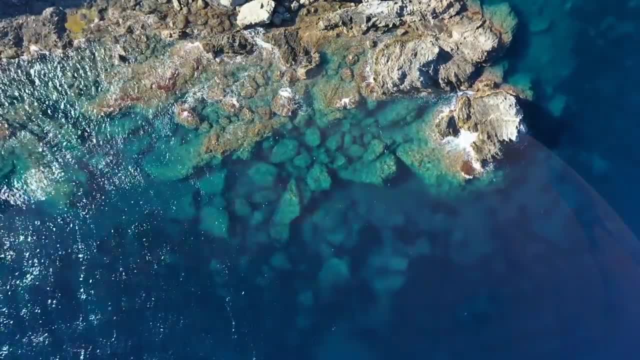 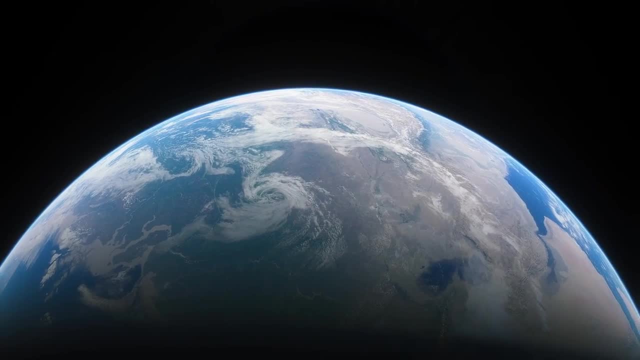 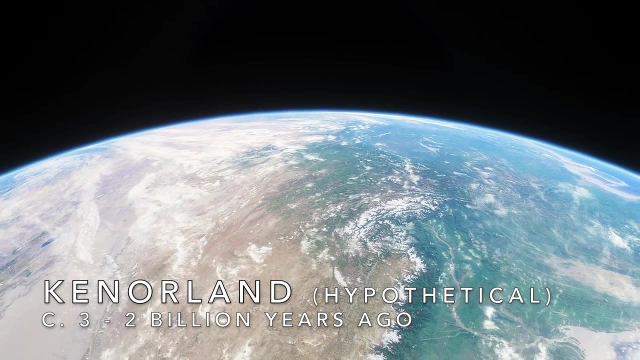 There is no real way of knowing where they existed on the surface of the Earth. Some have even suggested that they were all united as far-separated parts of a single, long-lived supercontinent called Kenorland, whose central regions have since been lost to time. 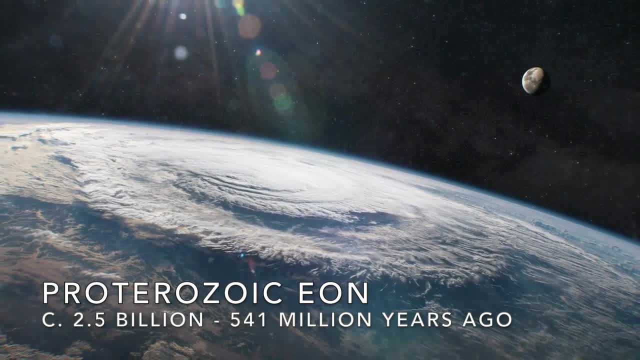 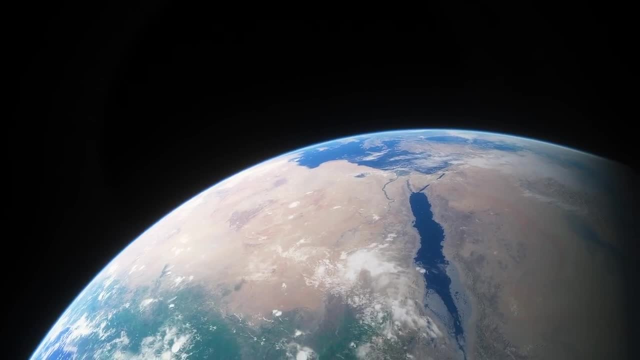 If we could speed the geological clock from the early Protozoic to today, we would be able to see the Continental Dome. This is aogrion of a rock whose crater is never sharp. It is considered a symbol of the age of the earth. 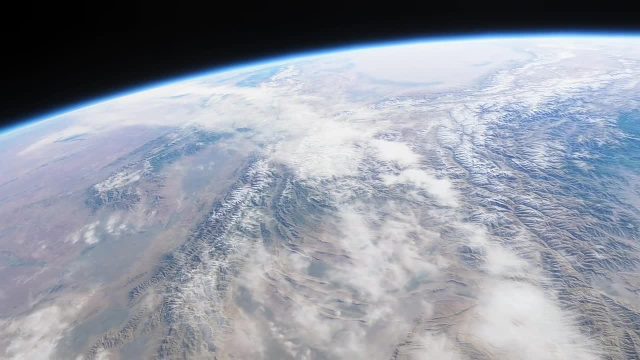 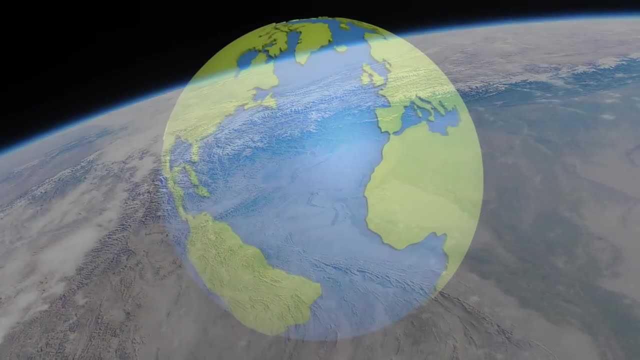 The emerald at the core of the rock is marked with the yellow dot on the rock. The red dot on the rock represents the number of years from which this rock killed 3,000 people. We know that the sea and the oceans coexist as one. 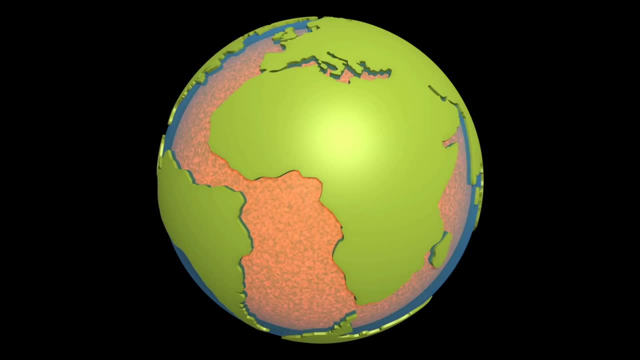 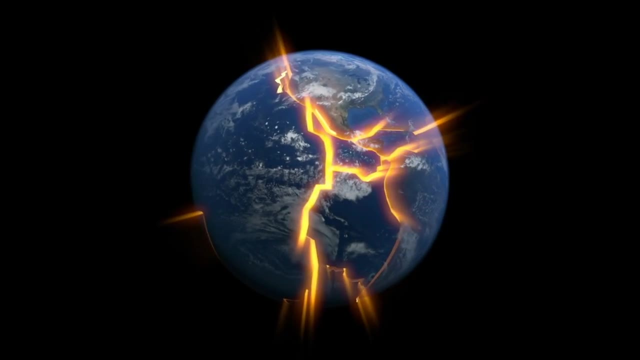 But this is a mystery. The sea is the same as the ocean, which is one of the third largest ecosystems in Земl- That's the right thing to say of supercontinents- and the dance is punctuated by their calm motions before. 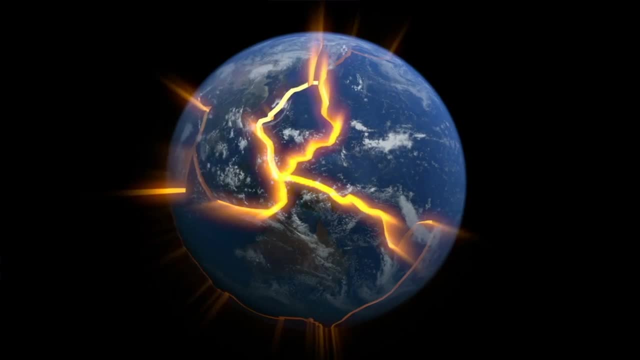 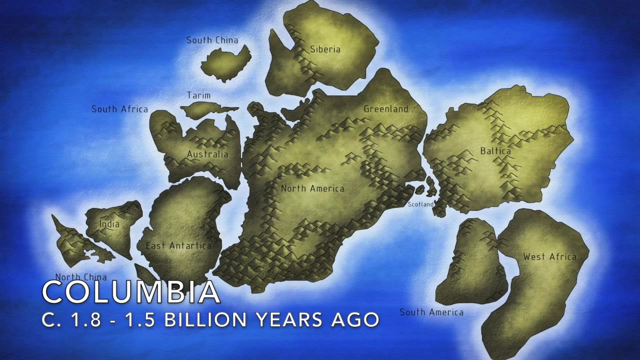 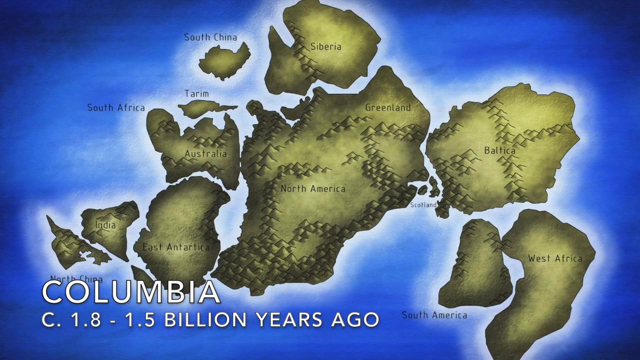 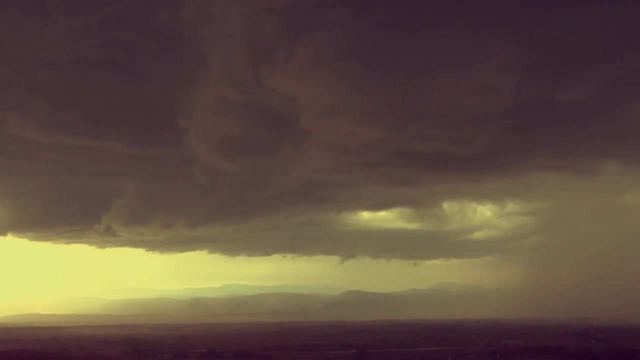 the continents whirled away once more. The supercontinent known as Columbia assembled around 1.8 billion years ago from crustal blocks that would later form parts of North America, Greenland and Europe. It was nearly 13,000 kilometers north to south and likely straddled the equator. 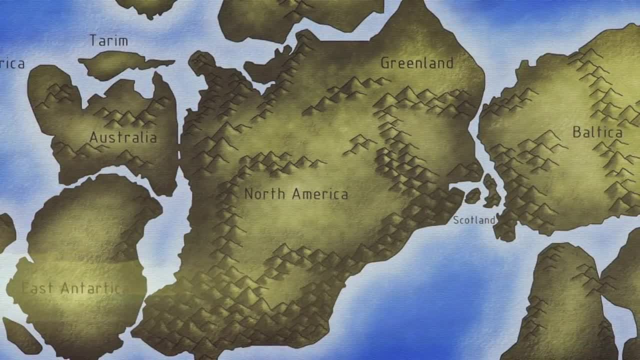 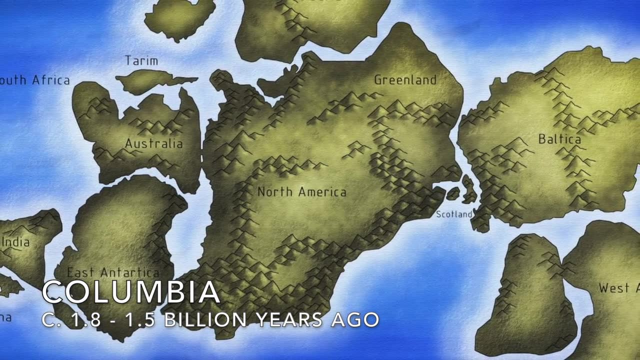 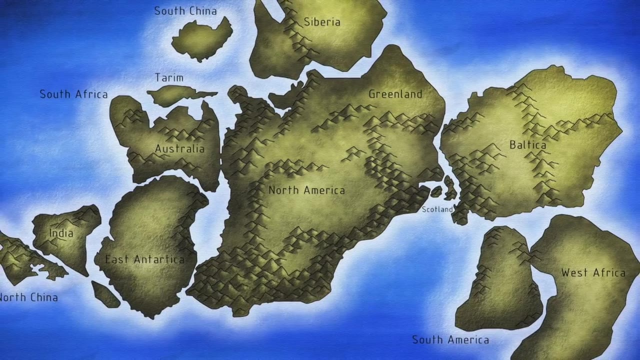 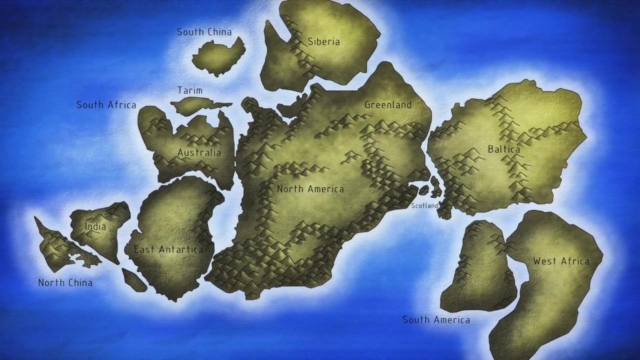 favoring the Northern Hemisphere. Different interpretations of the orogenic belts left behind from that time produce very different reconstructions of these continental fragments. One suggests that pieces of Antarctica and Australia lay along the North American west coast, while an alternative places India in the same position. Geological evidence suggests that the 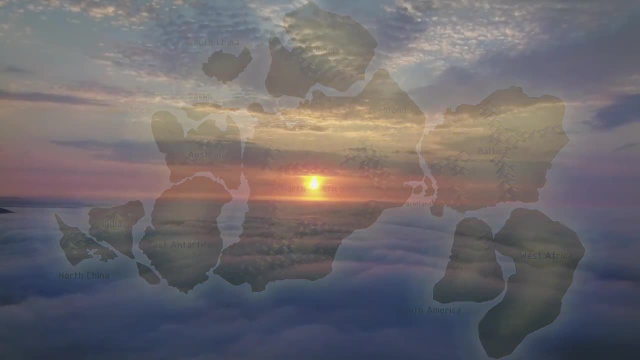 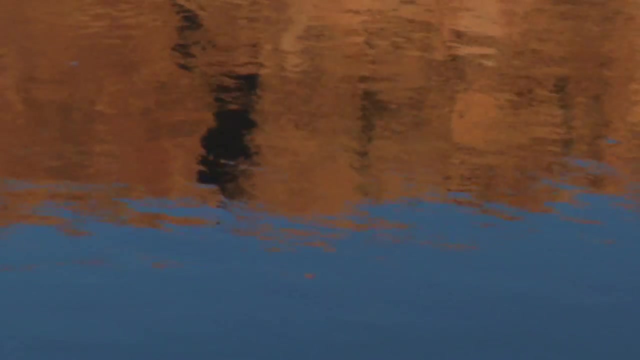 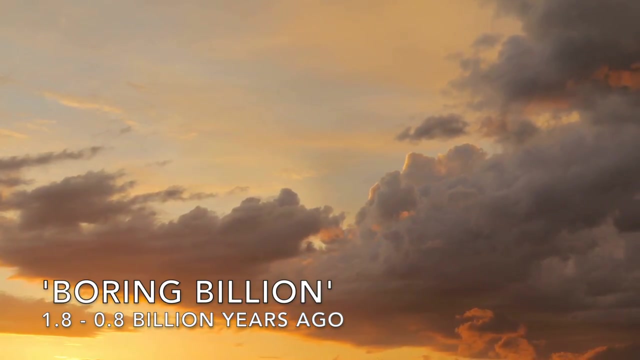 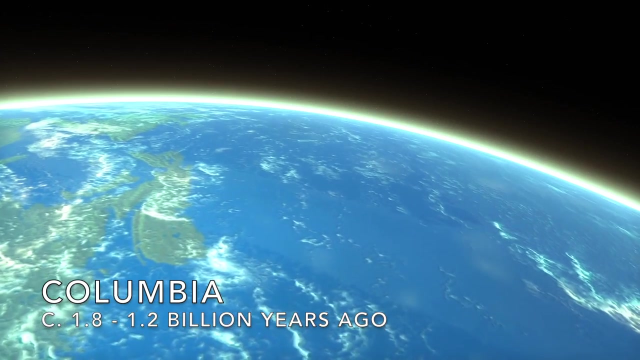 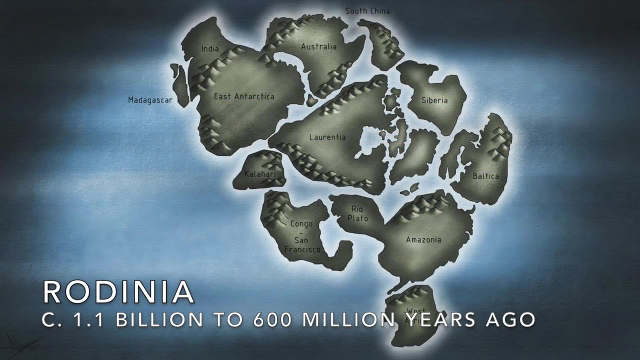 Colombian supercontinent persisted until around a billion years ago, possibly contributing to a period of unprecedented environmental stability, known affectionately as the Boring Billion. At the end of its tenure, new rifts formed and new continents tore away. Next came Rodinia. Proposed timings for Rodinia assembly actually overlapped with. 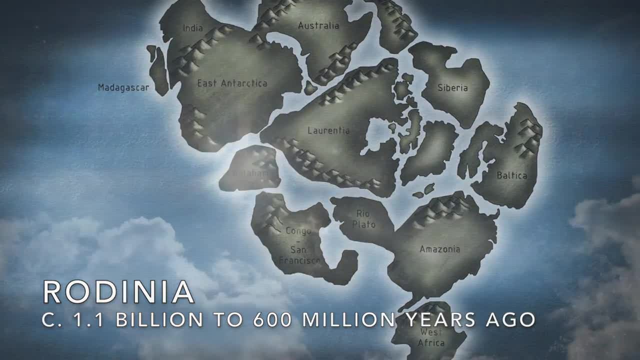 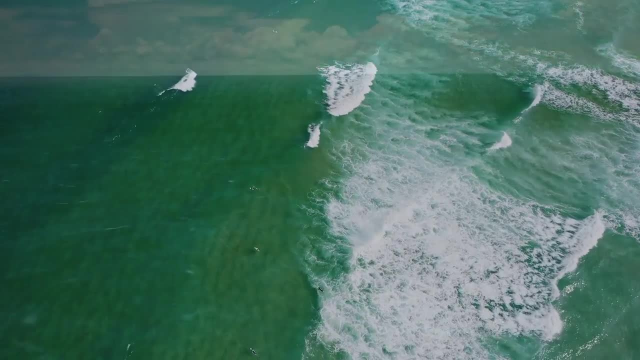 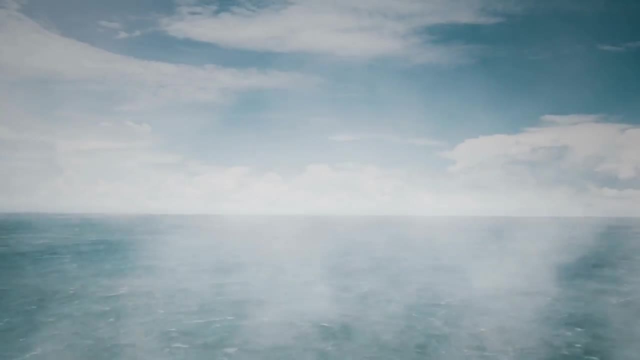 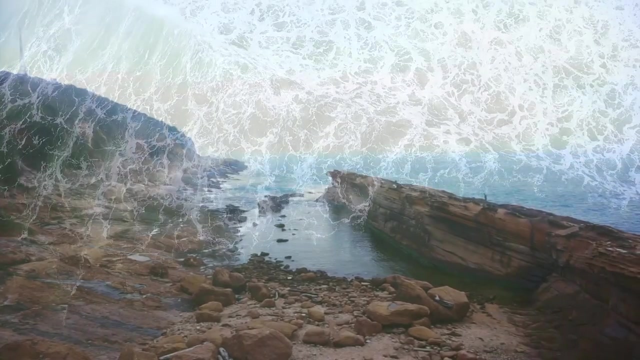 the breakup of Colombia. So it is possible that continents fleeing, one super assembly was soon caught in the grip of another. But as for Colombia before it, reconstructions are notable for their lack of agreement. At this significantly younger age, there are many more rocks available for comparison, but they are still disparate and much altered by 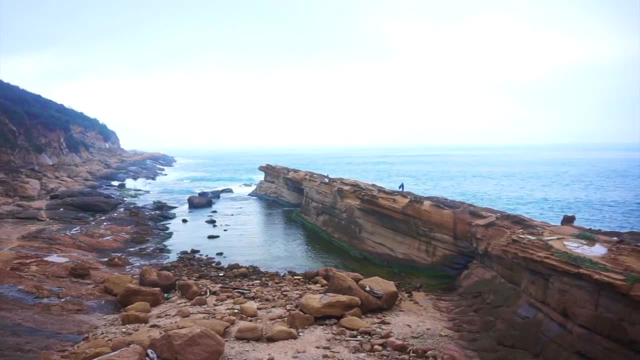 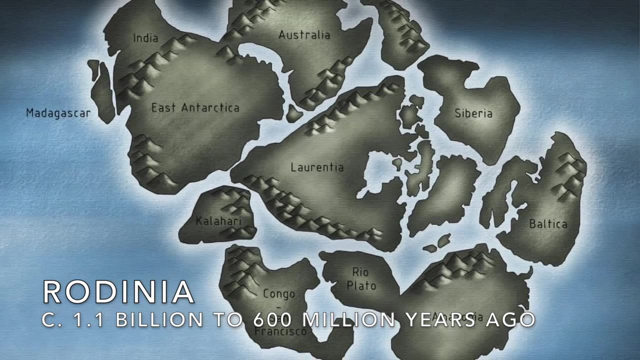 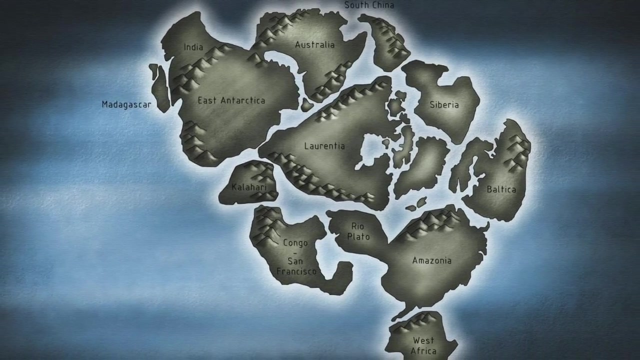 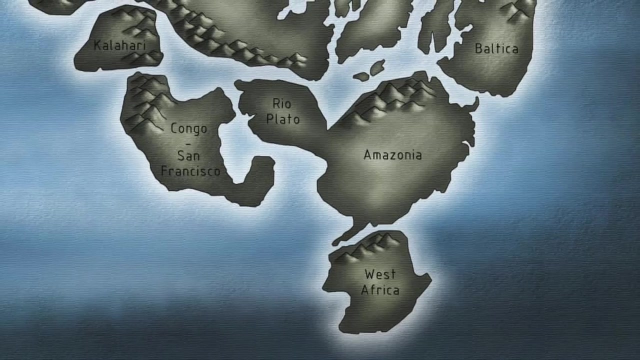 time. Most geologists agree that the North American crustal block known as Laurentia formed the core of Rodinia, with Eastern Europe, Amazonia and West Africa to the southeast, and Australia, India and Antarctica to the northeast. Fragments of crust that now form the eastern part of Brazil are attached to the south. 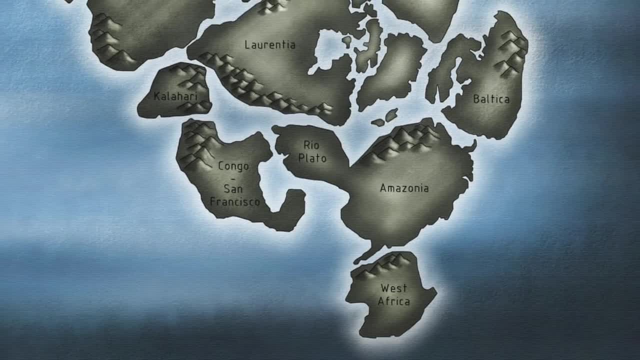 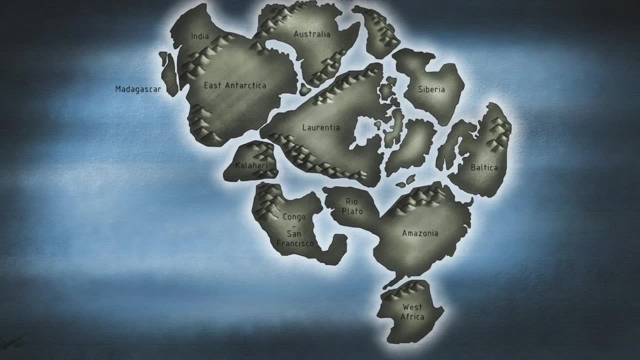 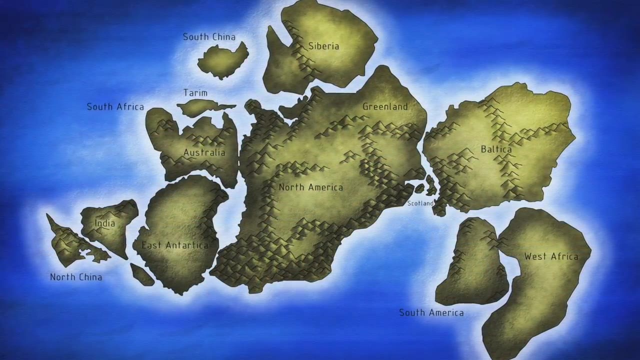 Fragments of crust that now form the eastern part of Brazil are attached to the south, But the positions of ancient portions of China and Siberia are still the subject of debate. To further complicate matters, as well as overlapping with Colombia's breakup, Rodinia assembly may have been concurrent with its own destruction, Like 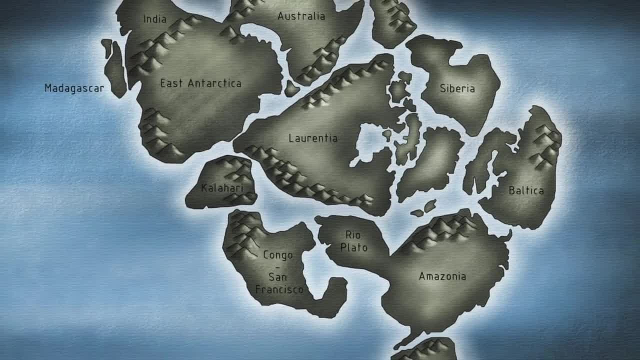 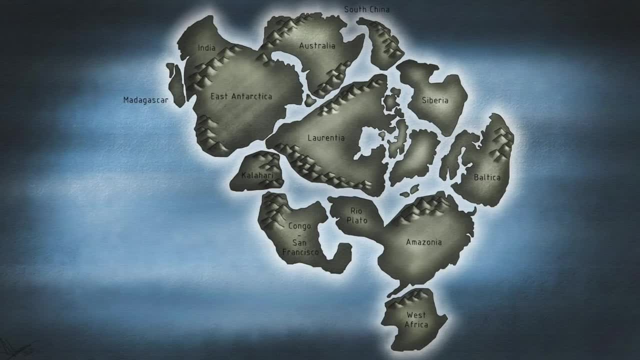 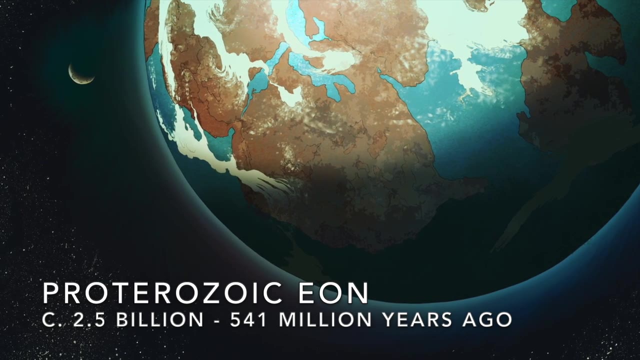 some vast and ponderous Newton's cradle continents crashed into the scrum even as others broke free. The Proterozoic Earth's surface was cluttered with cratons as Rodinia broke up between 850 and 600 million years ago. 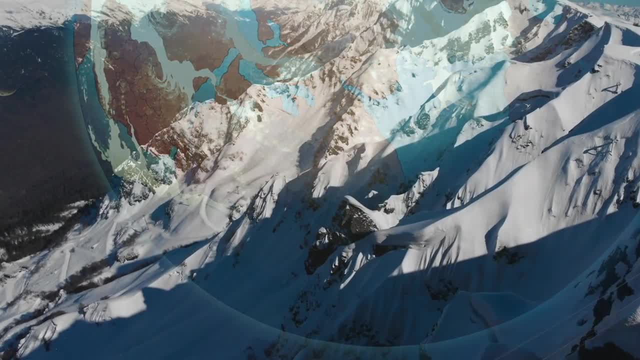 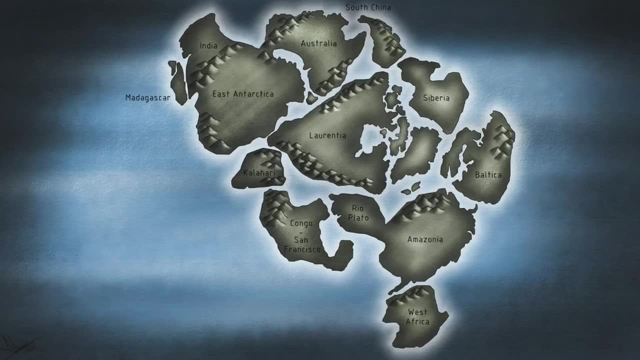 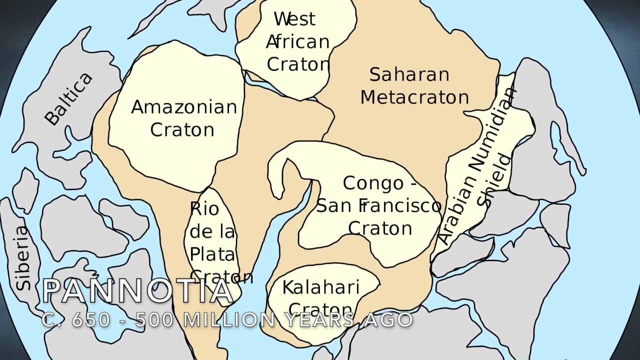 Some passed briefly across the South Pole, colliding as they approached from different directions. as Rodinia turned itself inside out across the globe, The resulting supercontinent Pannotia saw the Congo Craton amalgamated with Laurentia and other Rodinian fragments. 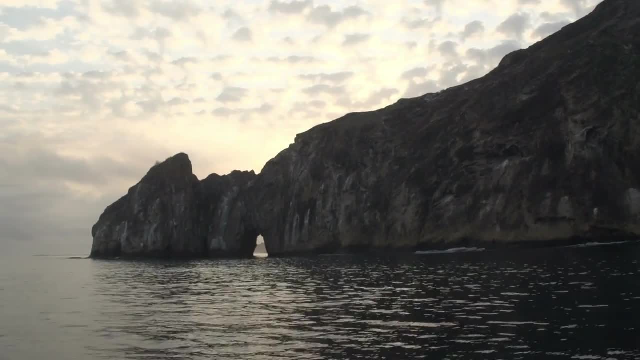 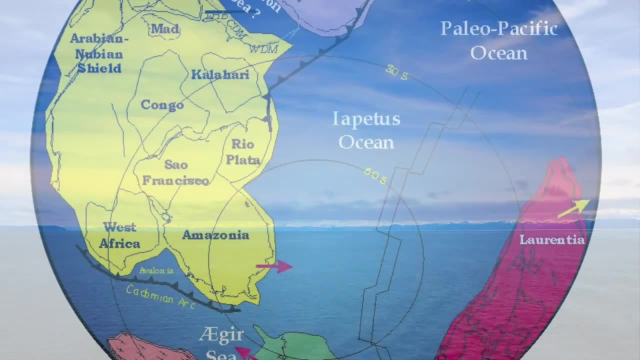 But the union was not to last. Even as the final sutures were healed around the edges, Pannotia began to rift apart from the middle. as a new ocean basin, the Iapetus appeared and began to widen. The very existence of Pannotia is far from certain. 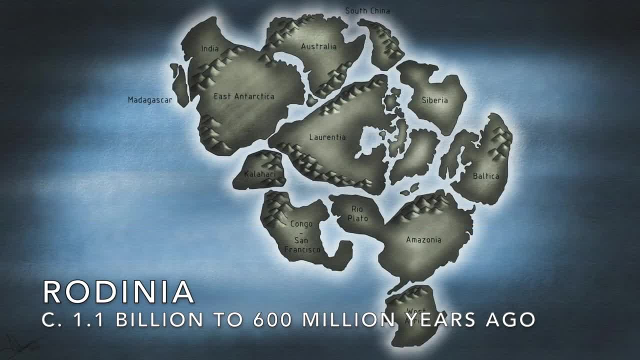 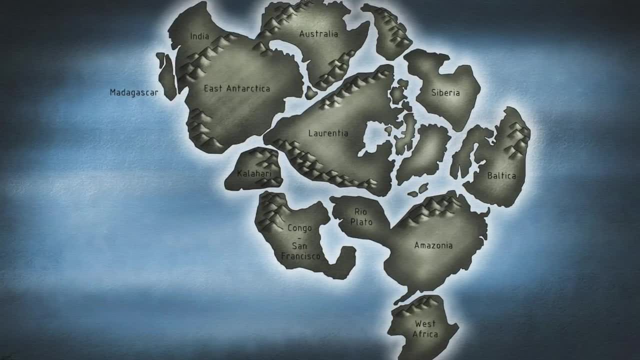 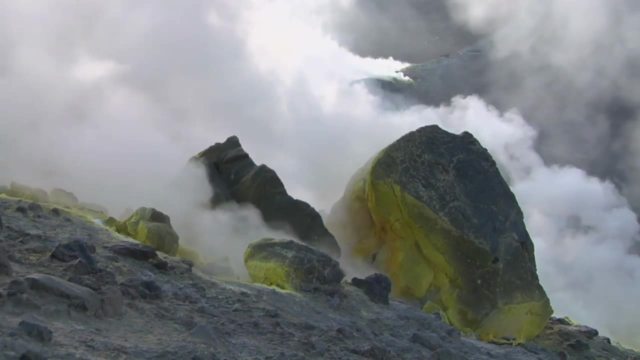 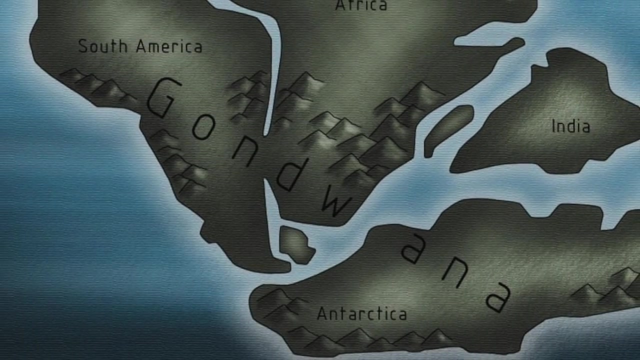 As the messy breakup of Rodinia is difficult to reconstruct across the pre-Cambrian-Cambrian boundary, But the next, or possibly concurrent, continental amalgamation is much better constrained. Gondwana may only be considered a supercontinent under one of the term's looser definitions, as several ancient cratons were excluded from its embrace. 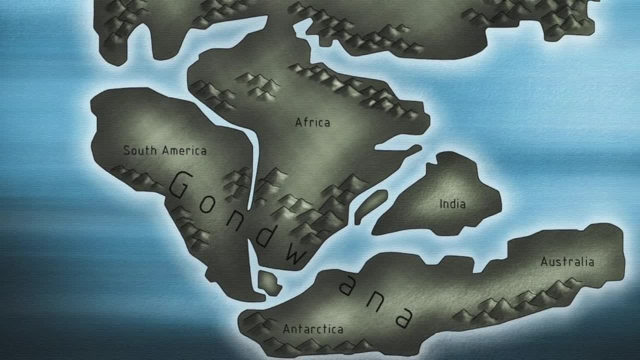 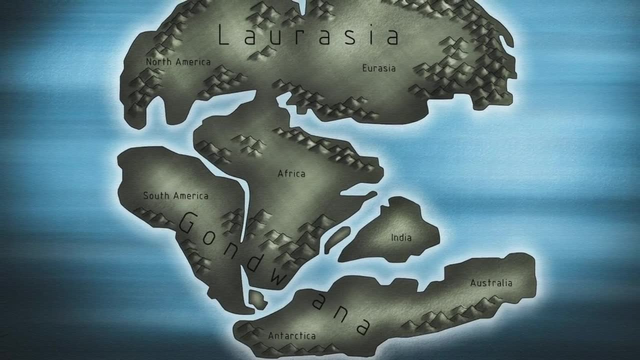 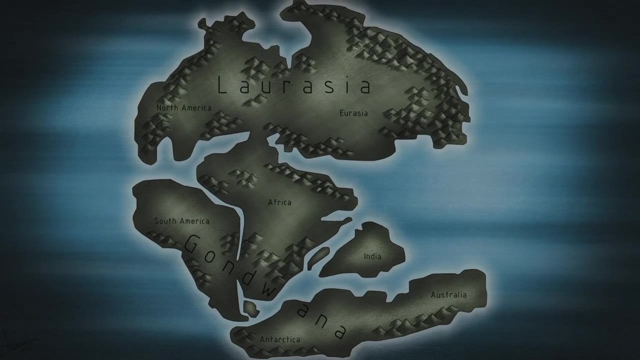 And yet this landmass, which began its assembly with the chaotic destruction of Rodinia and was only completed at the very end of the Protozoic, did represent the largest single piece of continental crust throughout the Paleozoic, Covering an area of around 100 million square kilometers. it saw two-thirds of today's continental area united. 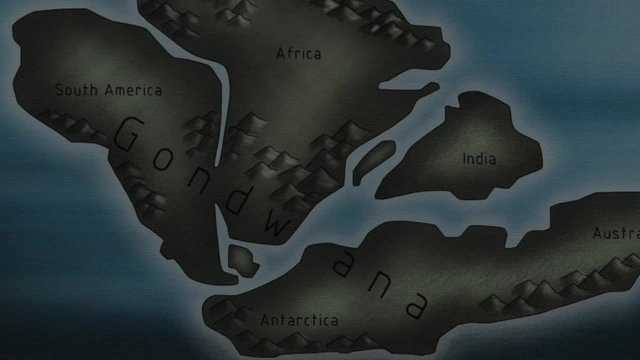 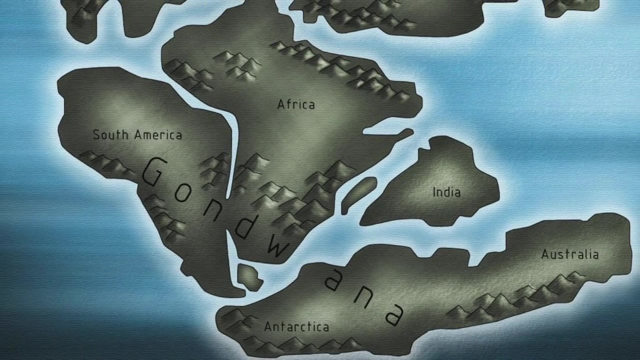 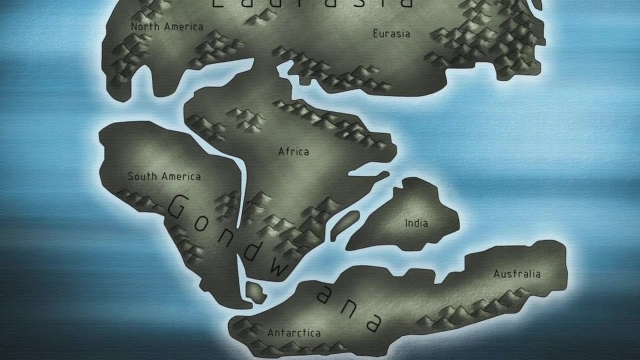 including cratons from modern-day India, Africa, South America, Antarctica, Australia and Arabia. This supercontinent was a melting pot of ancient landmasses and was crisscrossed by orogenic belts, each marking a collision, a lost ocean, a continental fusion. 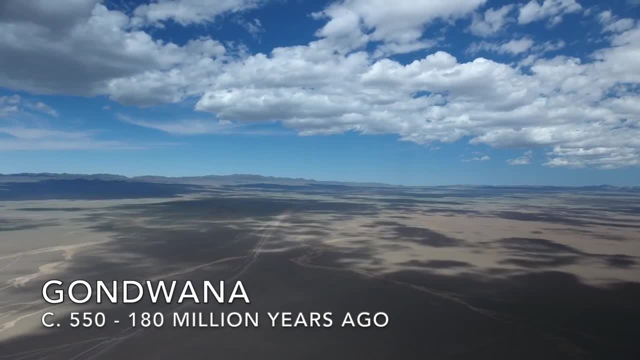 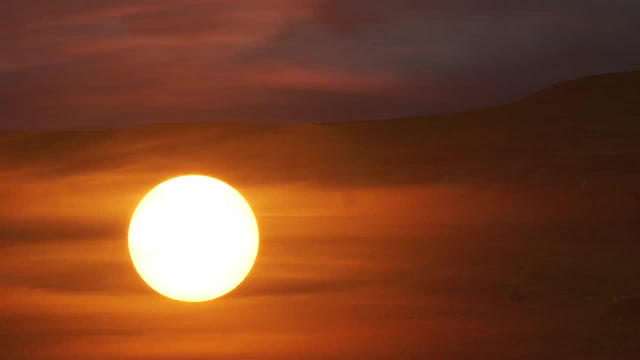 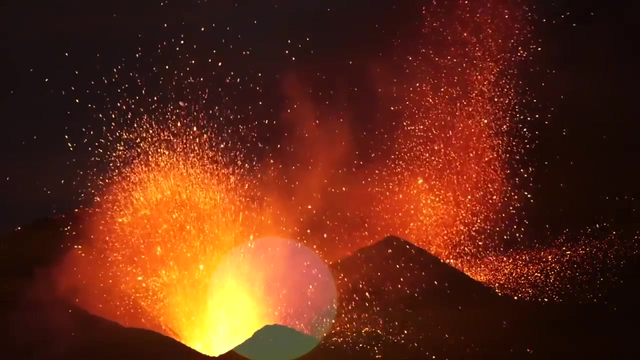 The origin of Gondwana was a brief calm moment after the continental chaos of the late Protozoic. For a few hundred million years there were no more collisions and the supercontinent drifted gently northwards until it eventually met its end 335 million years ago. 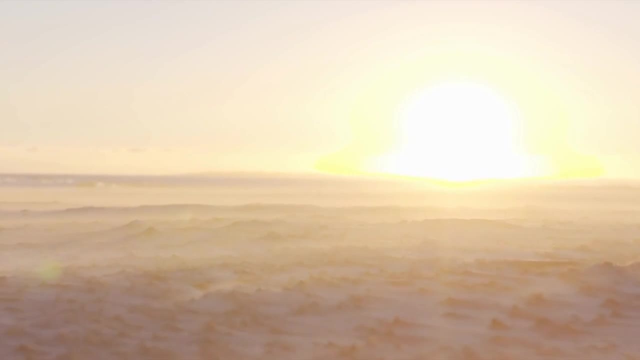 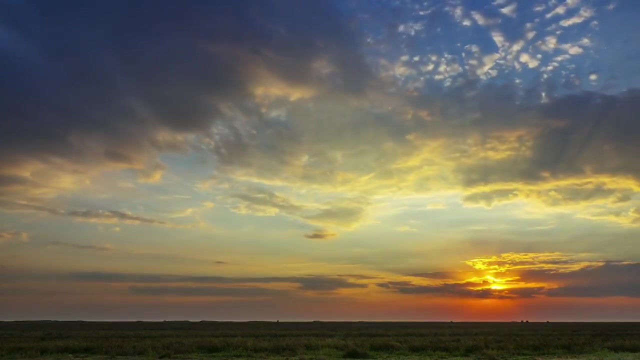 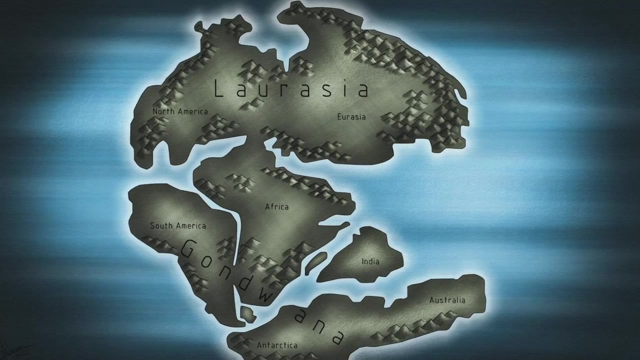 Unlike those that came before it, Gondwana did not die through shattering rifts and diverging fragments. Rather, it lost its supercontinental identity as it collided with the natural world. It now combined Laurentia and Baltica. It was assimilated into a greater whole, a supercontinent in even the strictest sense. 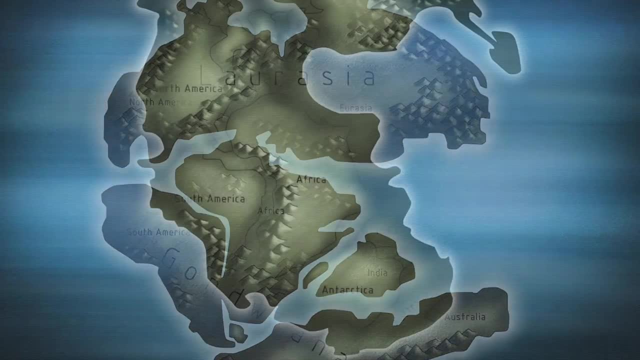 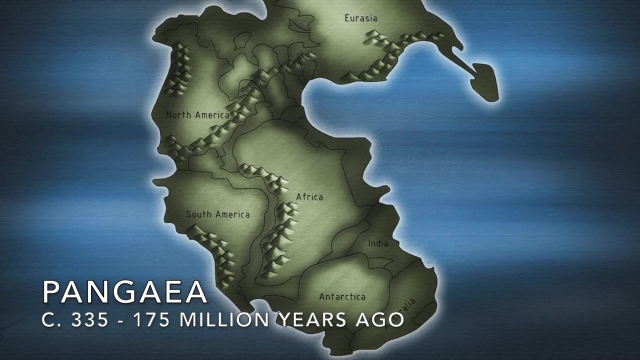 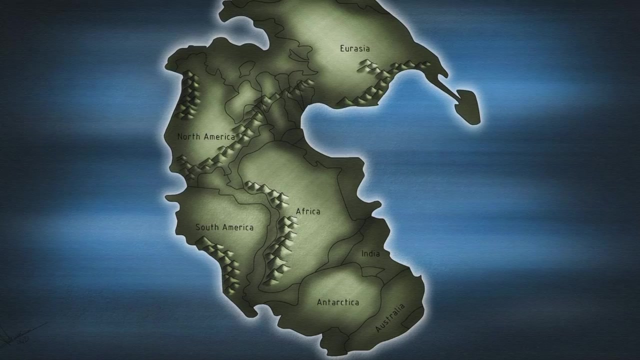 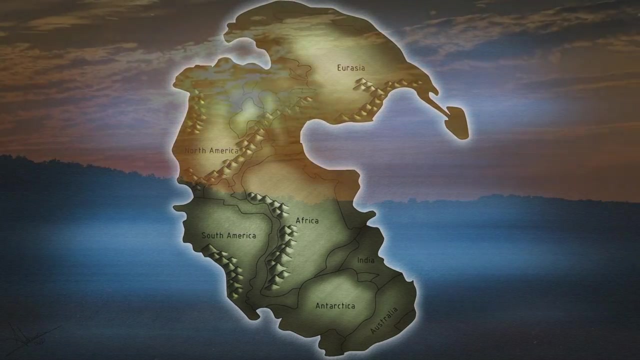 The last supercontinent, Pangea, Where there was nought but disagreement about the configurations of previous supercontinents. there is a wealth of supporting and corroborating evidence. There are plenty of rocks from its Mesozoic tenure, including fossils that can be mapped across once and future fragments. 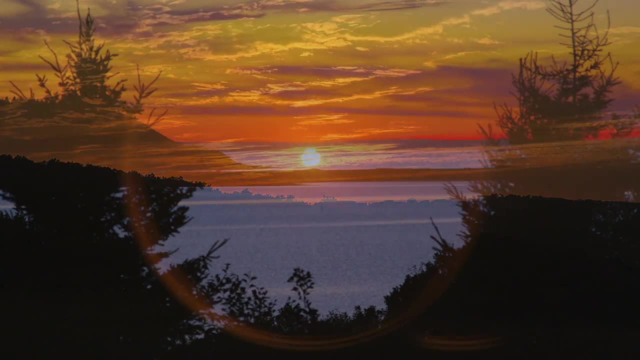 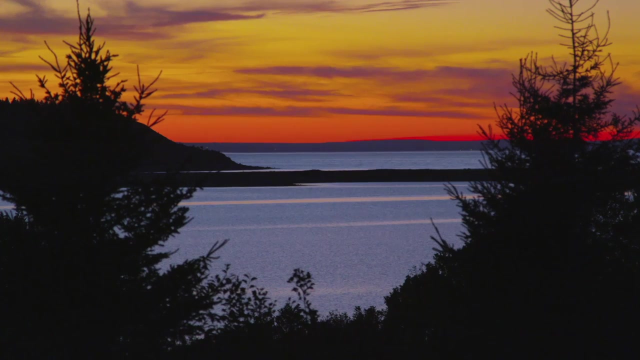 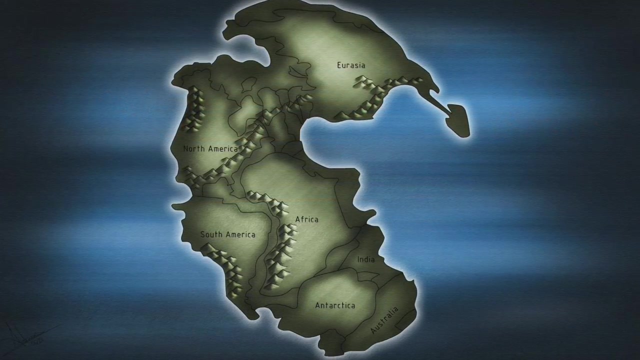 consistent magnetic anomalies and unaltered orogenic belts. Pangea, with its Gondwanan southern regions, reigned until 180 million years ago. The break-up of this vast and resplendent supercontinent saw the opening of the Atlantic Ocean. 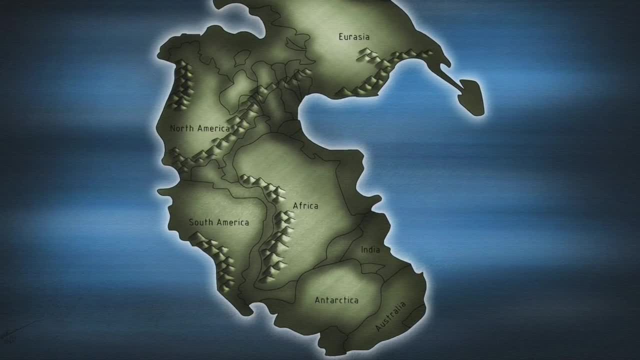 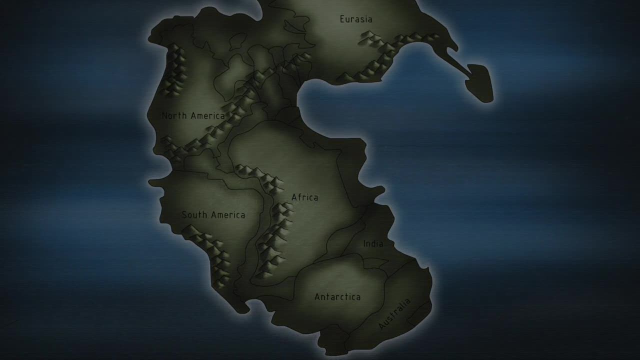 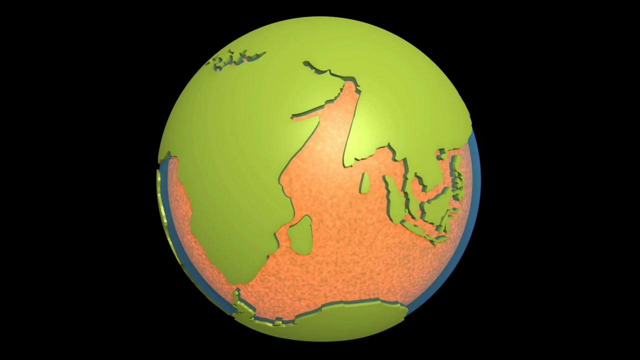 the migration of India towards the Asian subcontinent and the utter isolation of Australia and Antarctica. And so we find our modern world formed from the scattered fragments of Pangea, but also of Gondwana, Panosia, Rodinia, Columbia. 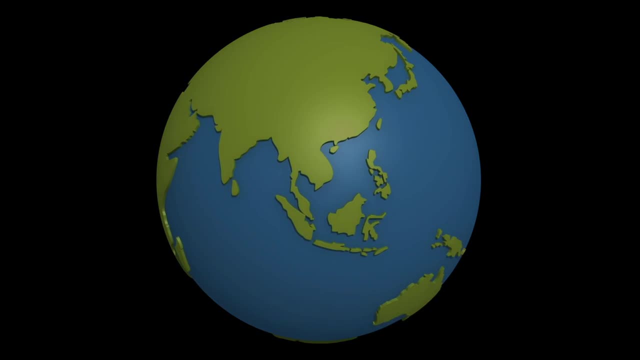 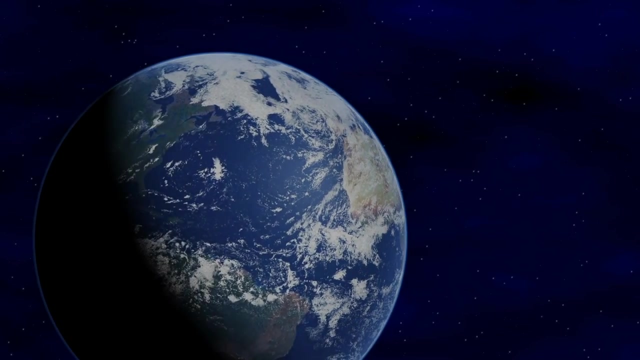 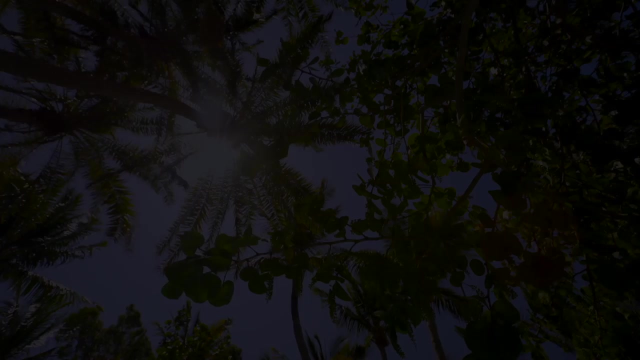 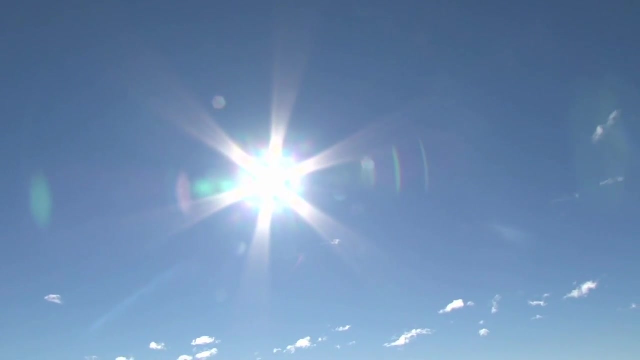 and maybe even Kenorland and Ur. Each supercontinental age was distinct in configuration, duration, climate and character. Pangea was covered in great forests, while Rodinia was barely greened at the edges. Panosia was a frozen wasteland, while Columbia baked in endless ice. 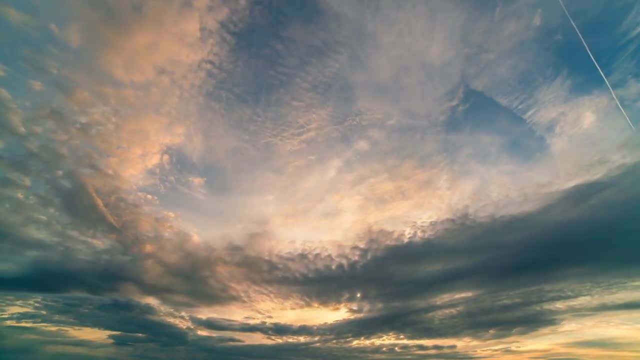 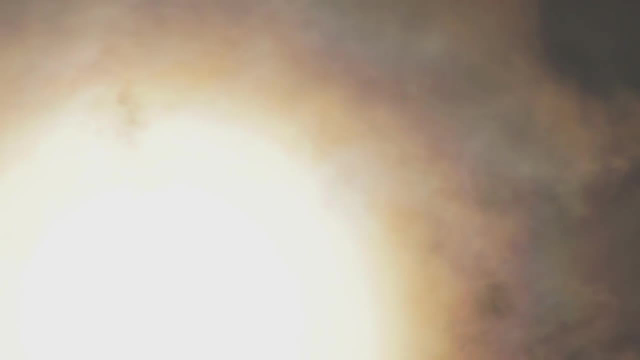 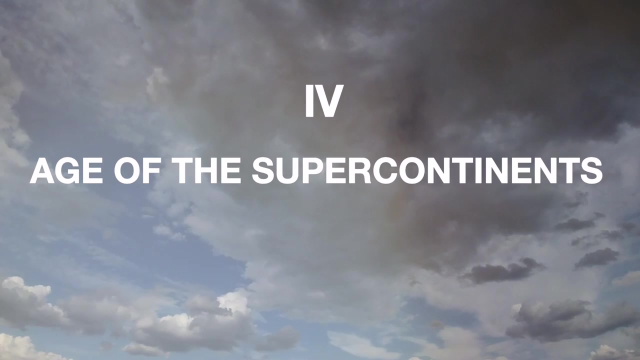 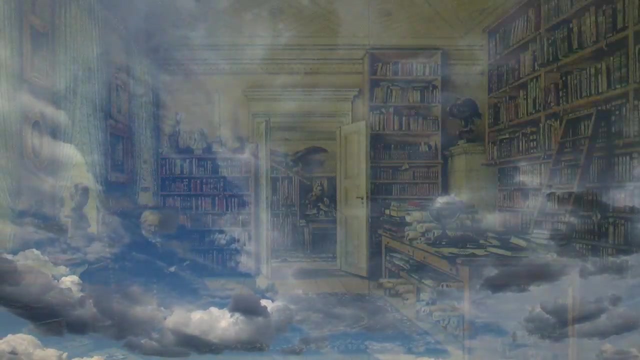 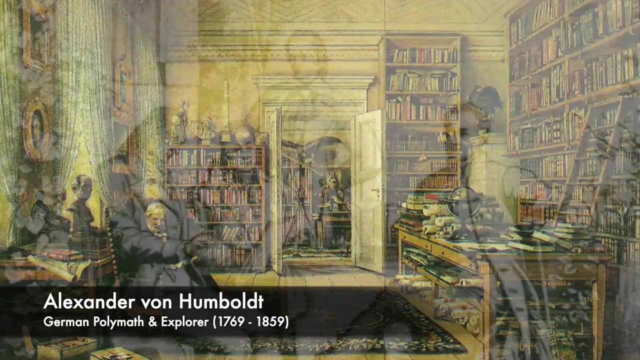 Yet, despite their differences, there are certain conditions that all of these supercontinents shared and which life may face in the coming supercontinental age. Alexander von Humboldt was driven by an insatiable curiosity for the world around him. The German scholar travelled extensively through the Americas and Russia. 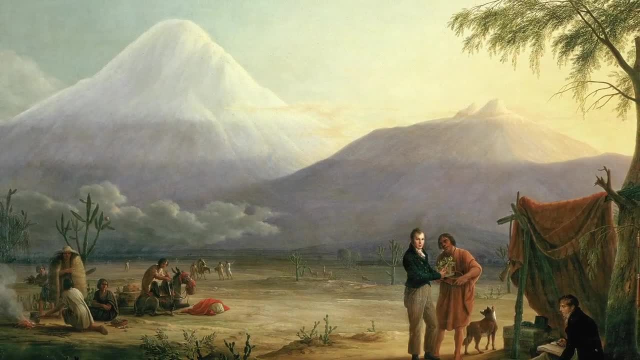 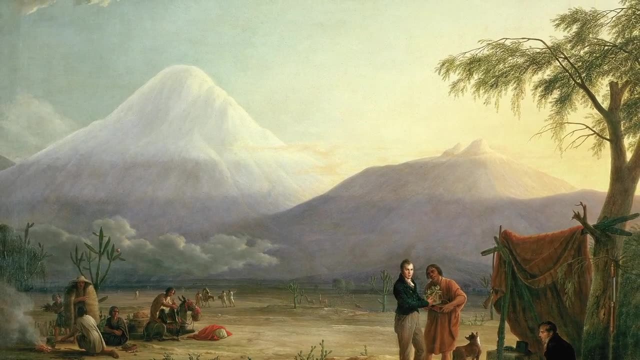 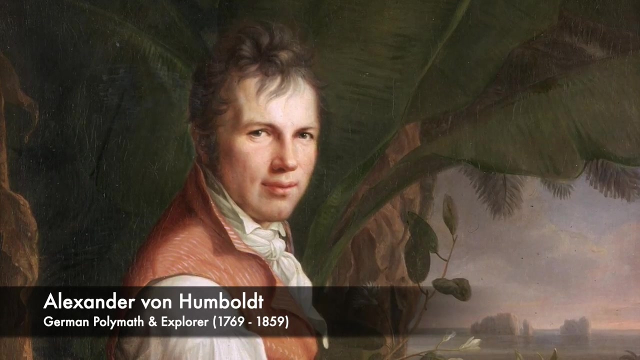 seeking to learn the secrets of those often harsh but exotic lands. Wherever he travelled, he erected weather stations to measure the air temperature, pressure and rainfall, and he collected data whenever he could to build a picture of weather variations over time and space. 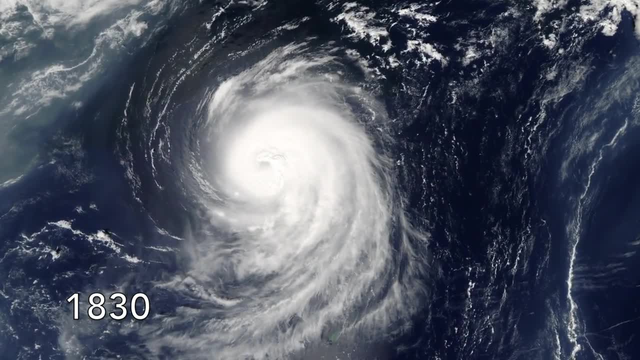 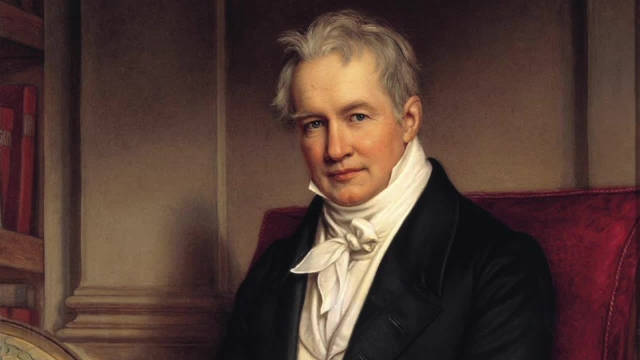 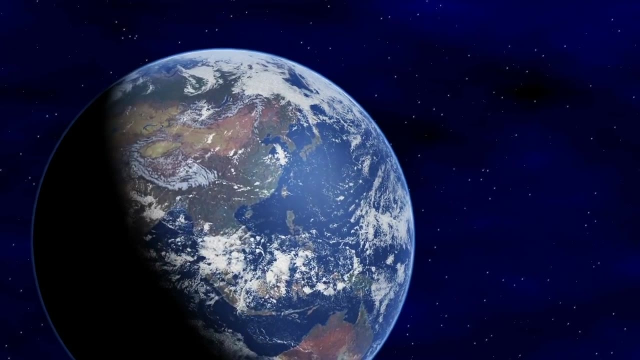 By 1830, he had collected enough data to map out those conditions over a huge swathe of Western Europe and Russia. Von Humboldt was the first to see clearly in his data what any Siberian nomad could have told him. The further inland you travel, the more extreme the weather would become. 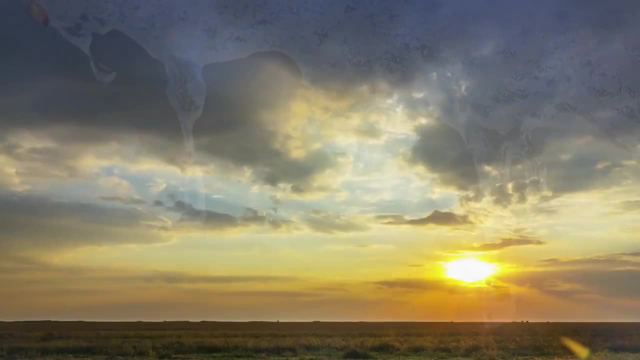 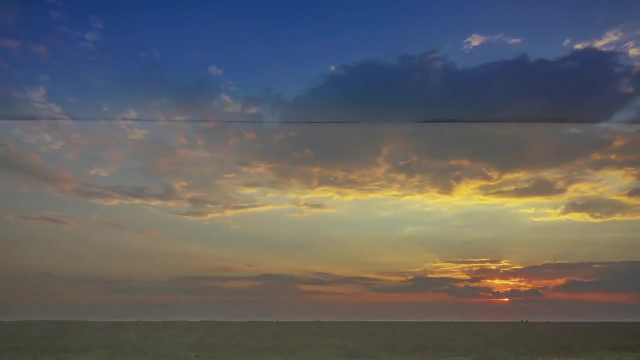 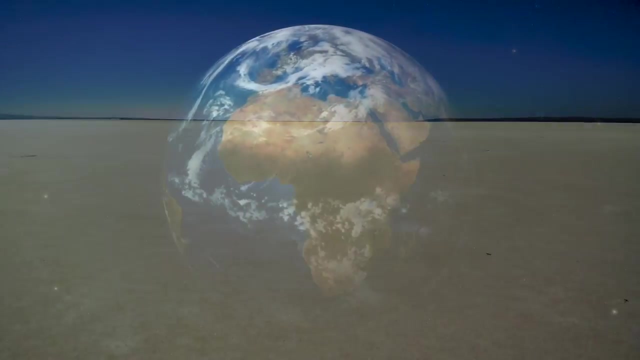 Winters in the interior were colder and summers were hotter than in coastal places at the same latitude. This so-called continentality is a feature of all large landmasses on Earth today and is more pronounced the larger the continent. For instance, Antwerp, close to the North Sea, in northern Belgium. 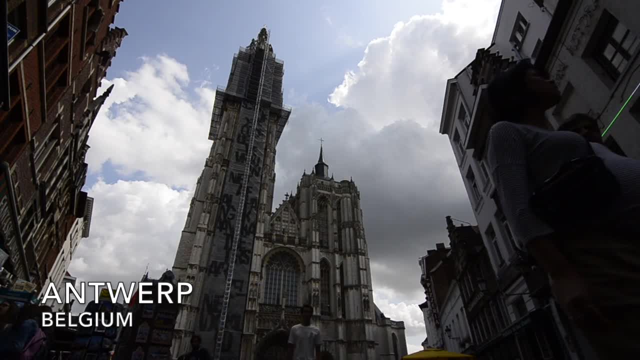 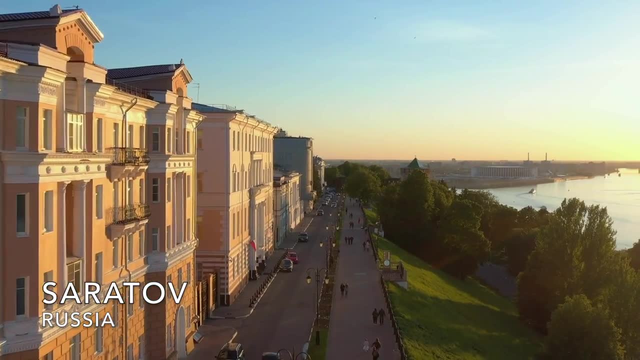 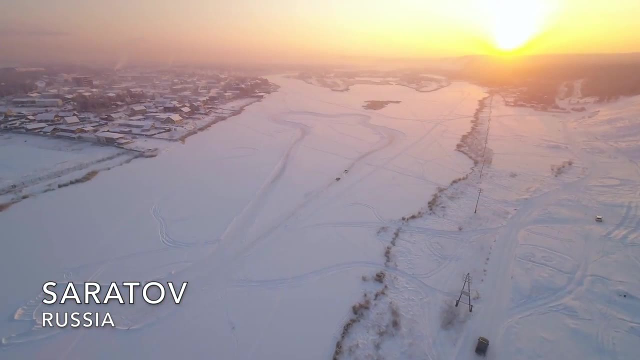 experiences an average summer-to-winter temperature range of nearly 15 degrees Celsius. Meanwhile, Saratov, deep in central Russia, sits at the same latitude but is some 2,000 kilometres from the nearest ocean. Its average temperature range is more than double that of Antwerp. These extreme conditions arise from the differences in how land and sea absorb the heat from the sun. In summer, land areas heat up much more quickly than the ocean, which can distribute its heat at depth, Whereas in winter, the oceans still have some store of heat left over to create milder conditions. 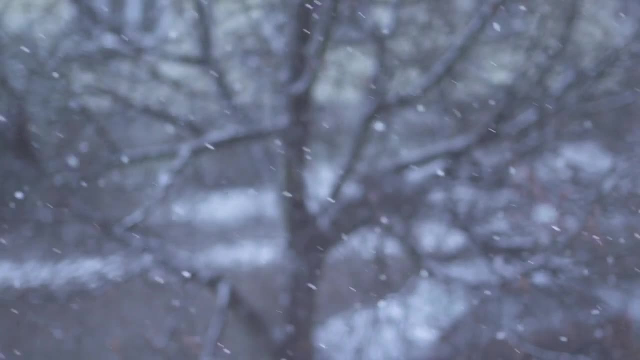 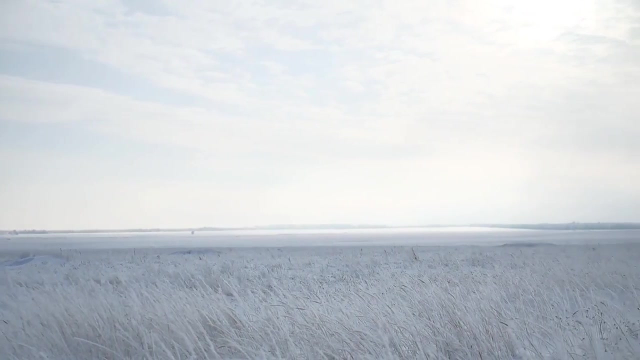 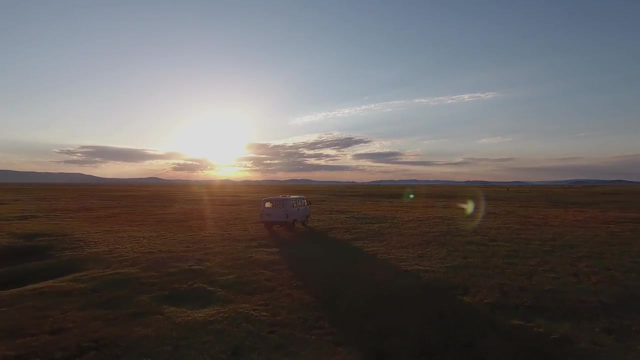 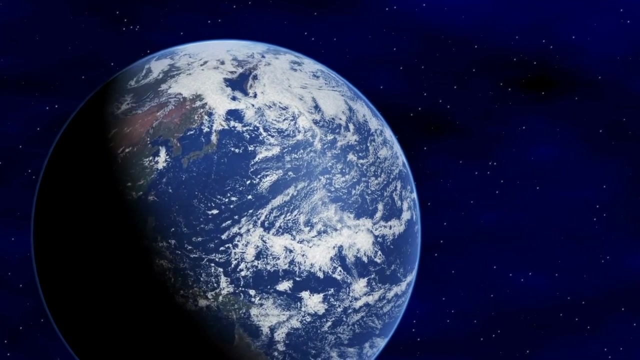 while the land cools much more quickly, Coastal regions reap the benefits of the ocean and the continental interiors are left out in the cold Or the heat. And it is not only temperature that defines continentality. Any satellite image of Earth today will reveal that the deep hearts of continents 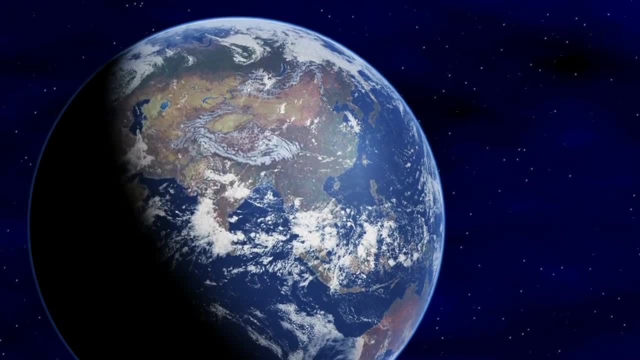 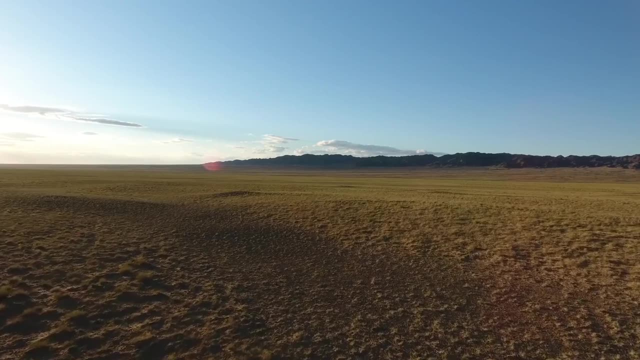 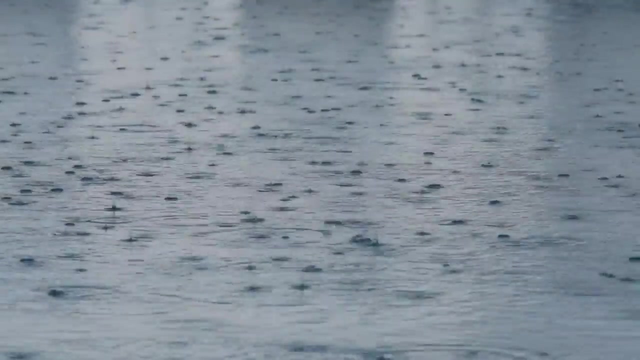 are often deprived of the green of life. They are deserts where little rain falls and living things struggle to survive. One reason for this is the sheer distance. Rain is ultimately derived from warm oceans, and the greater the distance from those oceans, the less rain that is left to fall. 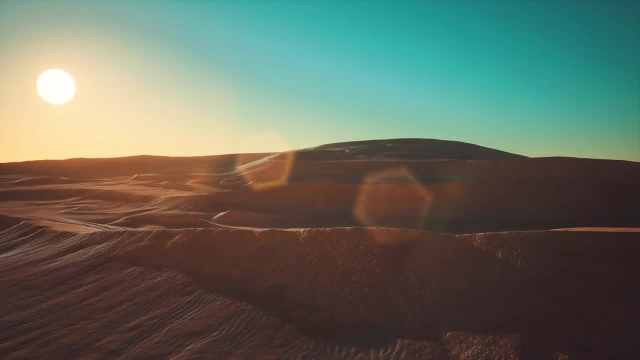 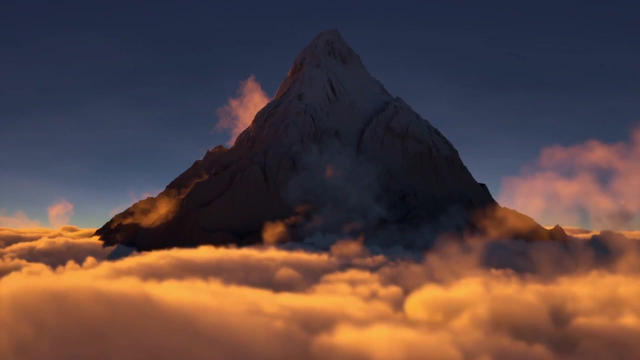 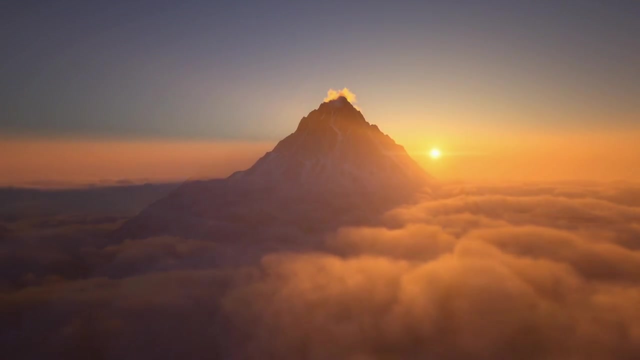 But the clouds and life-giving rain are also blocked by mountain chains. The warm, moist air is forced up steep mountain slopes where it cools, condenses and rains out. The resulting rain shadow mirrors the real shadow of the mountain, but can extend much further inland. 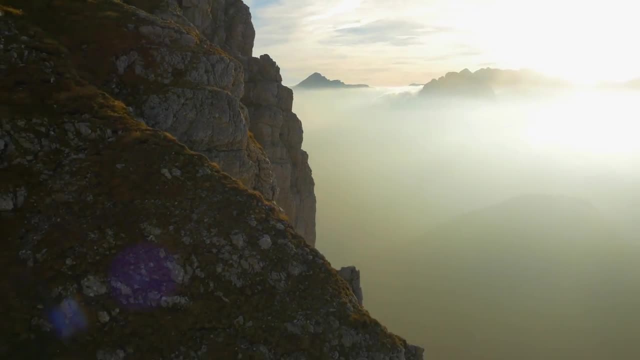 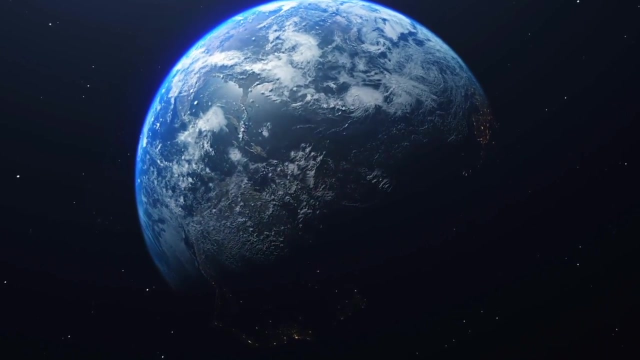 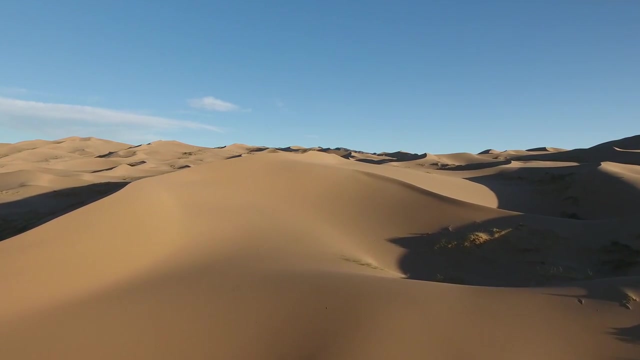 If such extreme conditions are to be found inside the modest continental landmasses on Earth today, then we can only begin to imagine the supercontinentality that held sway in the interiors of Pangea or Rodinia or Ur, Supercontinents positioned at low latitudes close to the equator. 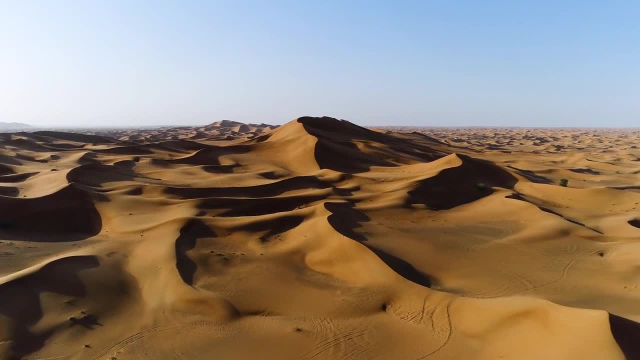 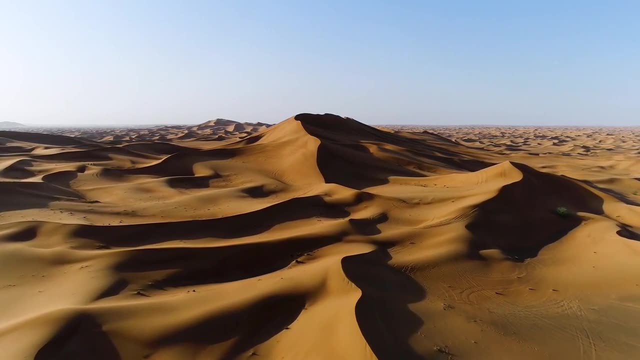 would see their central regions transformed into baits, Dusty deserts where not a drop of rain would fall for centuries or even millennia. Even for the likes of Pannotia straddling the South Pole, icecaps would be slow to grow. 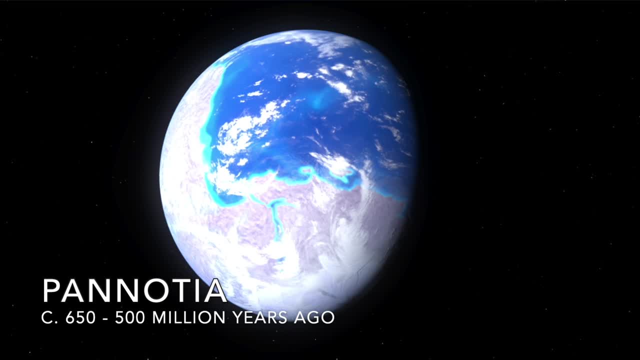 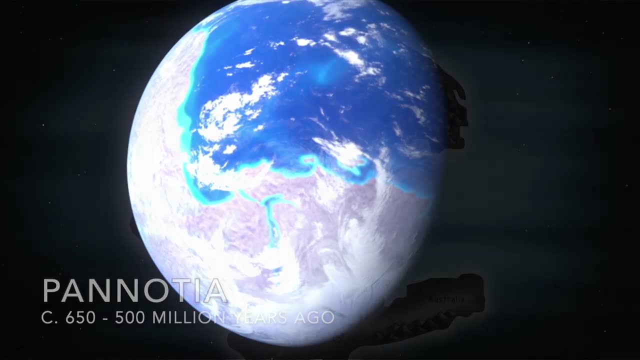 if the snow that fed them never arrived. The suturing of crustal fragments during the assembly of supercontinents or snow-capped icecaps would be the first to be found on Earth. Supercontinents during the assembly of supercontinents also generated mountains. 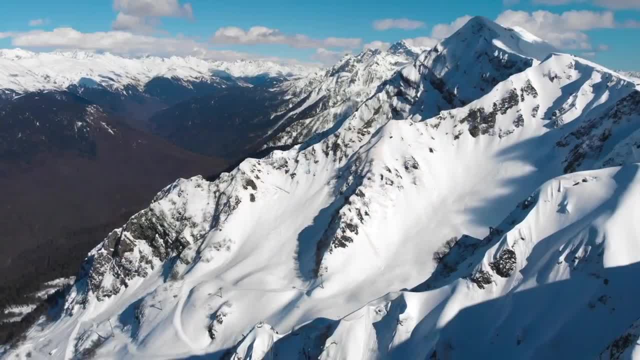 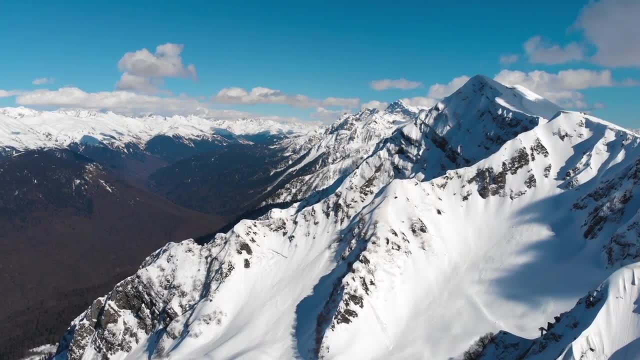 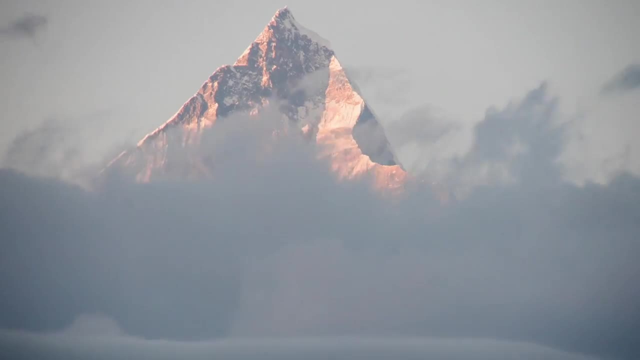 in staggering abundance. With every continental collision, huge ranges and plateaus to rival the Himalayas and Tibet are heaved out of the tortured ground. Monumental towering belts stop weather in its tracks, creating rain shadows that bring the desert ever closer to the coasts. 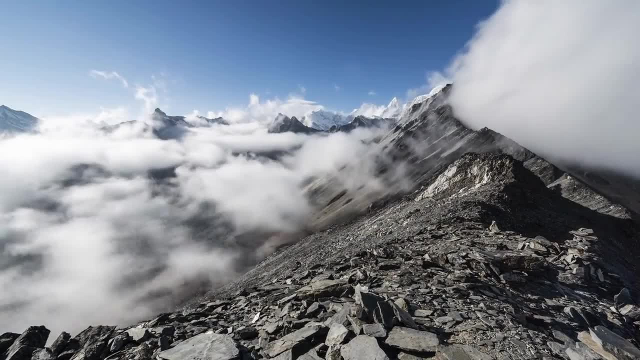 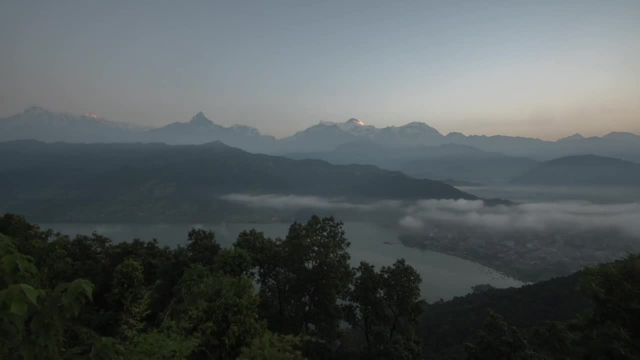 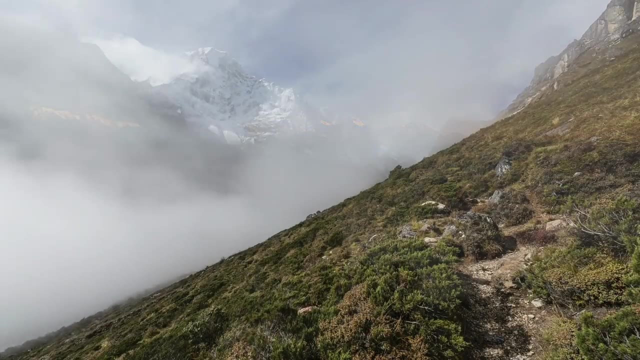 With vast mountain ranges, creating a high-altitude labyrinth of blockages and diversions, wind and weather is whipped into a frenzy. High-level plateaus pump warmth and moisture into the upper atmosphere, driving monsoons that sweep their devastation across the coastal landscapes. 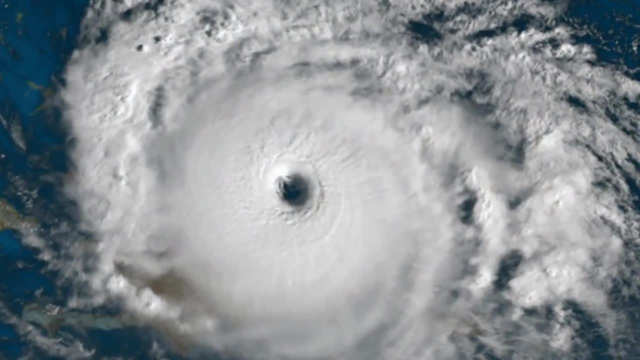 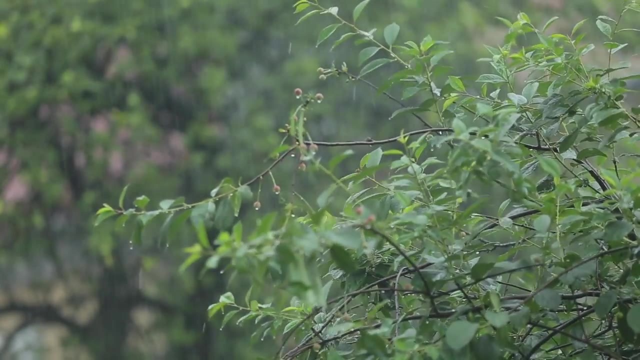 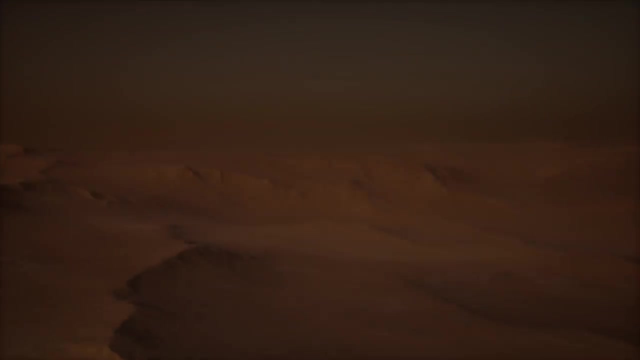 with terrible regularity. Flash floods and ephemeral rivers from these violent storms create huge inland deltas that irrigate the arid lowlands for a time, But these same winds, now stripped of their moisture, howl across the featureless deserts. 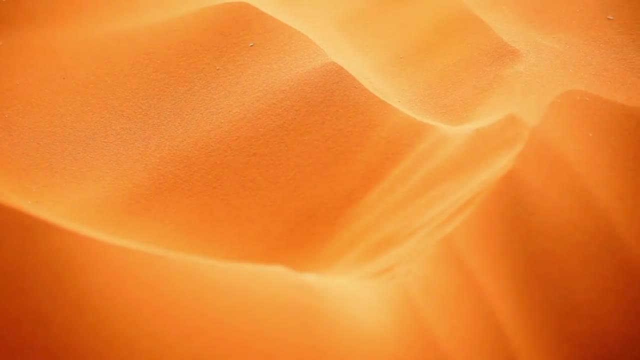 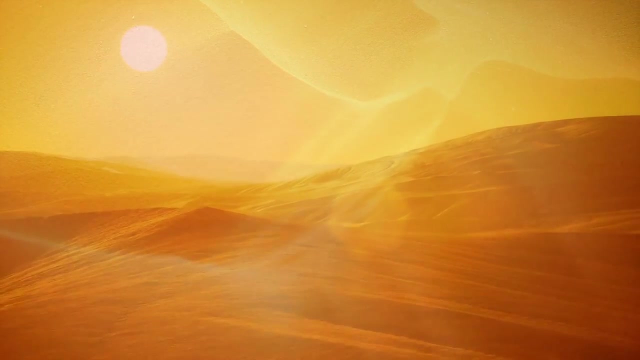 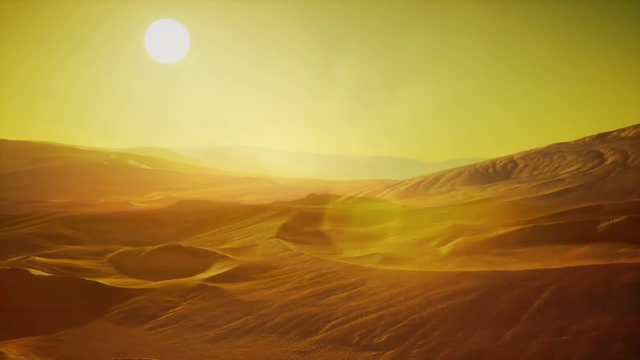 sending dust storms tumbling viciously for thousands of kilometres. Such harsh conditions in the centres of most of Earth's supercontinents would have been little concern for life, Since living things only began to colonise the land surfaces of Gondwana and Pangaea. 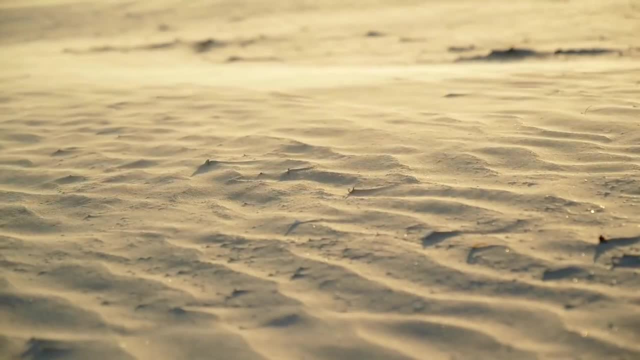 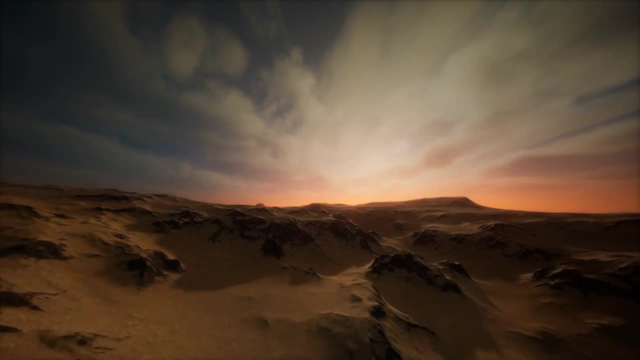 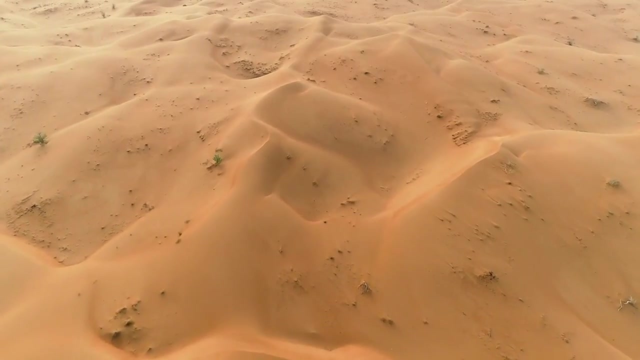 But for those pioneering forests, insects and teetering tetrapods, supercontinental life was unforgiving. Many places were all but uninhabitable: The dry interior deserts, the wild, wind-whipped mountaintops, But towards the coasts. 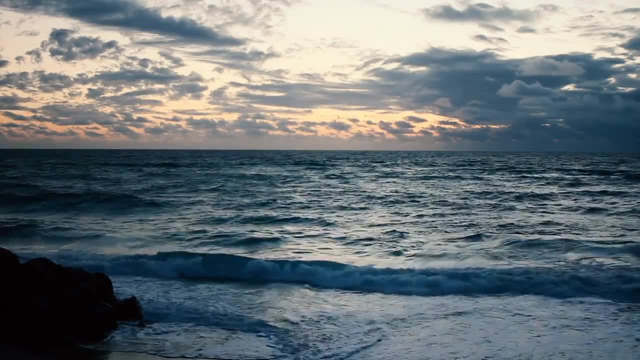 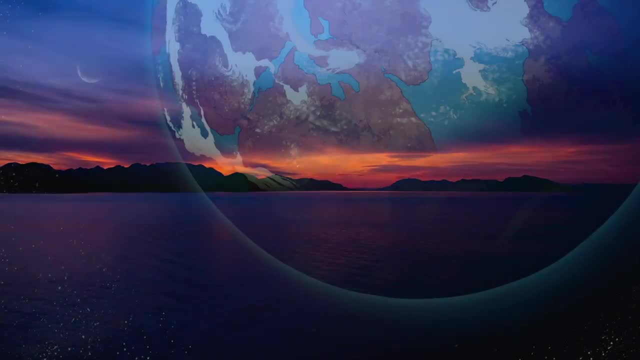 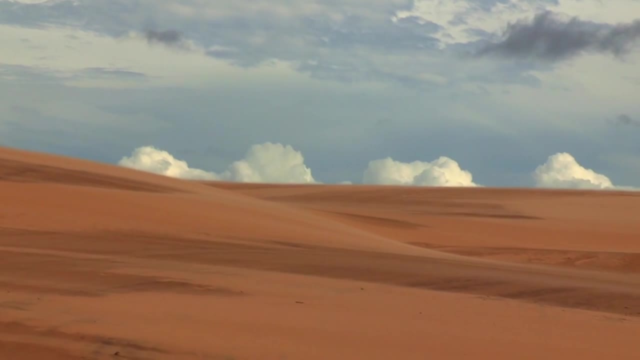 and along sustaining rivers and deltas. the supercontinents offered a bounty of newly exposed mineral nutrients and all living things thrived. Populations on land boomed and crashed with the march of the seasons, compared to the constancy of life beneath the waves. 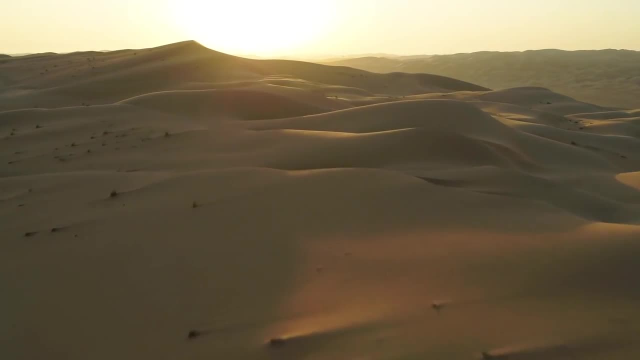 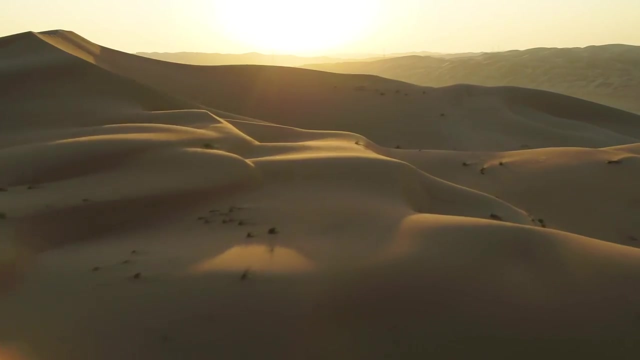 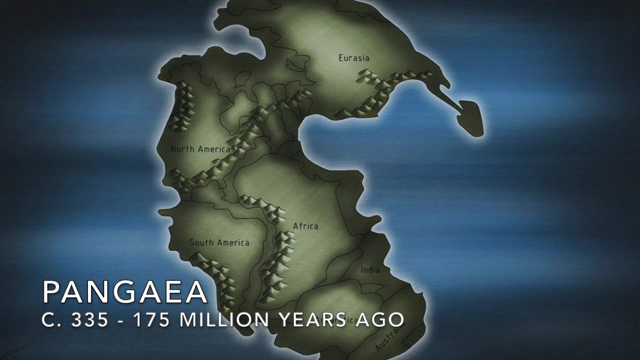 But there was plenty of time to adapt. The dance of the continents may seem frantic when we fast-forward through Earth's history, but the reign of Pangaea spanned the entire ancestry of the dinosaurs, from the first slithering steps onto land in the Devonian. 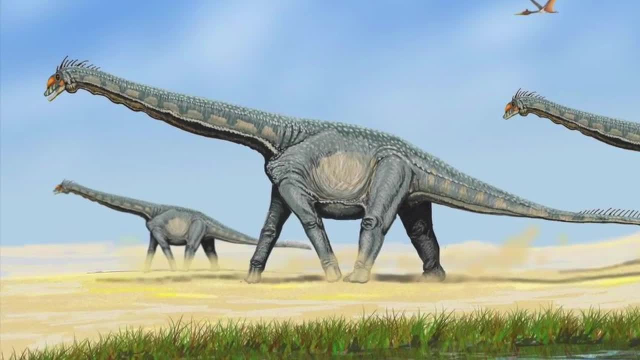 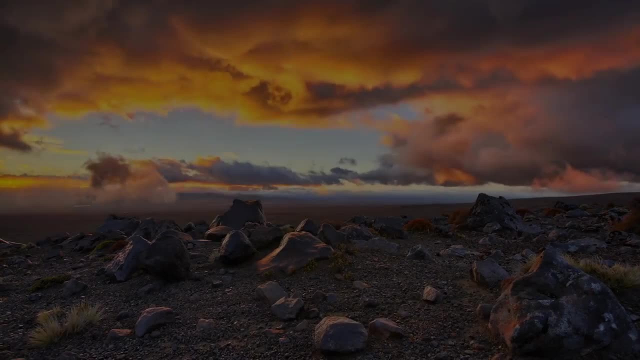 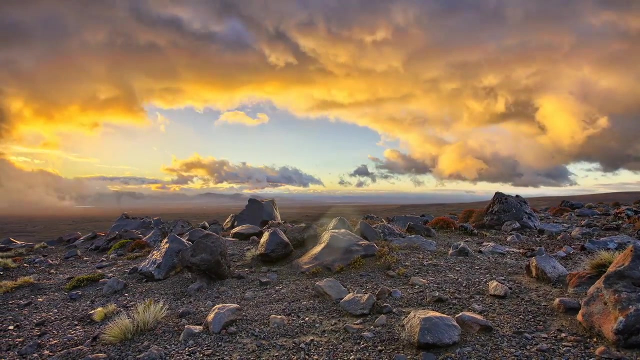 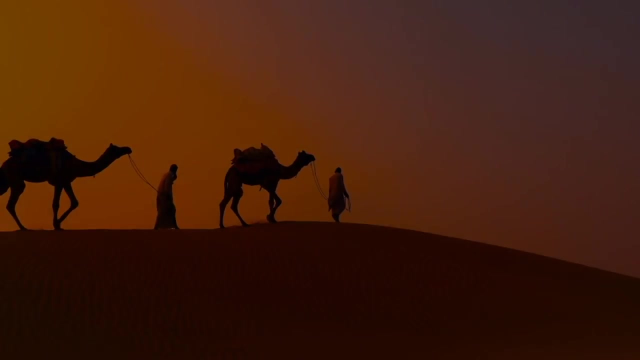 to the mighty, long-necked lizards of the Jurassic. We cannot truly know what it is to live on a supercontinent, since that is not something humans have ever experienced, even in genetic memory, And unless humankind persists for another 250 million years or so. 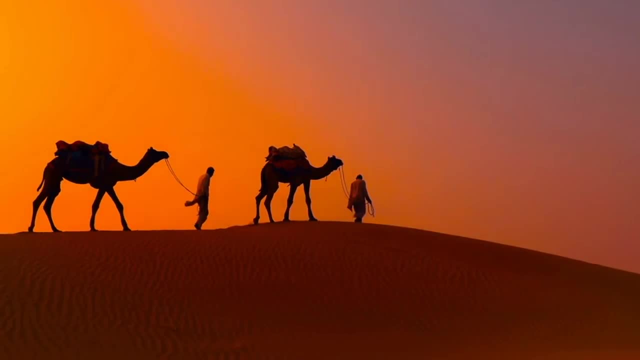 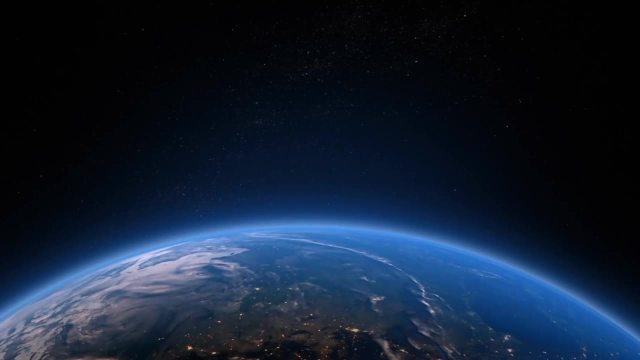 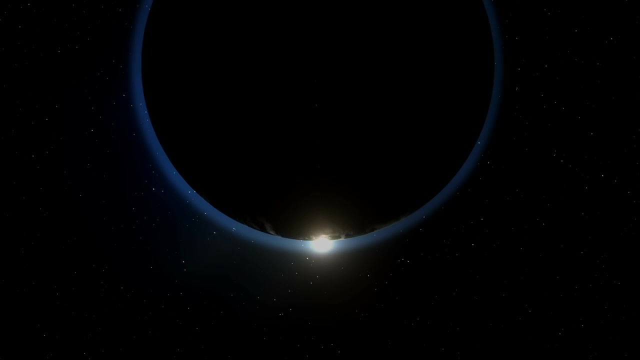 we may never know. We are living through a time of continental dispersion, But another supercontinental age is on the horizon. Even now the assembly is beginning. The current movements of the plates will bring continents together. one by one, Africa and Arabia will grind northwards into Europe.